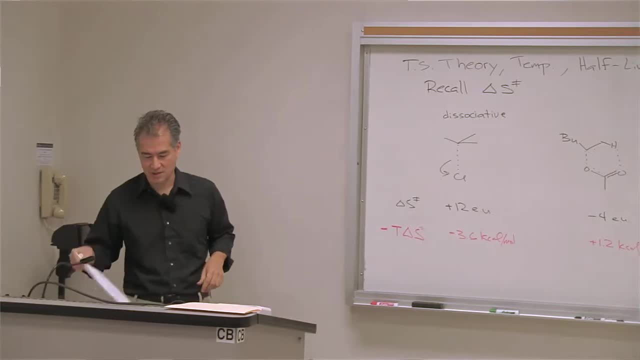 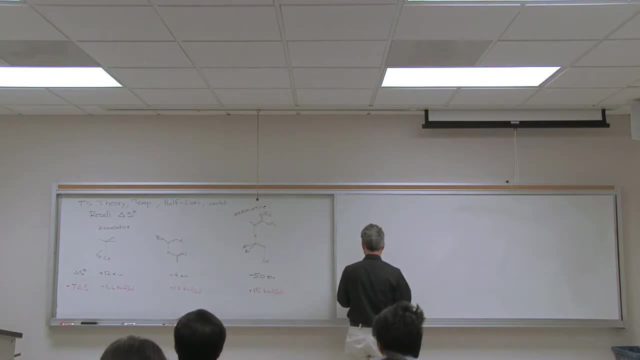 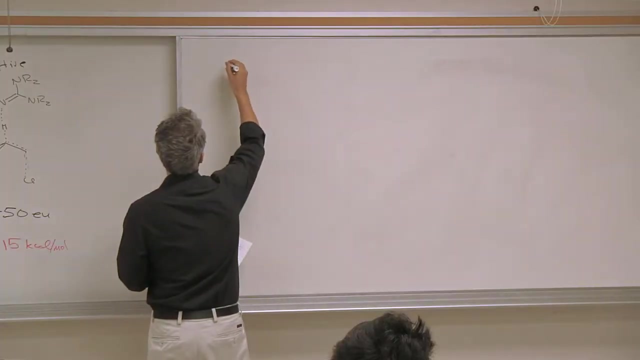 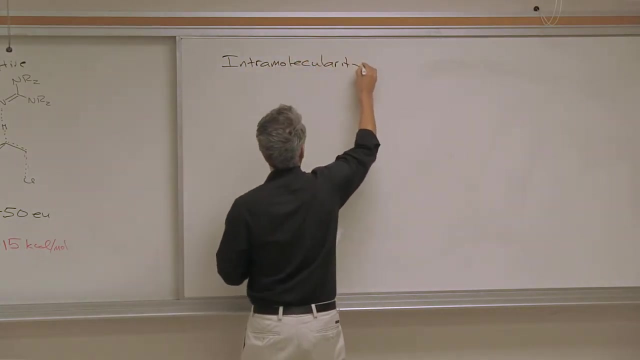 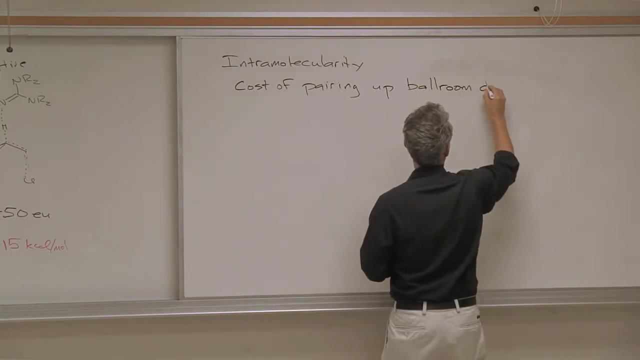 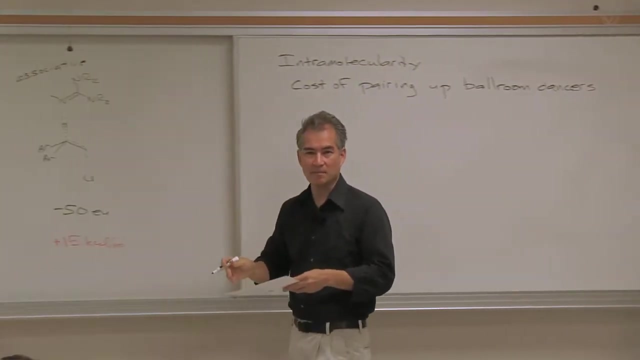 in kcals per mole and in factors of 10, what that's costing you in the transition state. OK, So let's take a look at another example of entropy costs in transition states. OK, I want you to think about the costs of pairing up ballroom dance. That's a highly 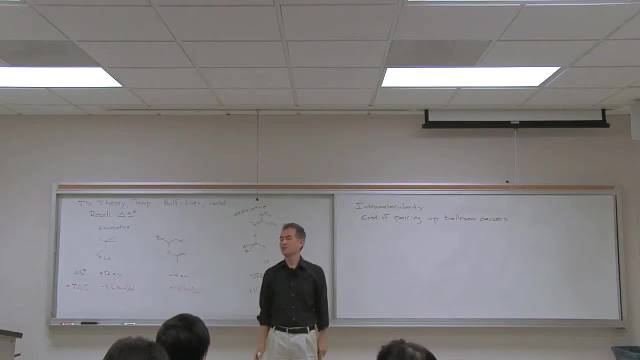 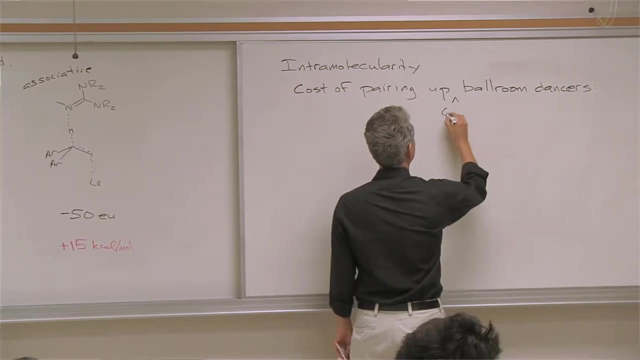 organized process, pairing up ballroom dancers. And now I want you to translate that into 6.02 times 10 to the 23rd ballroom dancers, because that's the way you really need to think. What would it cost to take 6.02 times 10 to the 23rd ballroom dancers and put them? 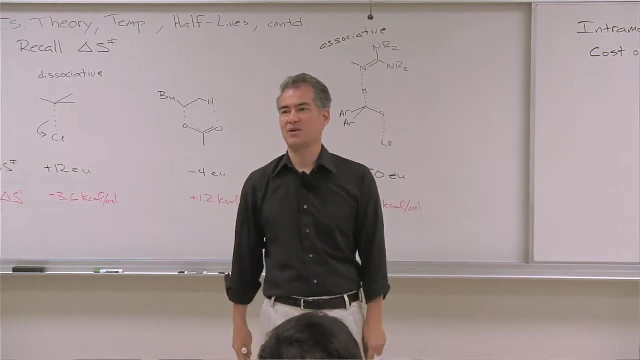 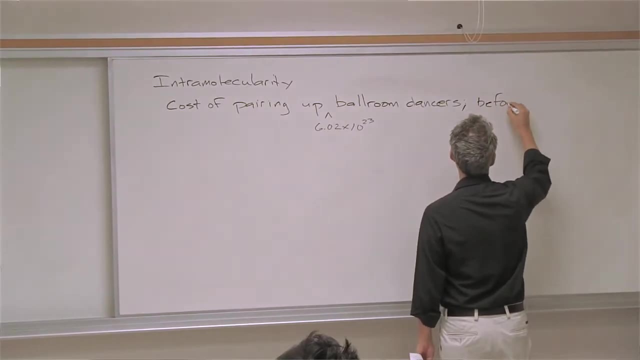 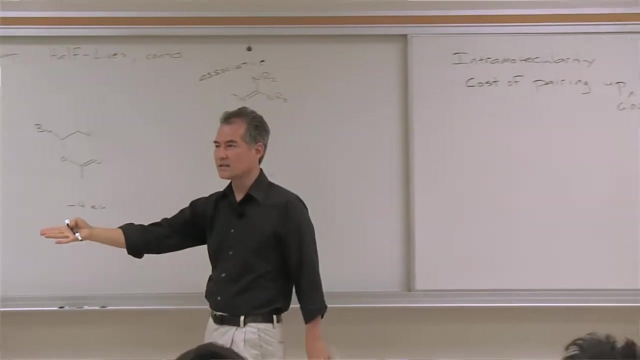 together and get everybody paired up before the music starts. We're not talking about dancing Just before the music starts, getting everybody paired up, And that's the entropic costs of a transition state in something like a Diels-Alder reaction. That's how you're. 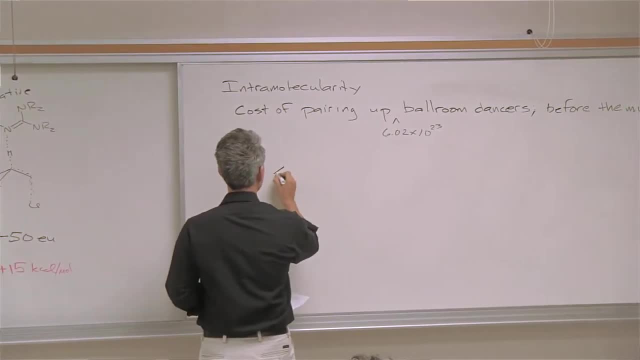 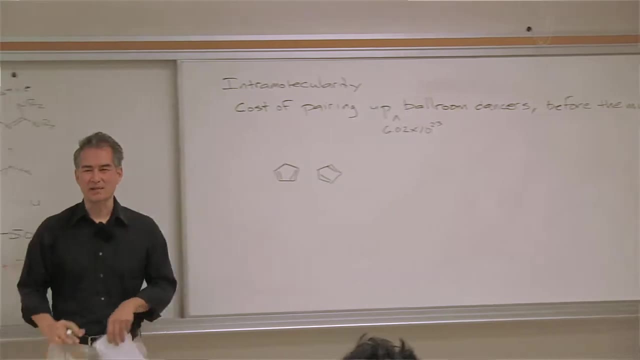 going to imagine how hard it is to get reactions to work. So when you draw out a reaction like this, you totally underestimate this. But the entropic problem here of getting 6.02 times 10 to the 23rd pairs of these 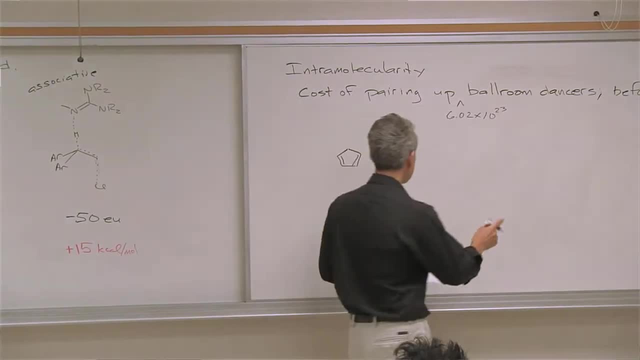 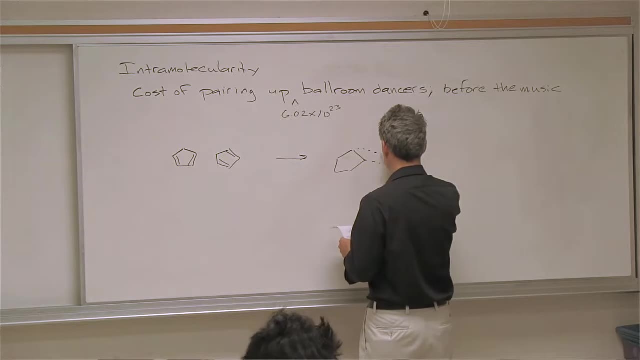 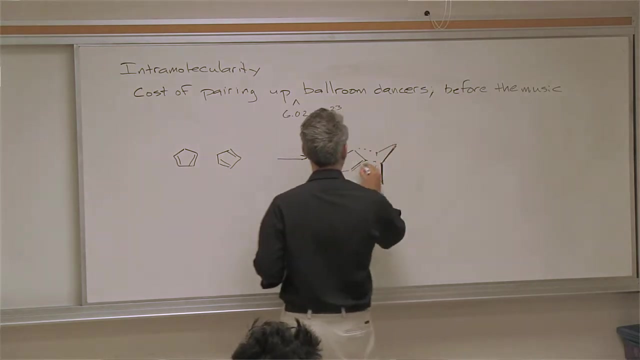 things aligned and ready to start reacting, And so those costs have been calculated. So in the transition state you've got these two molecules getting closer and closer, and closer together. I'm not sure I need to draw out all the bonds here, but you get the idea. 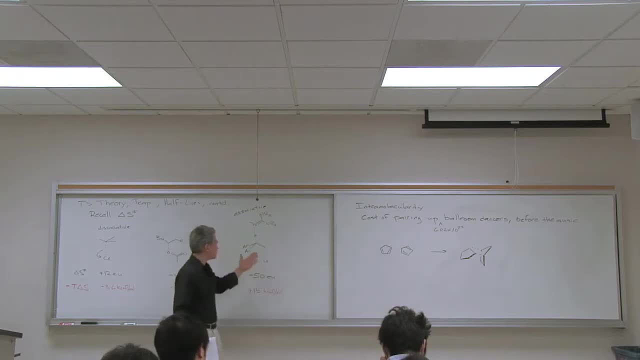 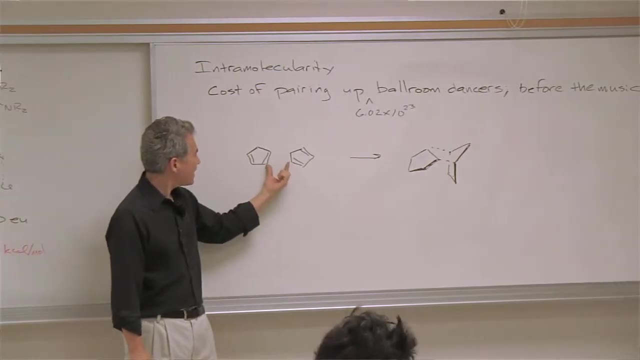 This is like that very entropically costly transition state I had here. that's really picky, Where all the bonds have to be a certain way and the alignment has to be a certain way. Now I've got to have to get two sets of atoms perfectly arranged in order when 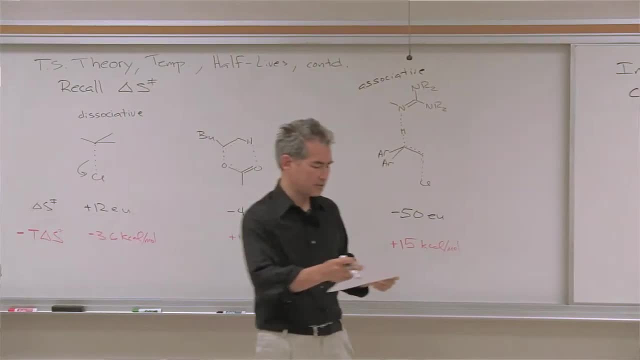 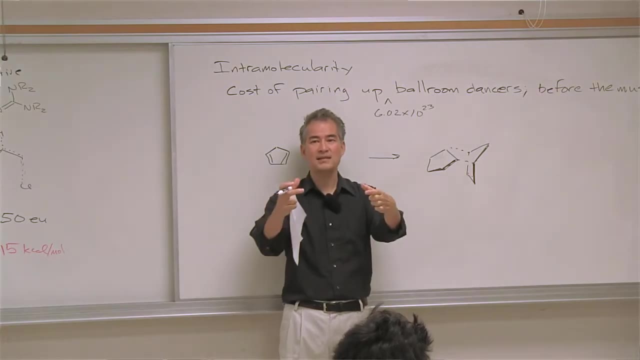 they come close to each other, And so the entropic costs for a Diels-Alder reaction, for a cycloaddition reaction, where we're simultaneously forming two bonds, Two molecules, have to simultaneously collide and get to a transition state where both of these carbon. 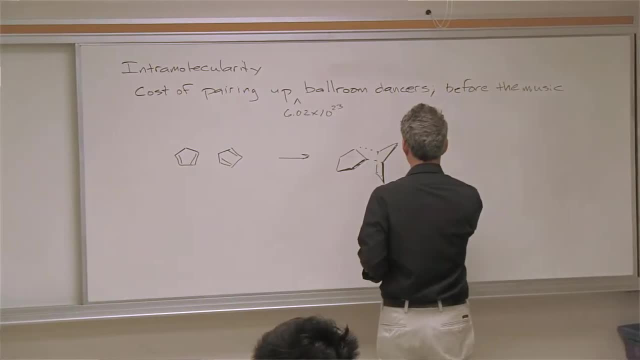 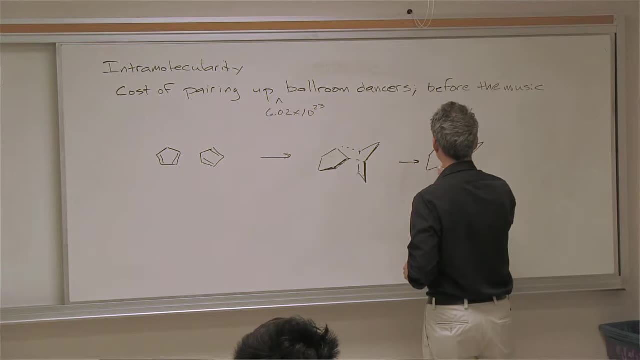 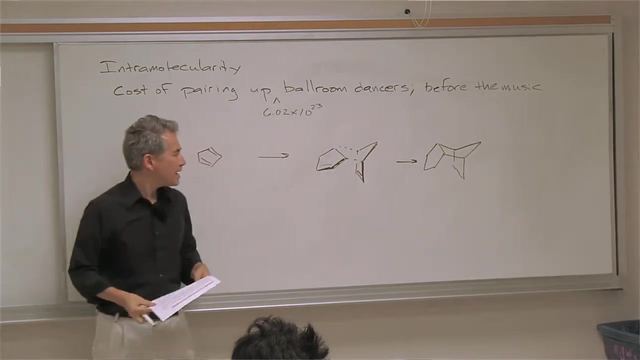 sets of carbon atoms are aligned perfectly, And so the cost of that. it's very similar in structure to the final product for this Diels-Alder reaction. If you look at the transition state for a Diels-Alder reaction like this, it looks very product-like. So if you can estimate the entropy, 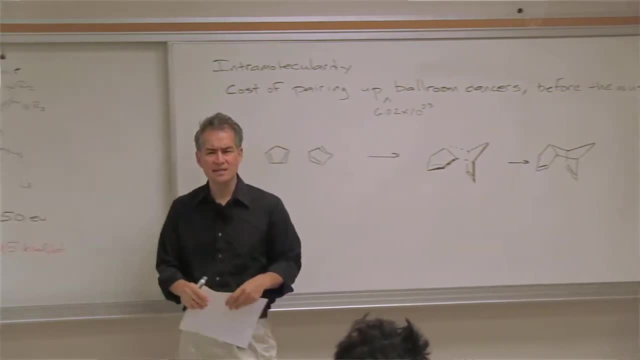 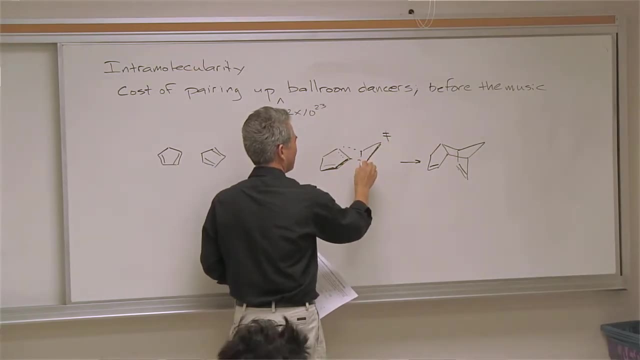 loss in bringing these two molecules together in the product. you kind of get a sense for the cost in that transition state. So here's the transition state with my dashed lines, And I don't want to add all the dashed lines here because it's going to become too complex. 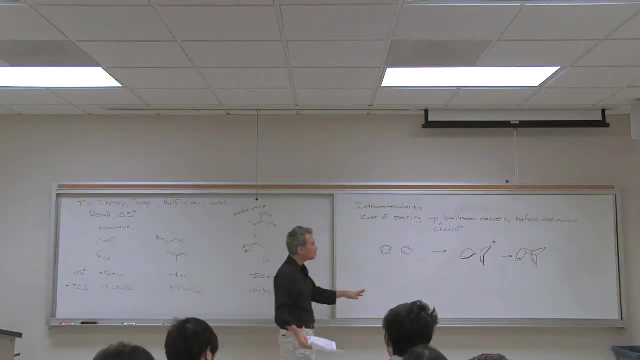 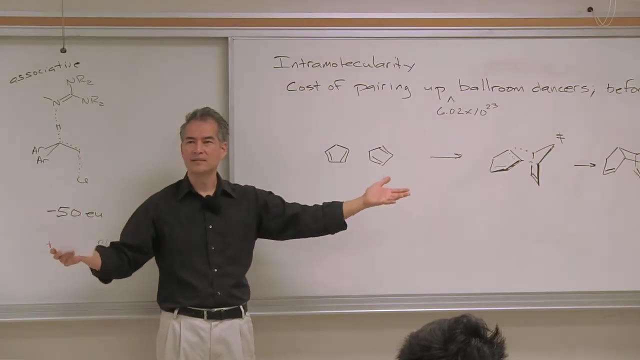 but you get the idea And you think about this- 6.02 times 10 to the 23rd of these transition states and what it costs to go from totally flexible and you can be anywhere you want, like a dance club, to being the ballroom dancer analogy. 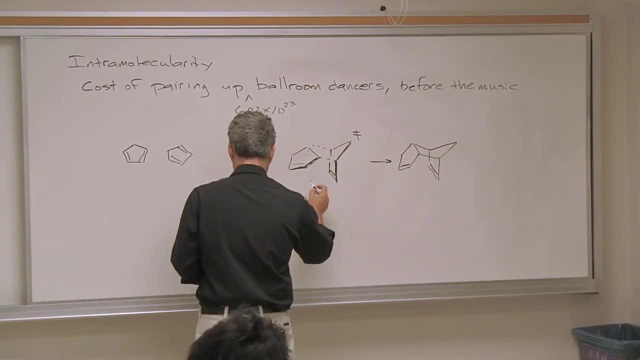 Let's take a look at what's happening in the transition state And I'll give you these numbers here. You can think of it either as product or transition state, because the transition state is so product-like And in this case, the numbers that have been estimated for enthalpy. 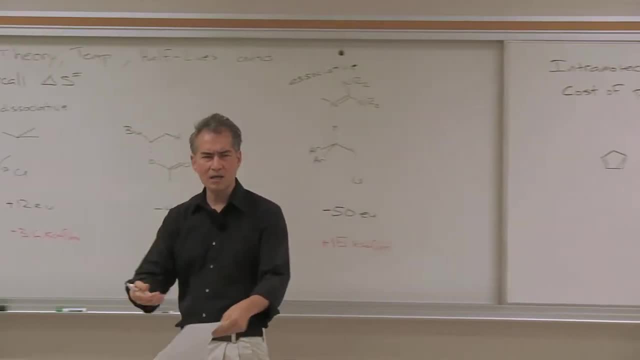 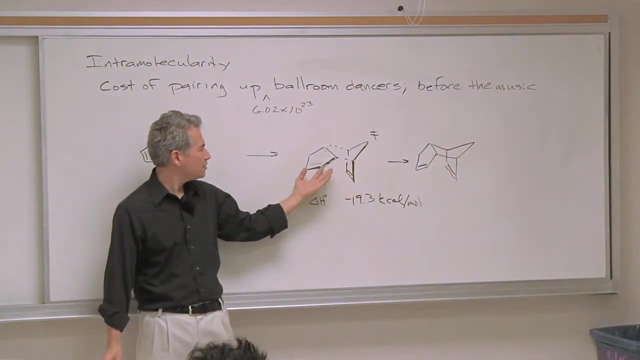 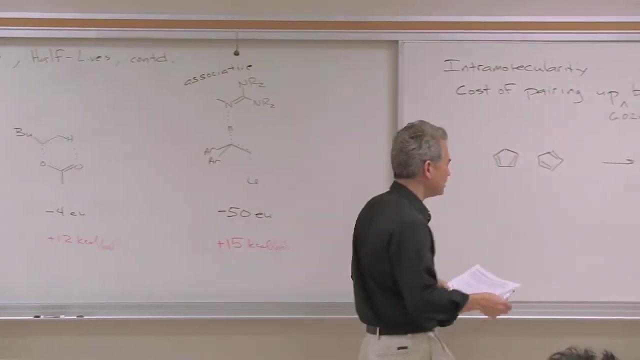 it's favorable. It's favorable to bring two molecules together in a Diels-Alder reaction. when you look at the final product, right, You go from. you trade off two pi bonds in this reaction for two sigma bonds, And we know that that's enthalpically favorable. But let's look at the entropic cost. 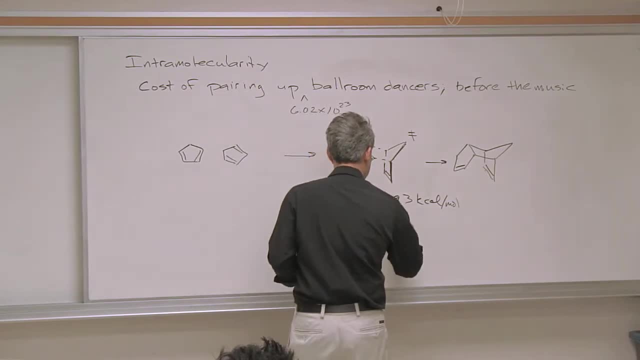 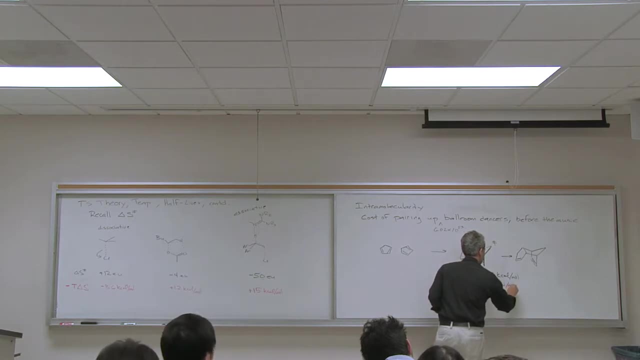 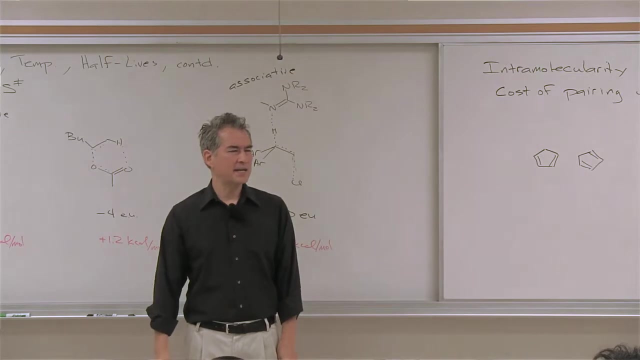 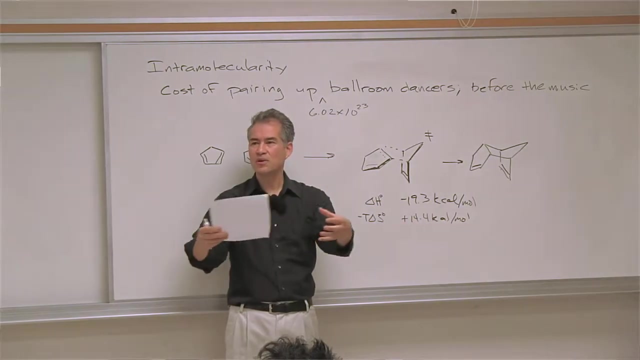 of bringing these molecules together, And this is where we see the expense. So, enthalpically a Diels-Alder reaction is favorable by 19 kcals per mole, but entropically it costs you almost 15 kcals per mole to bring this 6.02 times 10 to the 23rd molecules together. 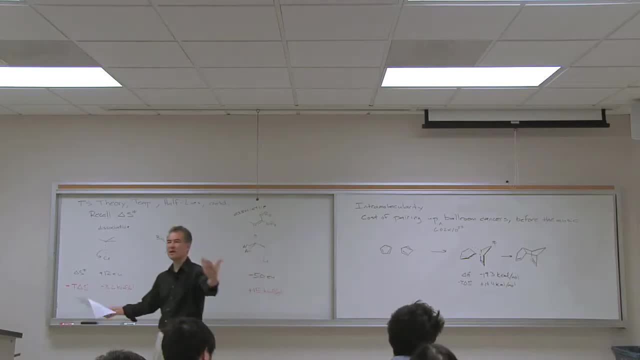 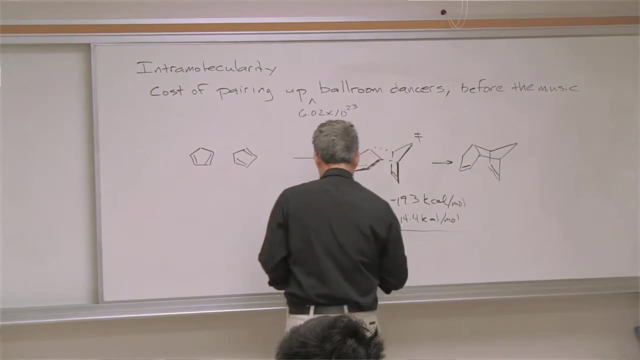 You almost cancel out all of the enthalpy benefit. It's so hard to pair molecules like this up, And that's the point: Entropy can almost, or sometimes totally, cancel out the enthalpy benefits. Subtitles by the Amaraorg community. You go from a situation that looked so favorable when we talked about Diels-Alder reactions before. The free energy change in this process is only about minus 5 kcals per mole. You don't get all of that 20 kcals per mole that you get from trading pi bonds for sigma. 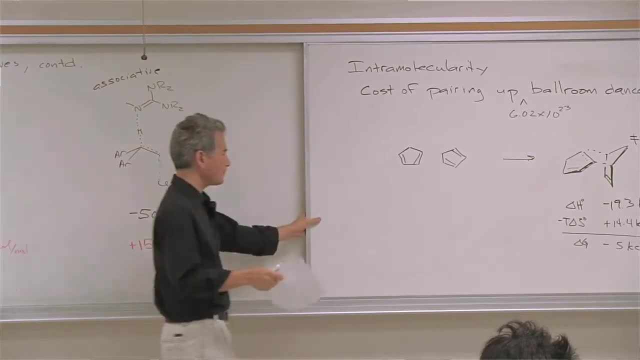 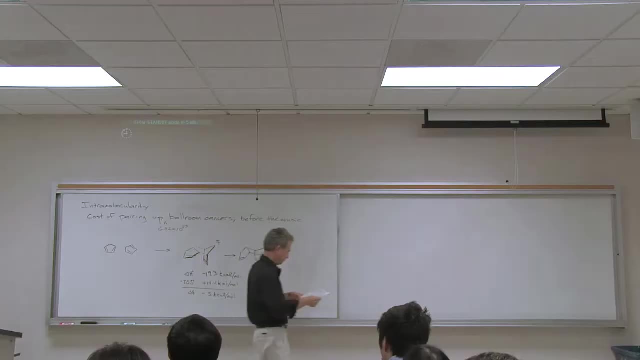 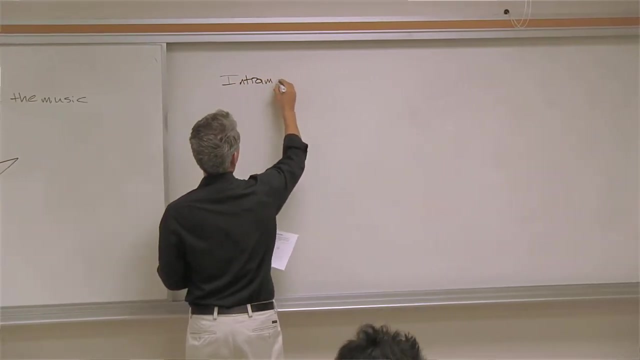 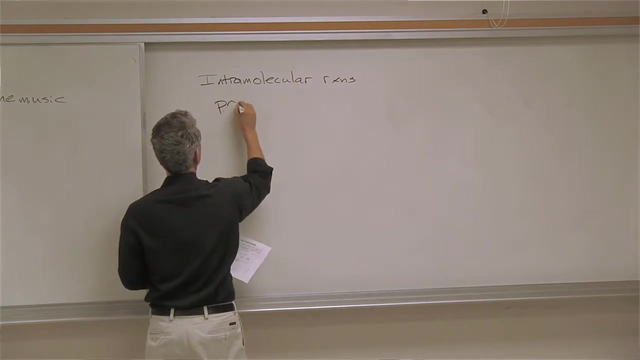 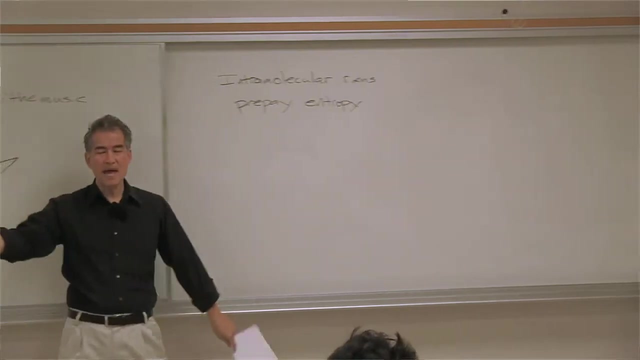 bonds because it's entropically expensive to bring things together. Okay, so how do you win? One way to win that's very common is to make reactions intramolecular. They prepay those T, delta, S quads. That's cost in the transition state. 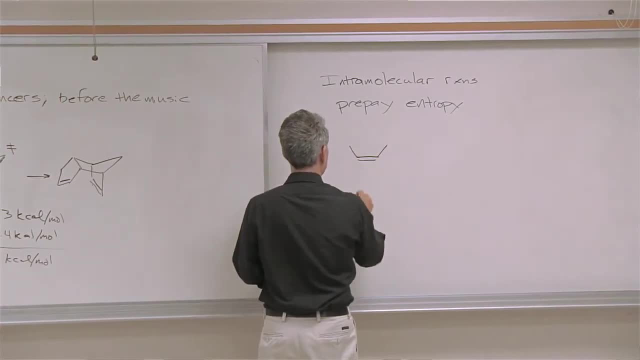 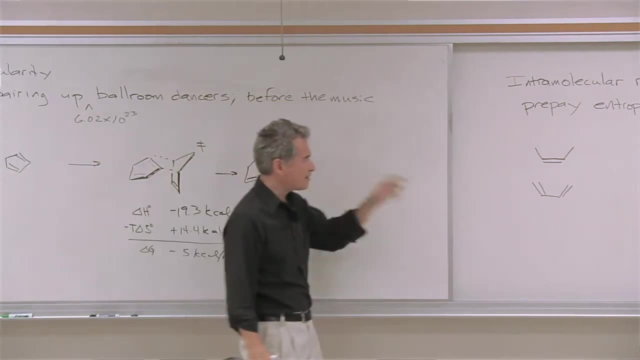 So let's take an example of two Diels-Alder reactions. Here's a kind of. this is a slightly more expensive in terms of the entropy of activation in the transition state because I have to freeze out this S cis S trans confirmation for the diene. 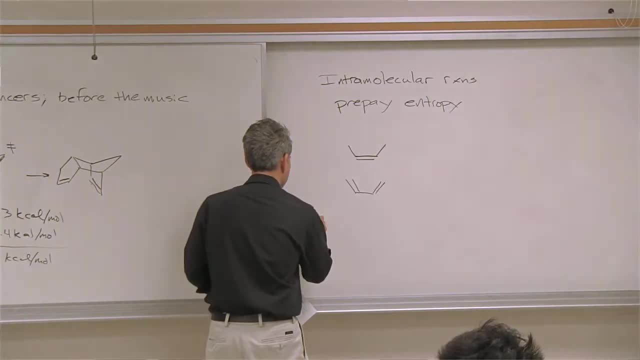 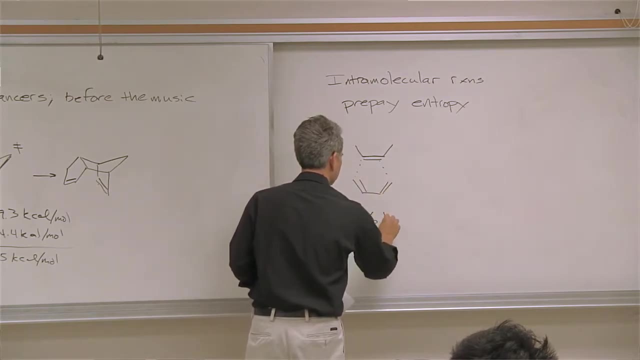 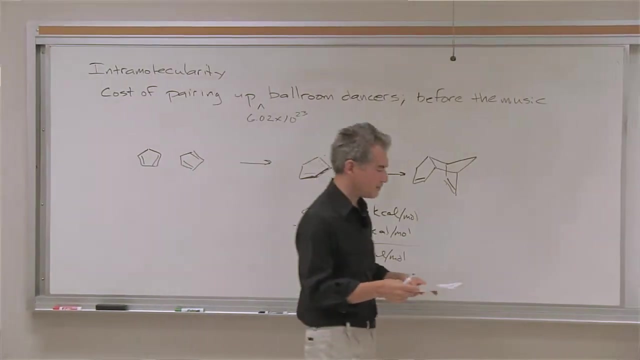 It's a little worse than cyclopentadiene. If you look at the costs in the transition state for this Diels-Alder reaction, it's about 16 kcals per mole uphill. That's the entropic cost. I'm bringing those molecules together, making the diene adopt a cysoid confirmation. 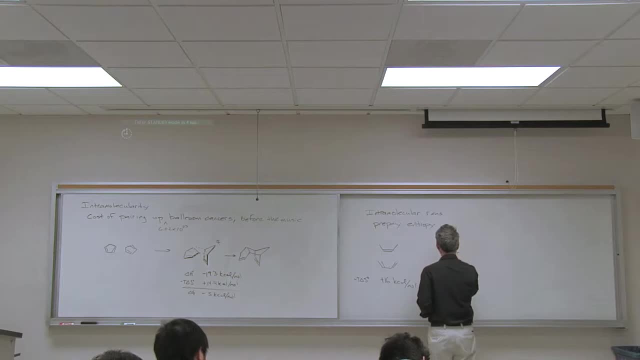 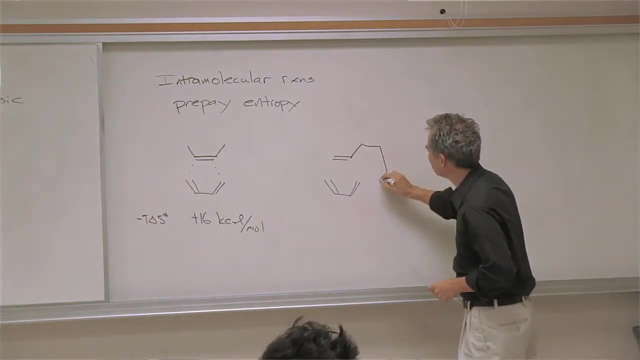 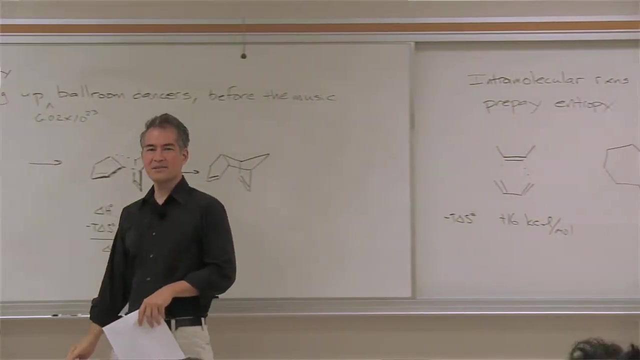 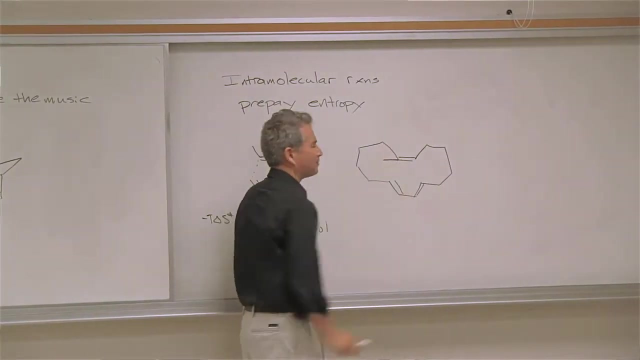 But if I take a very similar reaction and I simply join these two substrates together, imagine how restricted the you're starting off with these things very close to each other. What I have a number for is the one where there's a methyl group. 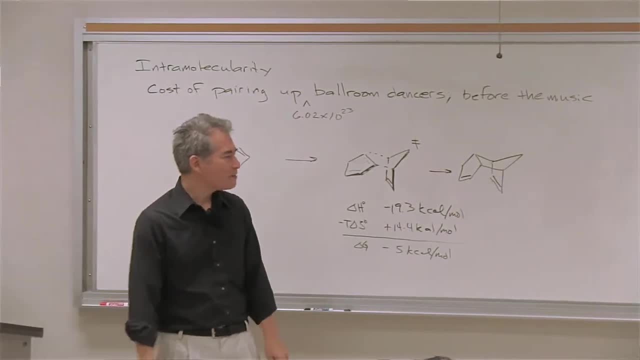 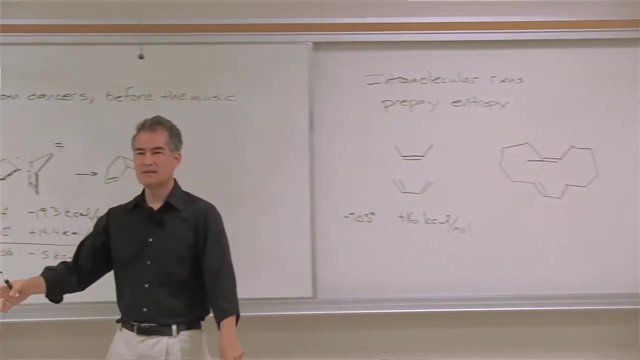 Here, But pretty similar right. By having rings on both sides, these are held close together all the time. It's like you get to prepay this cost of going from infinite numbers of confirmations. You don't start from infinite numbers of confirmations. 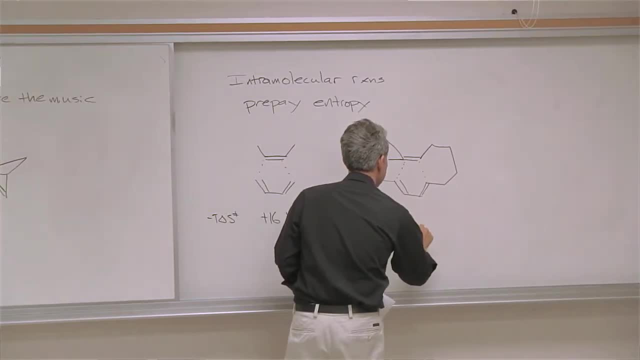 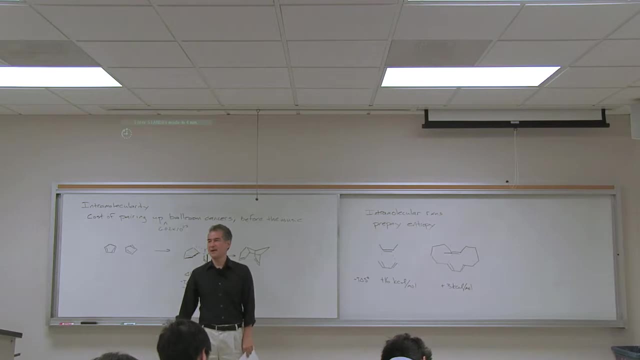 And so when you look at the entropic cost in the transition state, instead of being 16 kcals per mole for this reaction, it's only three. That's why intramolecular reactions are valuable. This is kind of an extreme example. 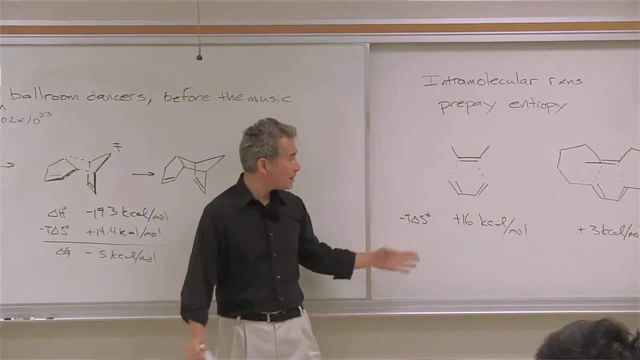 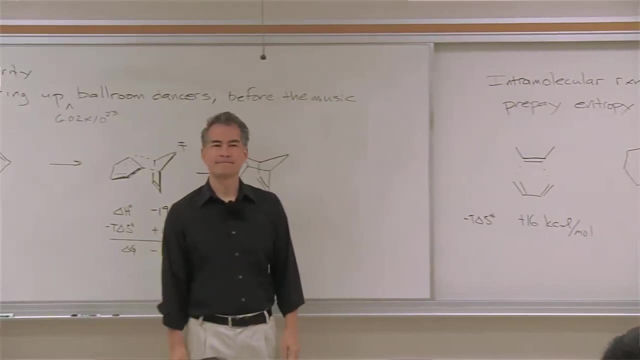 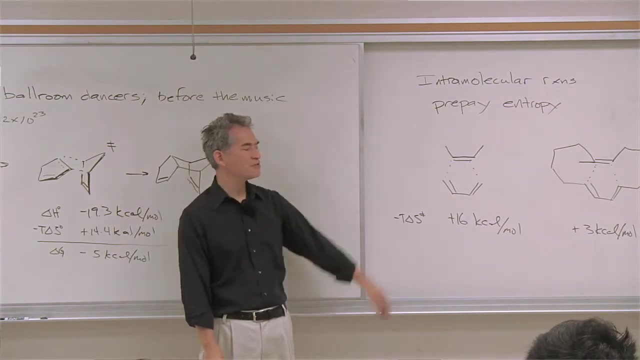 Because it's we've locked it on both sides. So how many times faster do you expect this transannular Diels-Alder reaction to be than this simple intermolecular case? Just in terms of entropy acceleration, How many kcals per mole difference? 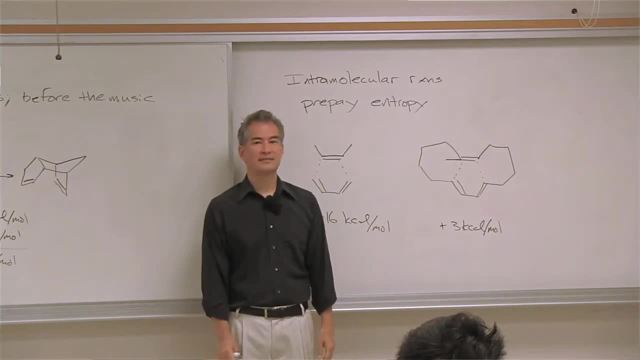 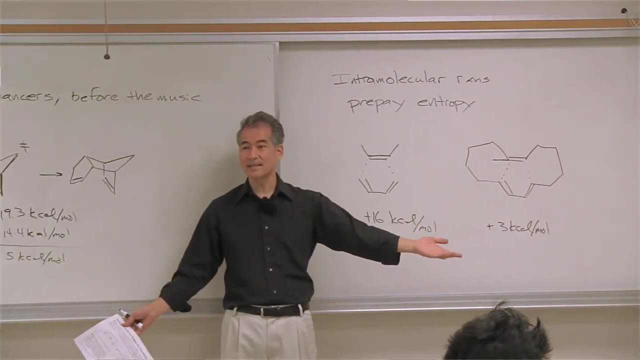 13. How many factors of 10 is that 12.? If we divide by one, it's 13 kcals per mole. divide by 1.4, that's something like nine. You expect this to be a billion times faster just because of what you're buying yourself. 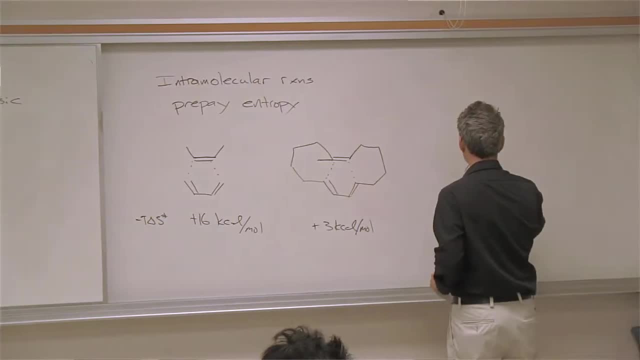 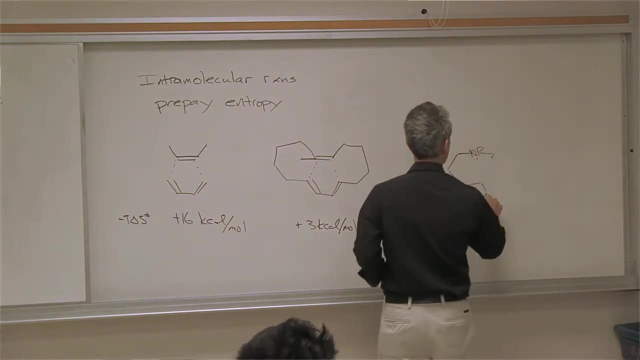 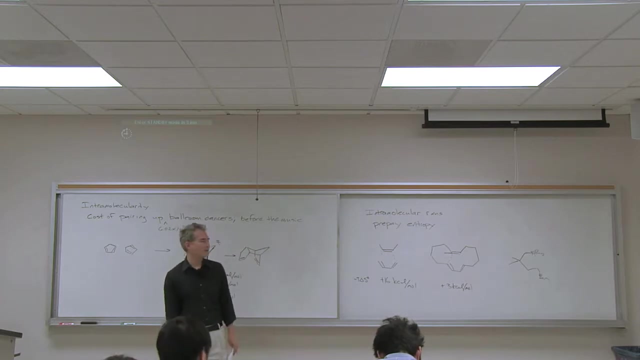 in terms of entropy. So this is why it's so common in organic chemistry to see reactions that look like this, Where you're forming some sort of five member ring. It is cool to form rings. Lots of things we care about have rings. 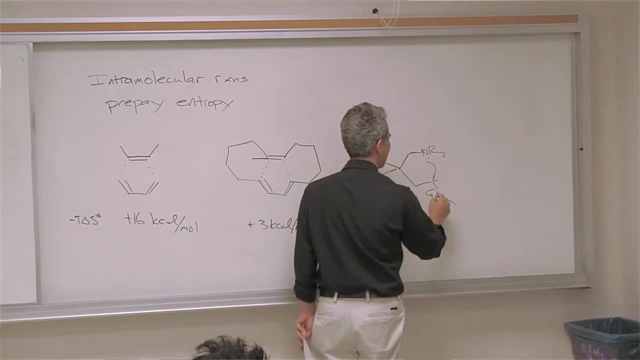 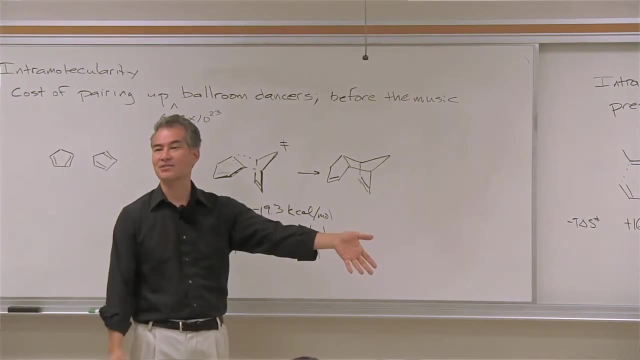 But the main advantage When you're doing some methodology project is you're making your reactions entropically easier. You're cheating. You're cheating on entropy If you really want to impress people. do intermolecular reactions. Those are hard. 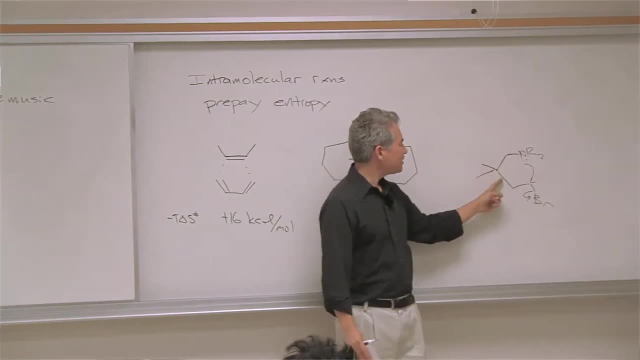 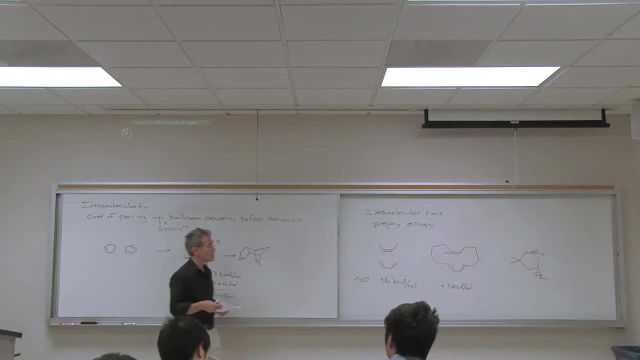 Right. Once you bring these things close together by tethering them, there's only so far apart that they can get. You're prepaying in a huge way those costs of entropy. So reactions in general that involve five member or six member transition states intermolecular. 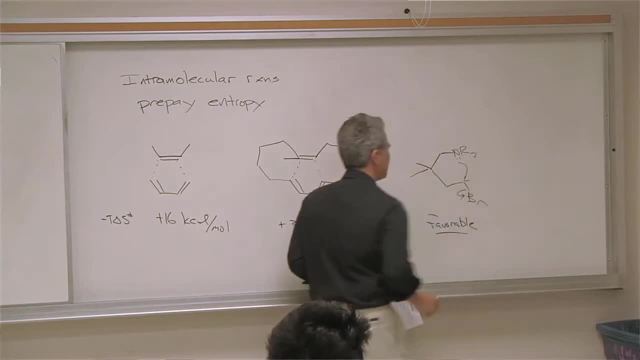 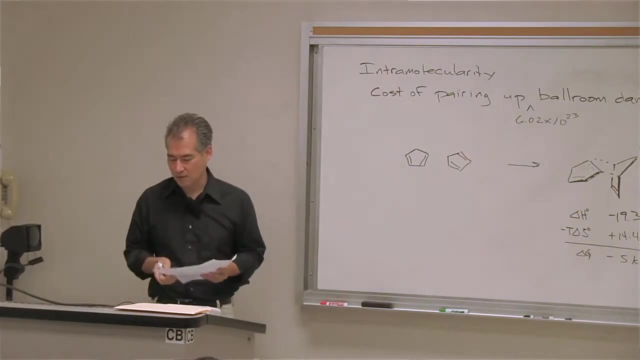 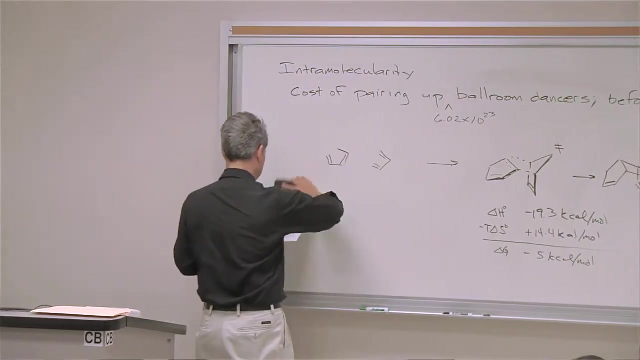 reactions Depend from entropy. You prepay the costs of entropy, Costs that can be as high as 15, 16 cake house per mole can be the entropic costs. So intermolecular reactions are common. OK, Let's try to put this together in a reaction coordinate diagram. 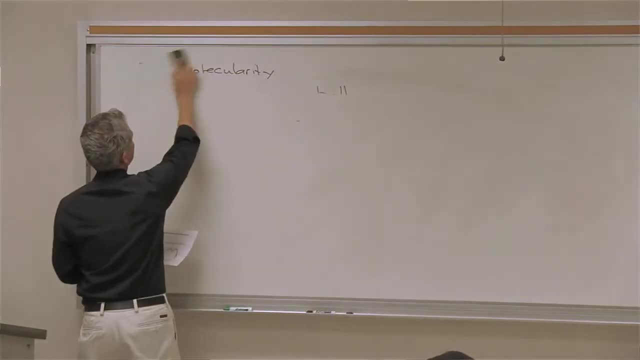 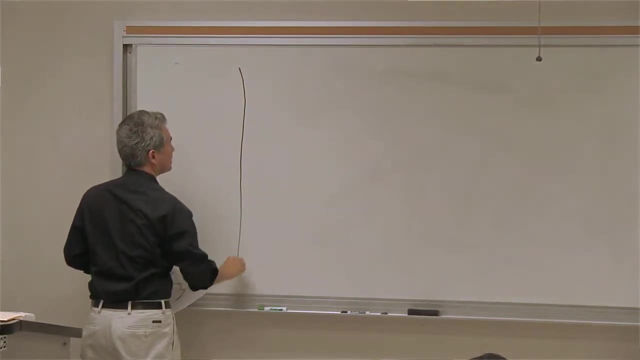 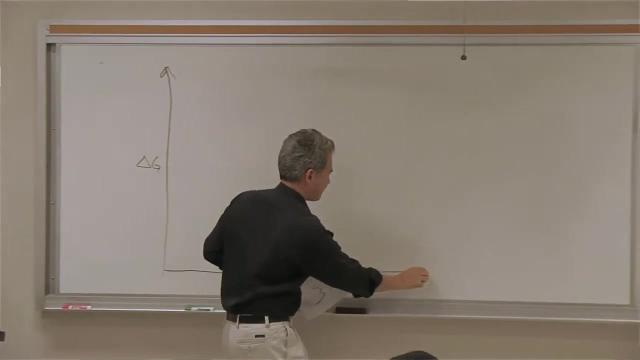 It seems kind of abstract to talk about entropic costs in transition states. So I want to paint a picture of a reaction coordinate, A coordinate diagram for a simple- I don't know a simple reaction, but simple in terms of number of steps. 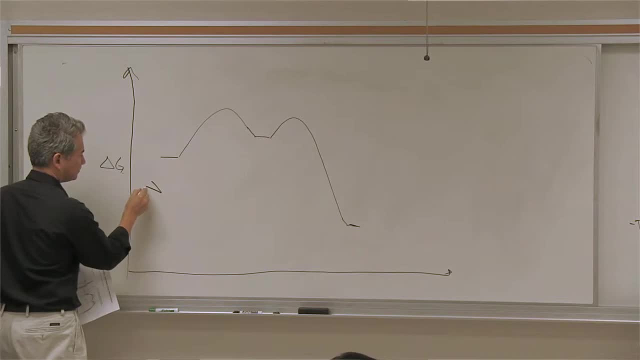 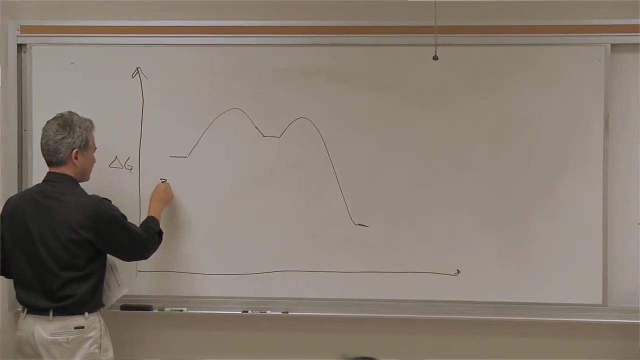 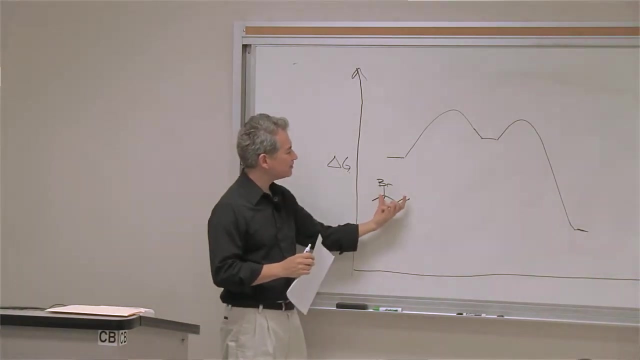 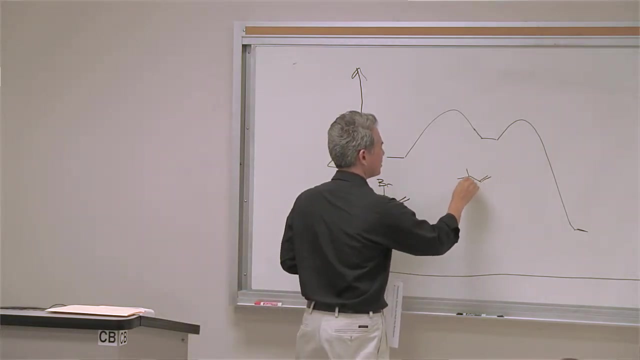 So let's imagine we have this allylic halide And we want to do a cycloaddition reaction with the cation. So if I make the leaving group leave, I've got a two electron system. still here There's a carbocation. 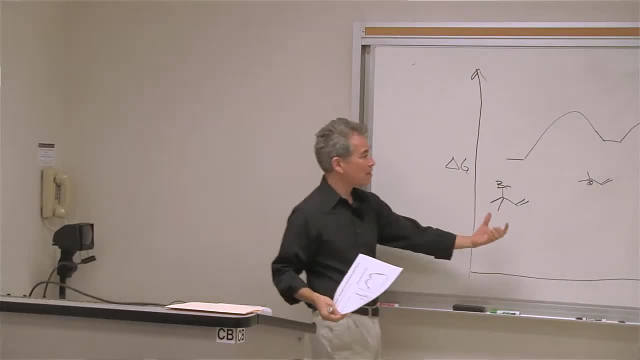 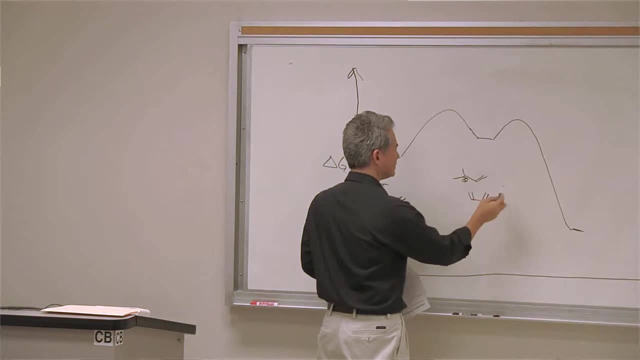 But there's only two electrons in the carbocation, So I can A reaction with a four electron component. Two electrons, four electrons. Let's imagine what that would be like. You'd push the arrows. It would look something like this: this, this: 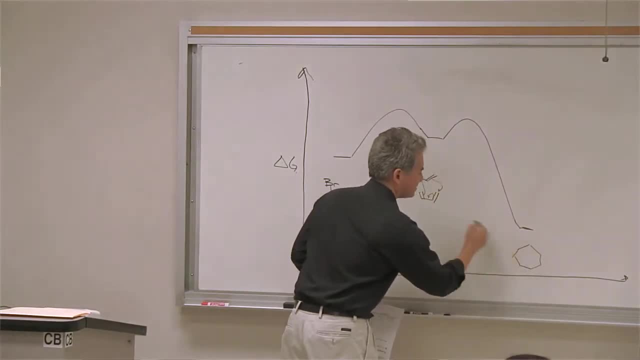 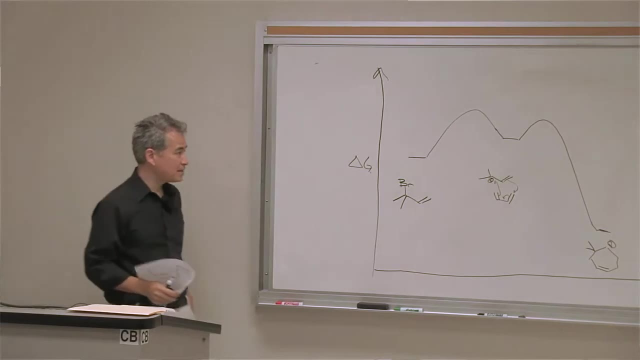 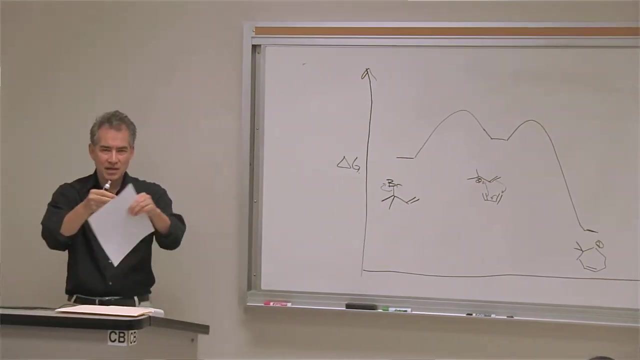 And you'd end up with some seven membered ring, And there are not this simple example, but there are examples of four plus three cycloadditions. And there's two steps in this process. One step involves ionization of this bromide. 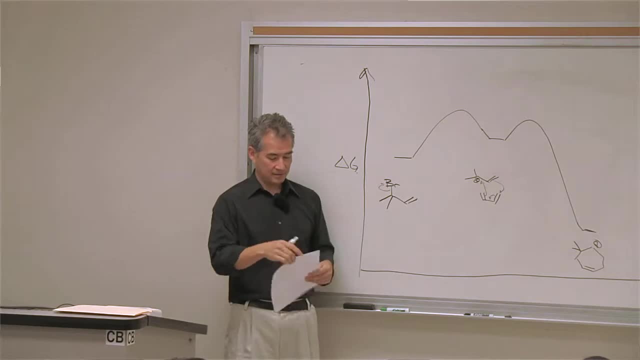 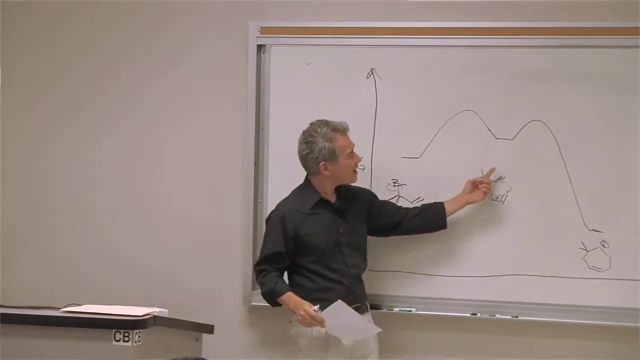 These are coming apart, And tropically that's good. It's good to have things come apart in a transition state. Right, You can become more disordered, But then in this second step, this is going to be a very entropically demanding transition. 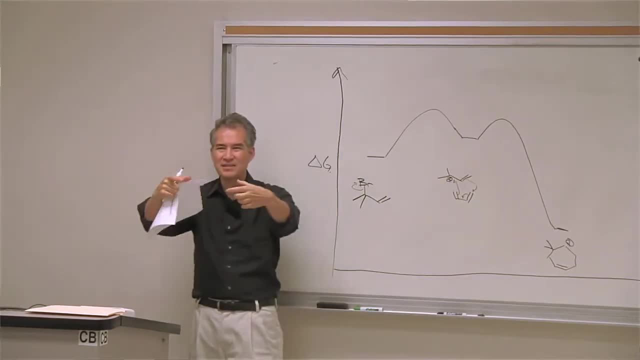 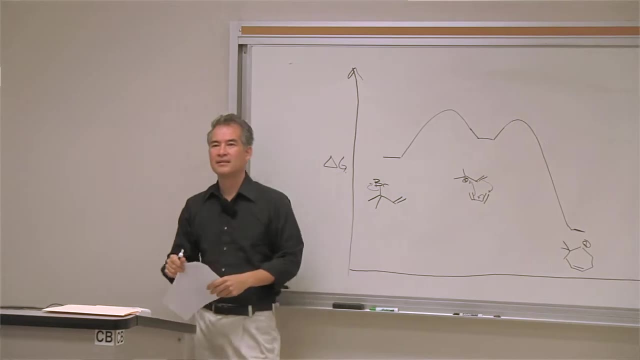 state Right now. it's like a Diels-Alder reaction, where I have to bring the two pieces together and simultaneously collide so that this atom is close to that one and this atom is close to that one over there. That's an entropically expensive transition state. 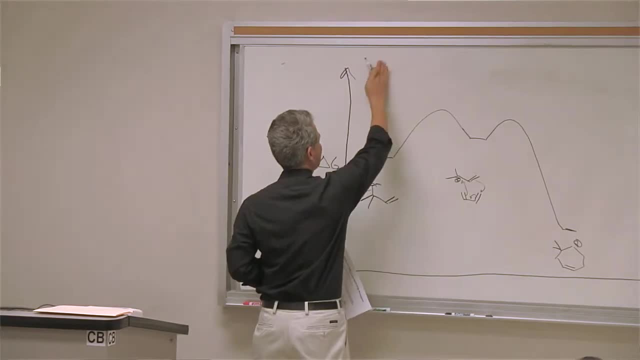 So what you can imagine: as you increase the number of electrons, you're going to have an entropic transition state. So you're going to have an entropic transition state As you increase temperature. let's try to imagine this. Let me use a different colored pen here. 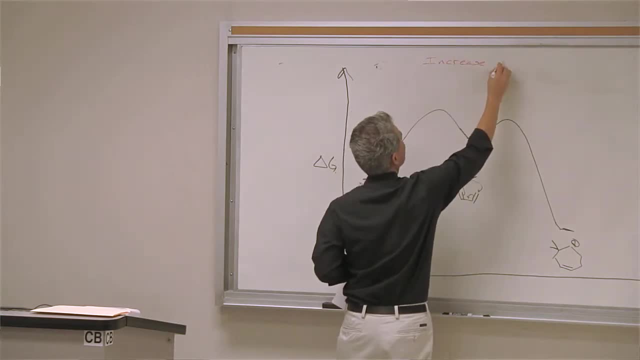 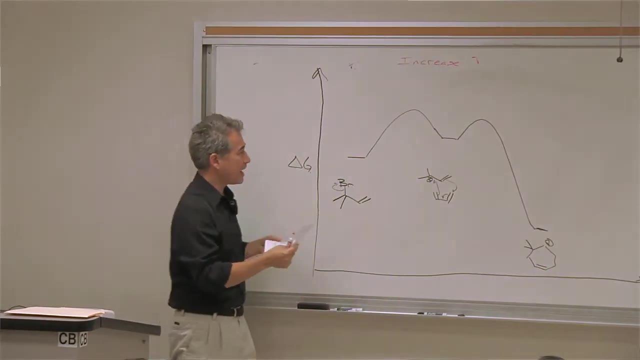 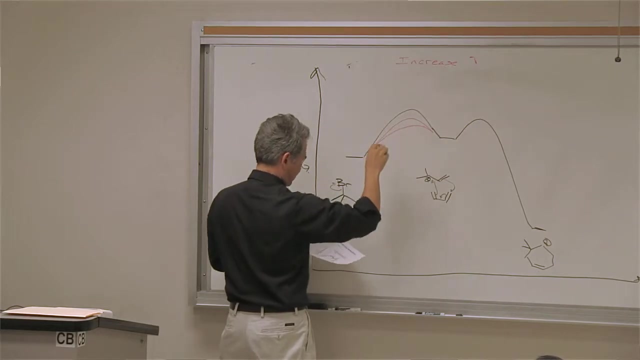 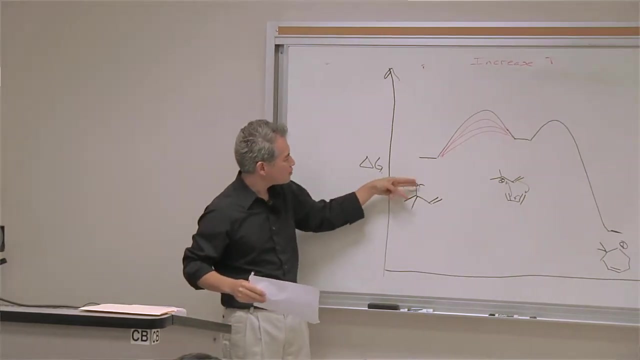 As you increase temperature. what do you expect to happen? So, as you increase the temperature, what you might expect is going to happen is that this entropically expensive transition state is going to start to get lower and lower and lower. That's beneficial to heat things up, and let this explore all these other conformations. 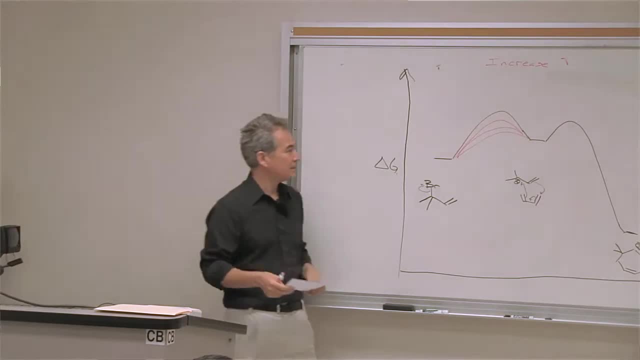 where bromide is going to be. The bromide is not so close to that aloe piece, But over here on this second step, let me try to draw out an arrow here so we can be clear. Here's what's happening as we increase the temperature. 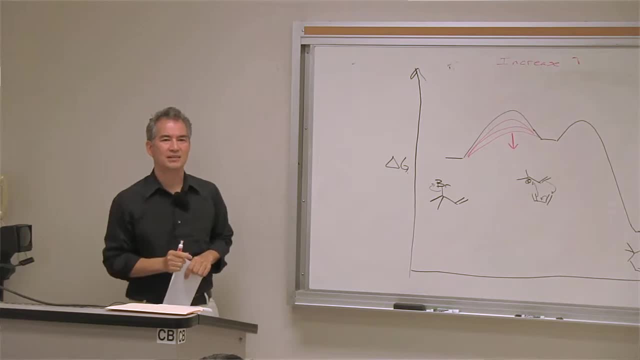 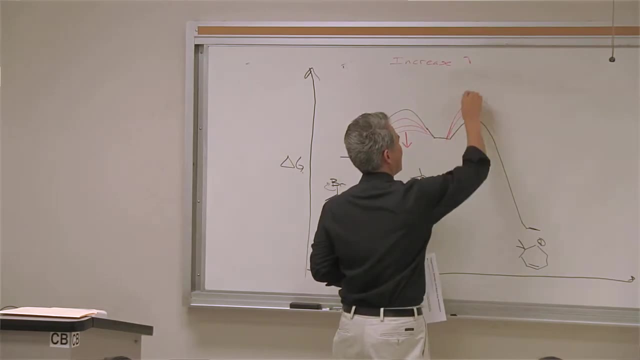 That barrier is going to get lower. But in the second step for this reaction, where you have to bring things together in this very precise way, what you can imagine is that the activation energy barrier will increase, And so this is the way you have to imagine the effect of temperature. 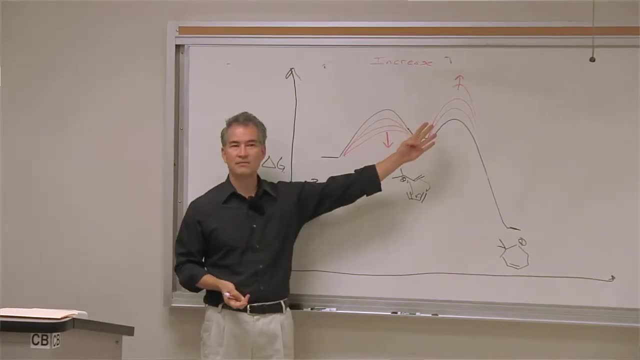 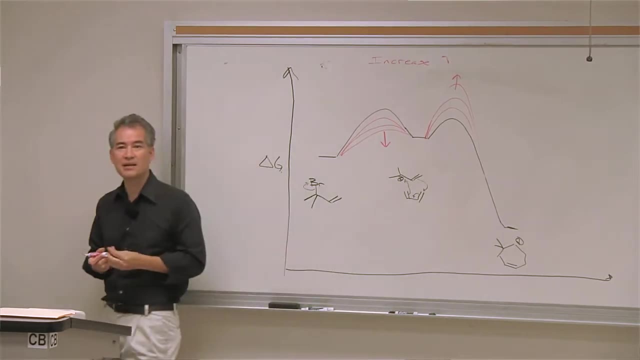 The effect of temperature on reactions depends on what's happening, What's happening in each of those transition states. Some transition states can go up in energy if they're entropically expensive. Some transition states can go down in energy And all of those things are happening at the same time. So changing the temperature distorts the energy landscape in your reaction coordinate energy diagrams And it depends on whether you're increasing entropy or decreasing entropy in the transition state. Now the benefit of going to higher temperature: you change the energy landscape, but all reactions. 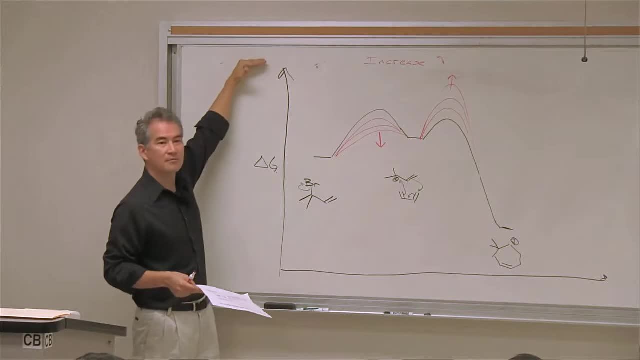 get faster. So as you're increasing the temperature, you're increasing the energy landscape. As you're increasing the temperature, you're also increasing the number of molecules that can make it over these barriers at the same time. So all of these things are happening at the same time. 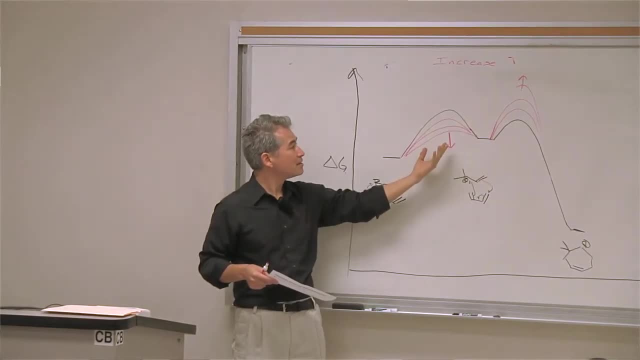 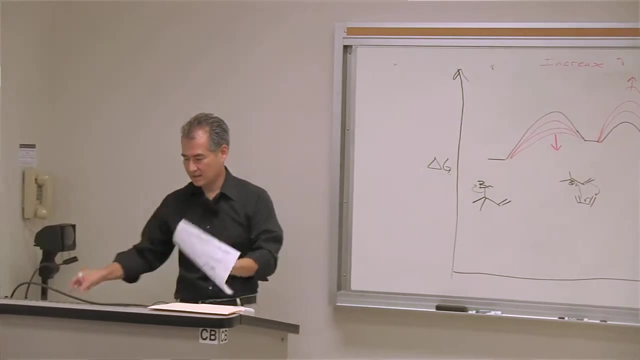 So it's good to keep in mind the fact that you can actually change the rate determining step in your reaction as you change the temperature, And it has to do with the entropic costs in each of those transition states And sometimes you want that to occur. 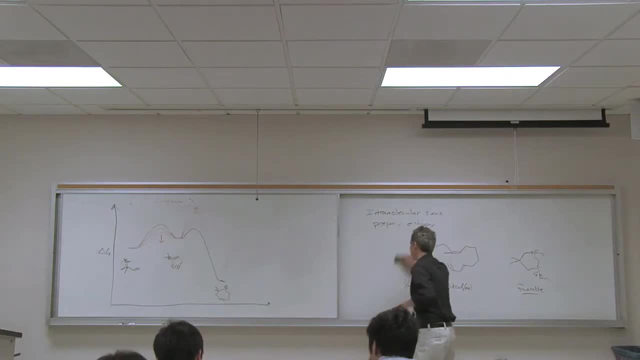 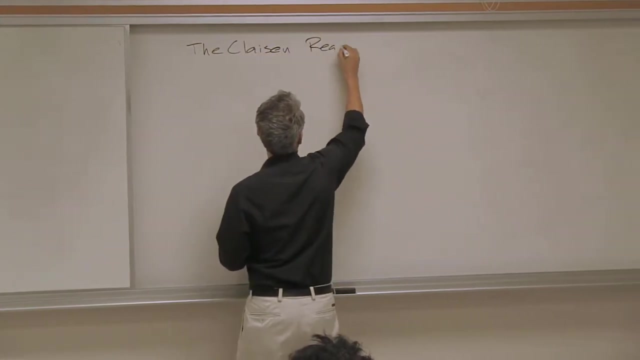 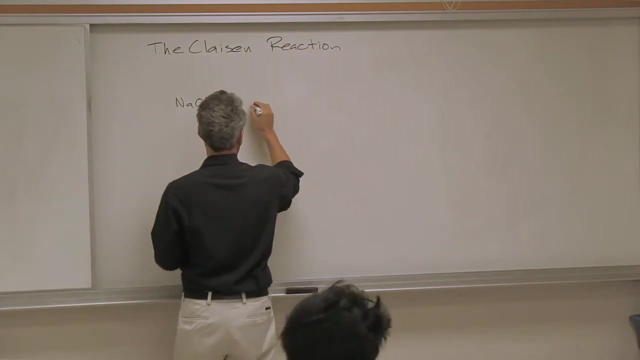 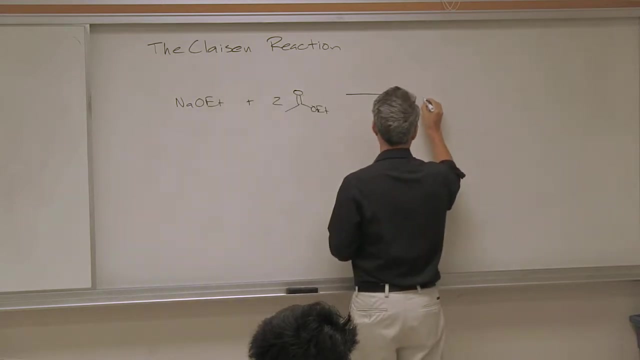 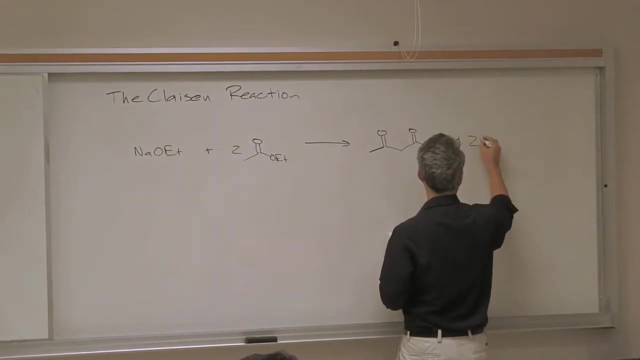 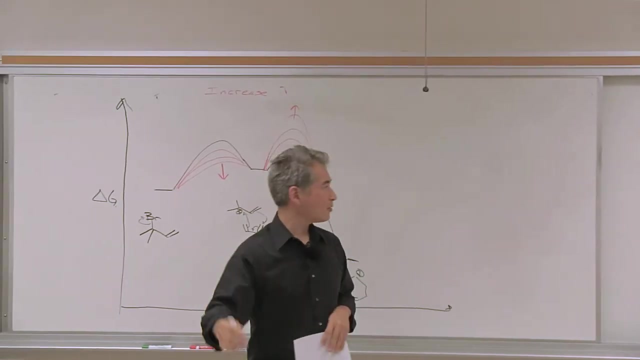 That's one of the things that happens. when you screen reaction variables, You can sometimes end up with very beneficial effects by changing the temperature. We're used to seeing a lot of that. It's called a Claisen reaction. it's a carbon-carbon bond forming reaction. 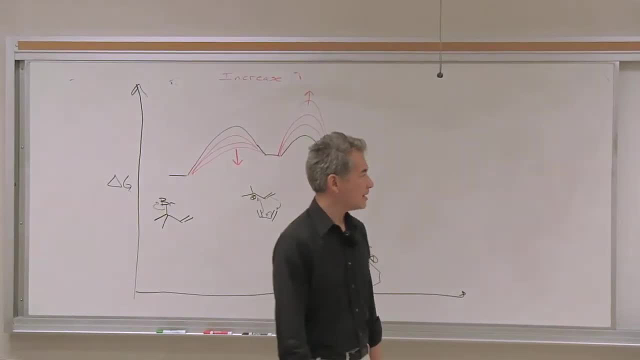 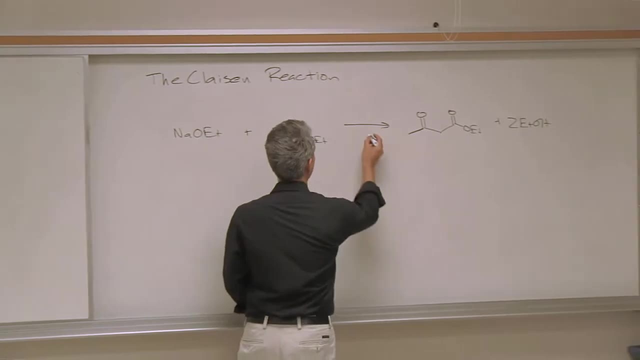 I'm going to teach that next quarter when I teach a sophomore organic chemistry class, And it's not a favorable reaction. in fact, this is an equilibrium process. You don't do many equilibrium reactions, And so the problem with this reaction is that it's not favorable. 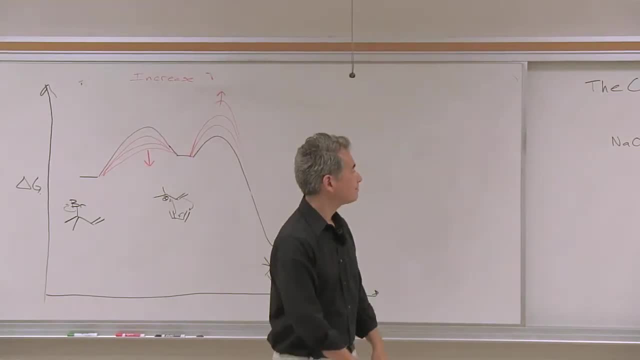 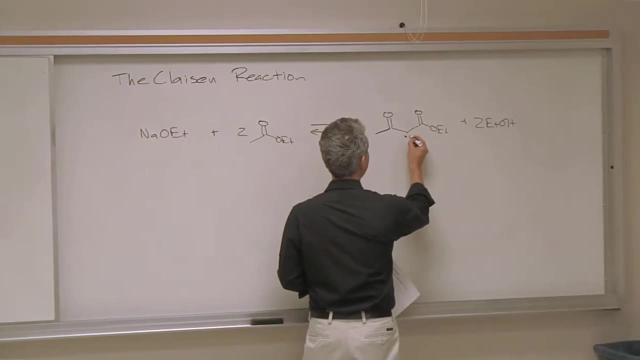 And so how do you make a Claisen reaction favorable? Well, what you do is you add a base in there like this one, and then you end up with this highly favorable carbanion and you can draw that as the enolate, actually the sodium is. 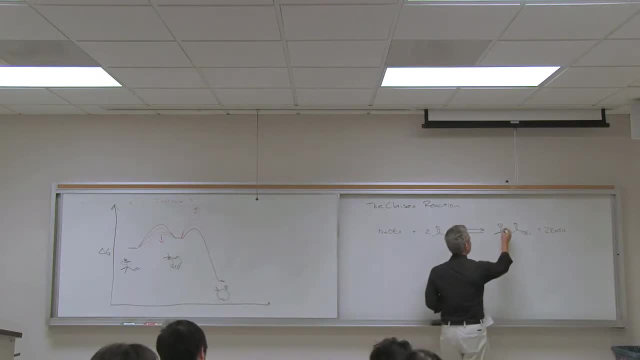 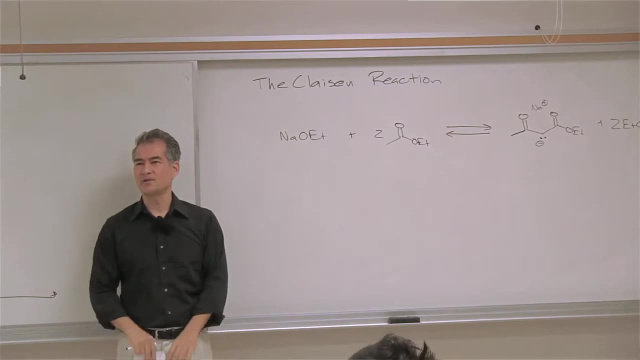 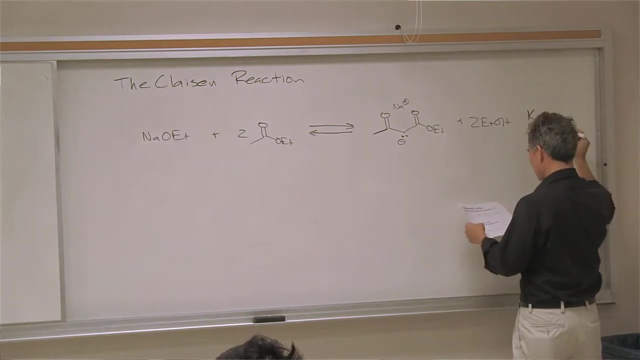 coordinated to the oxygen in the product. That's the classic way of thinking about what favors the why. the Claisen reaction should be favorable. It's still not favorable Even with that sodium ethoxide in here as the driving force. the equilibrium constant. 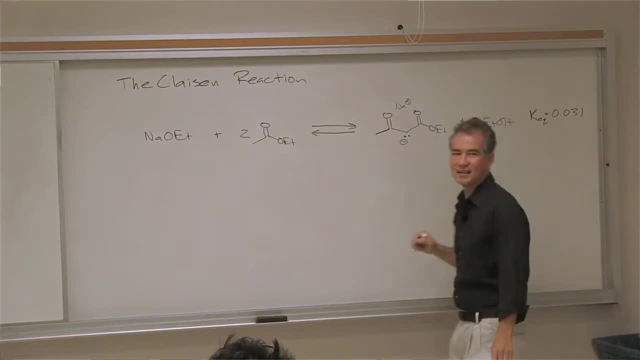 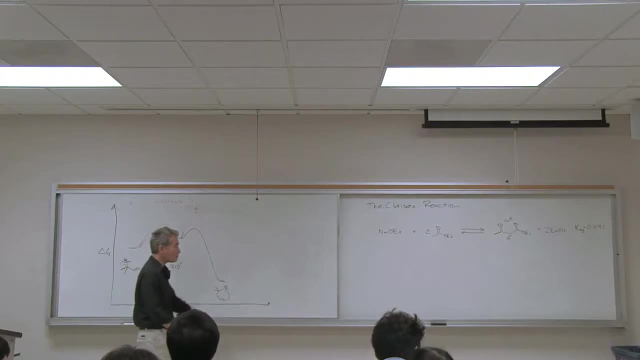 for a Claisen reaction is this: It's highly unfavorable, even when you use this deprotonation trick, And so why is it that people use? how are people at all able to do a Claisen reaction in organic chemistry and get decent yields out of that? 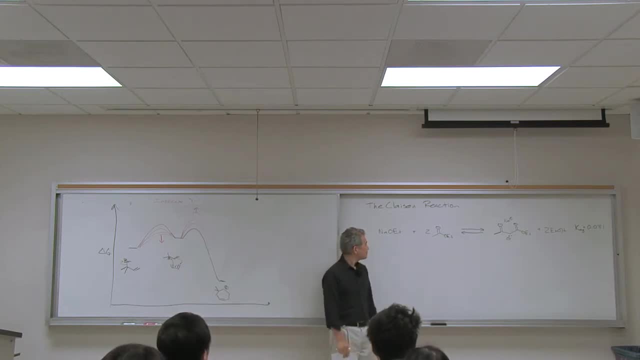 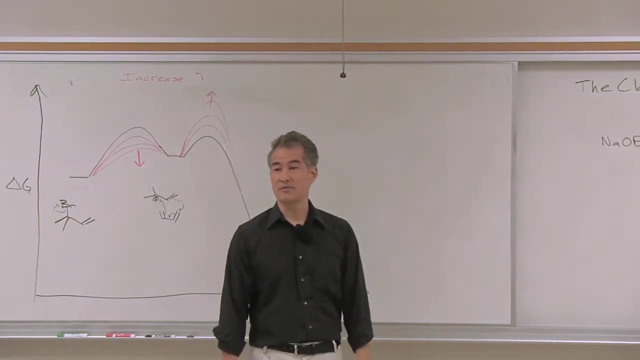 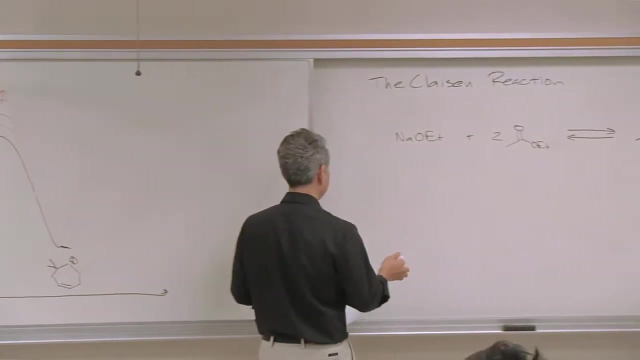 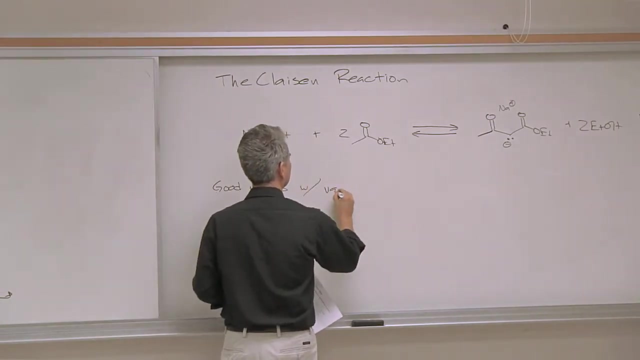 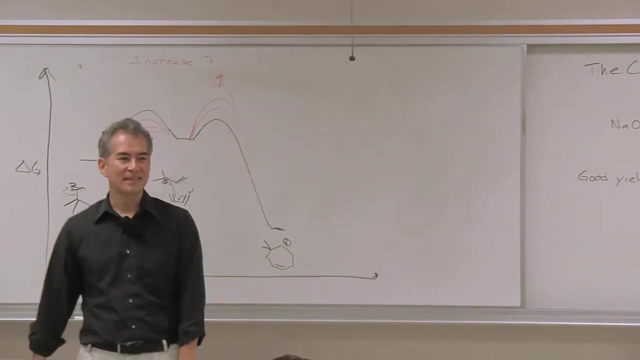 Lewis acid won't help you change the thermodynamics. It's a catalyst. A catalyst will just accelerate the rate at which you reach equilibrium. He used vast excesses of the reagents. That's how you win. That's how you're able to make the Claisen reaction work. 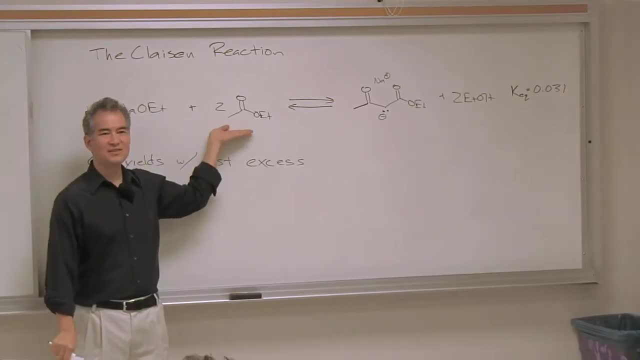 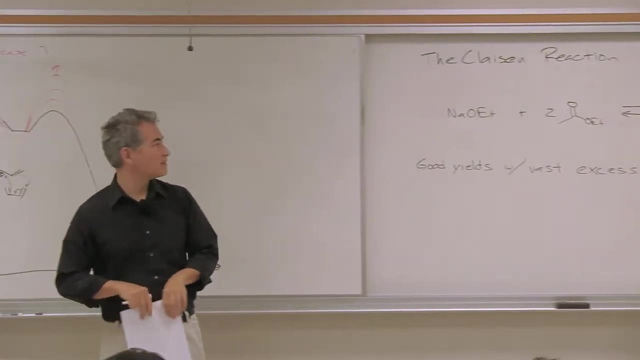 The only way to get good yields out of this simple Claisen reaction is to use this as your solvent for the reaction. That's how you get yields that are worth talking about Only when you use that as a solvent for the reaction And so use vast excesses of that. 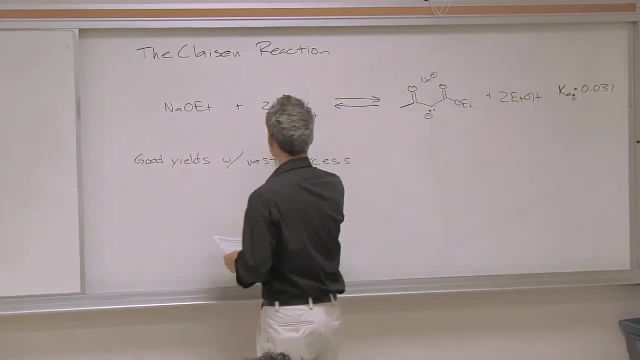 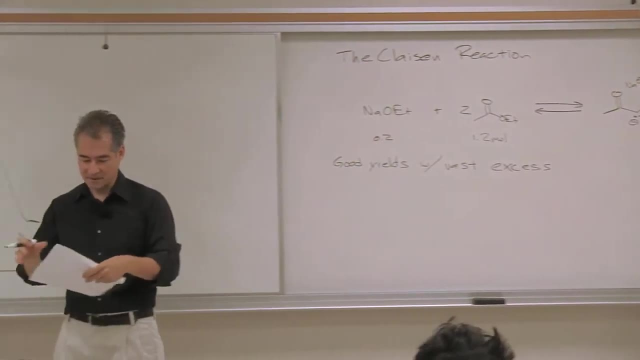 And you still don't get a good yield actually. So just to put things into perspective, if you use big excesses of one of the ethyl acetate, which is cheap, You still have to base the yield on your sodium ethoxide in order to get what would be a worthwhile 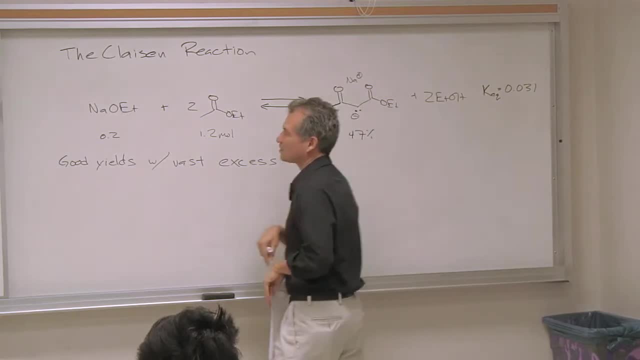 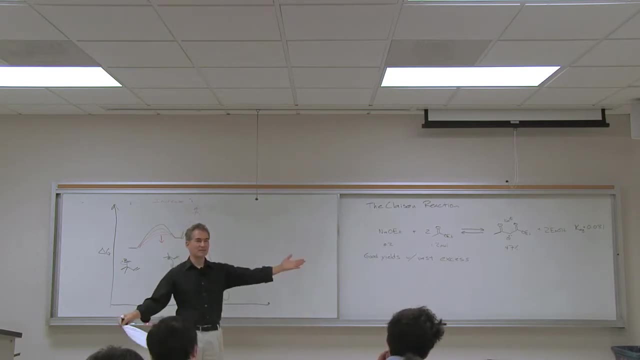 talking about yield. So if you base the yield on the sodium ethoxide and use huge excesses of the ethyl acetate, you can get a 47% yield And that's determined by thermodynamics. You can't change that feature of the reaction. 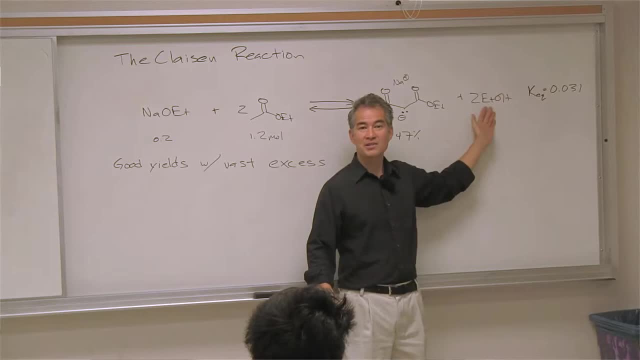 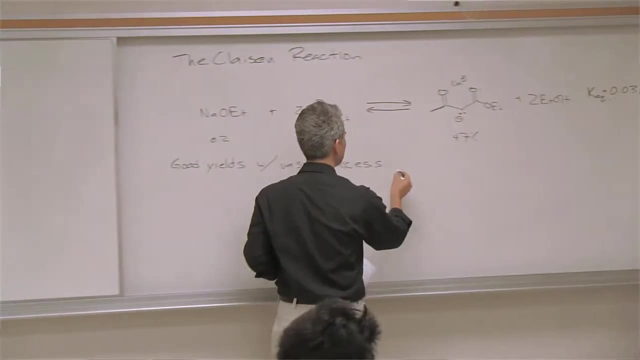 Now, if you're really tricky, you can try to remove ethanol from the reaction by distillation, And that's the way to bring the yield up, And without doing those things you'll never get a good yield in this reaction. All of these things I'm talking about are based on Le Chatelier's principle, where you 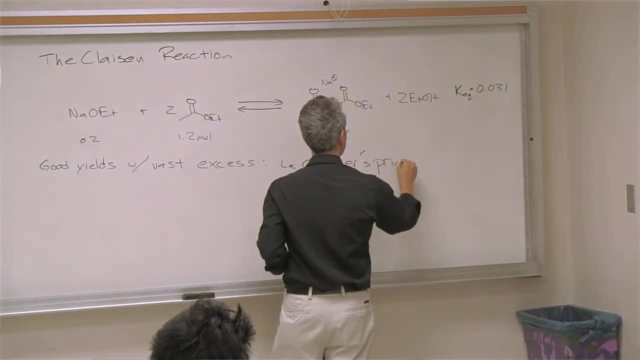 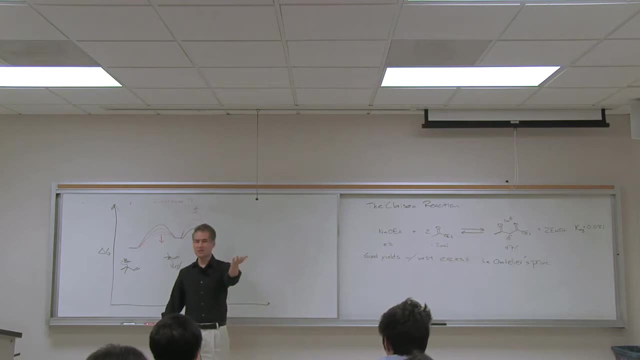 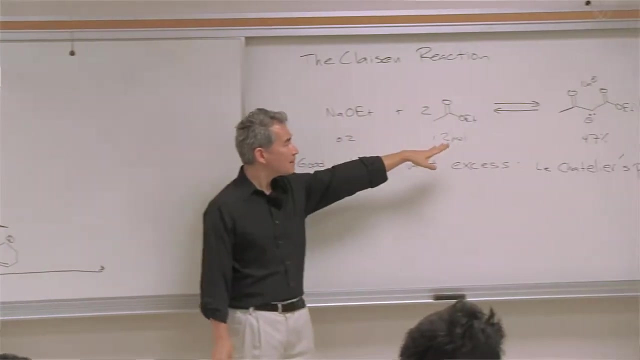 can drive reactions to completion or further towards products by removing products from the reaction or by using vast excesses of the reagents, And you can do this in the lab to make your reactions work faster and better. Excess reagents can drive reactions thermodynamically and it can also make reactions faster. 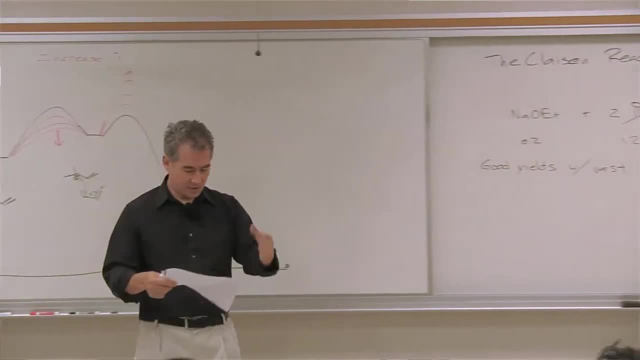 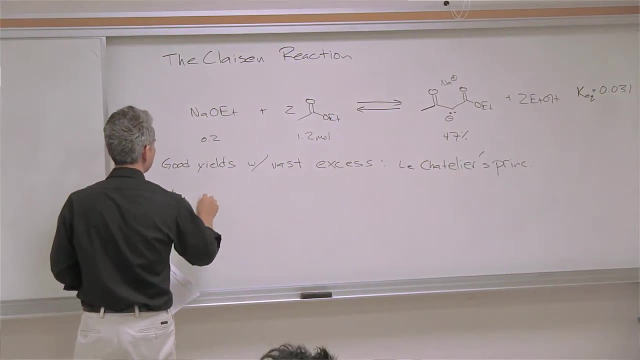 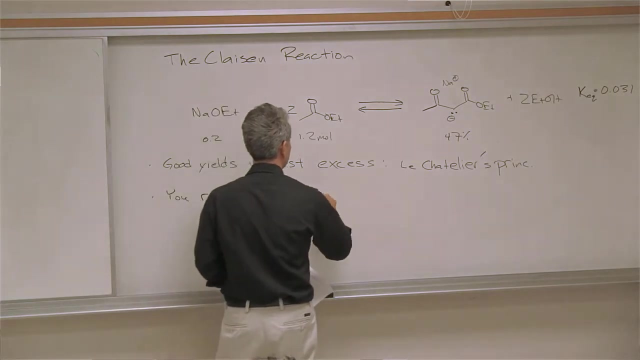 Ten times more, ten times faster, that kind of thinking. So you can do that in the lab And you should do that in the lab. Now, in practice, let me just remind you, you rarely run reactions in the standard state. And what is the standard state? 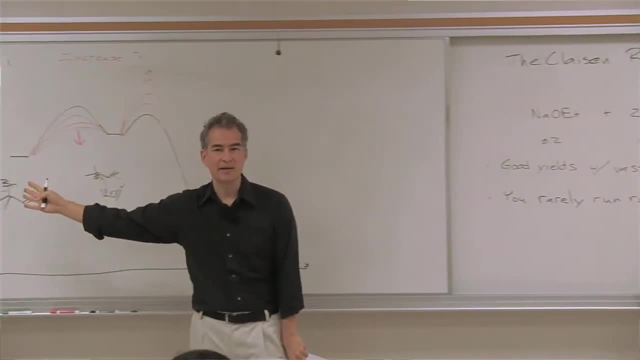 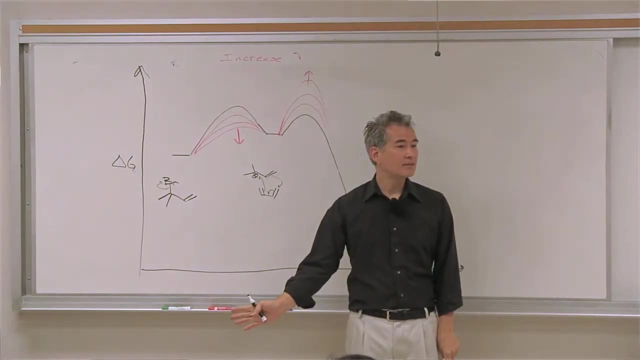 The standard state for all of these reaction coordinate diagrams we've been talking about is one molar. You'll assume that everything is present at one molar: Your palladium catalyst, your substrate, carbon monoxide, all of these things are present at one molar. 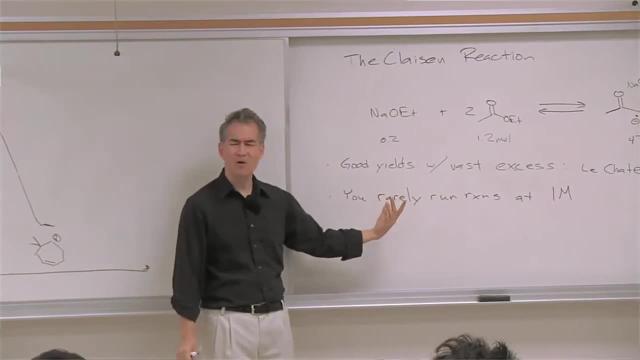 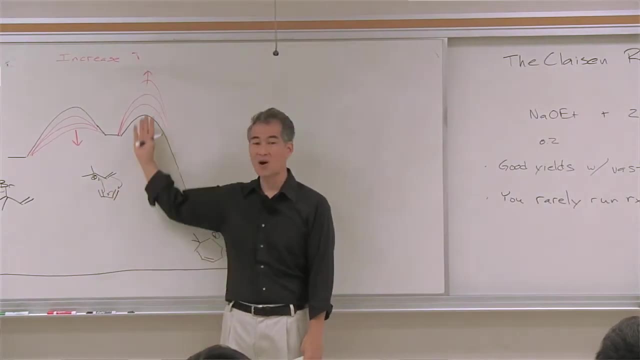 But you don't actually run reactions under those conditions. You kind of have to back out. What would happen if I didn't have right? What would happen if I didn't have butadiene in there at one molar concentration? This would be even harder. 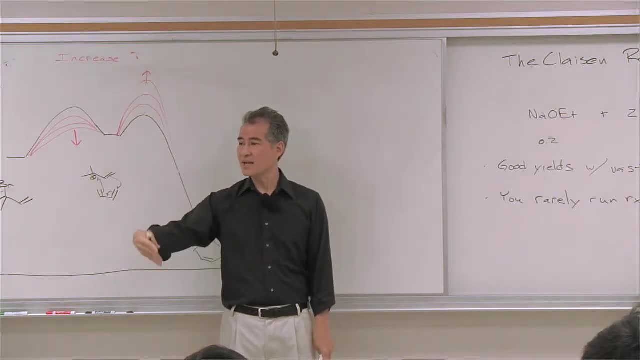 That barrier is going to be even higher if you're not in the standard state. So your thinking ought to be always: start with the standard state and then extrapolate. Okay, but I don't run reactions at one molar. When I set up my reaction, it was only 0.2 or 0.1 molar. More typically, the reactions you run in the lab are in this range of 0.1 to 0.5 molar. That's a typical range. If you do the calculation for number of millimoles you put in divided by the amount of solvent. 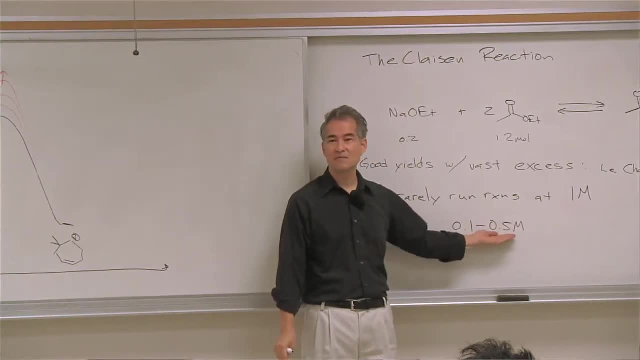 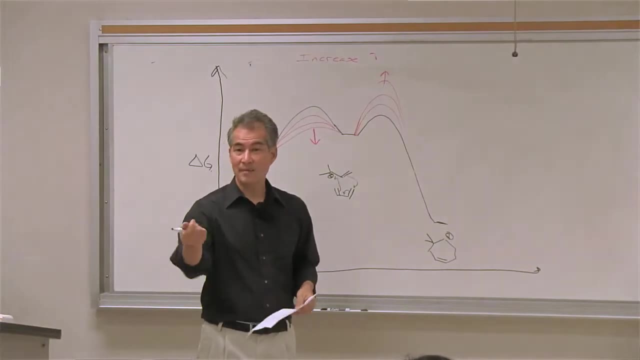 and that's screwing you in terms of your rates. If you want your reactions to work faster, make them more concentrated And they'll be harder to stir. they'll be thicker and harder to stir, but that's the way to make your reactions faster is run them more concentrated, closer to that standard. 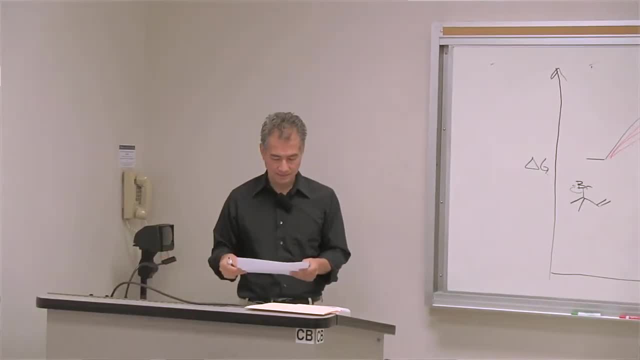 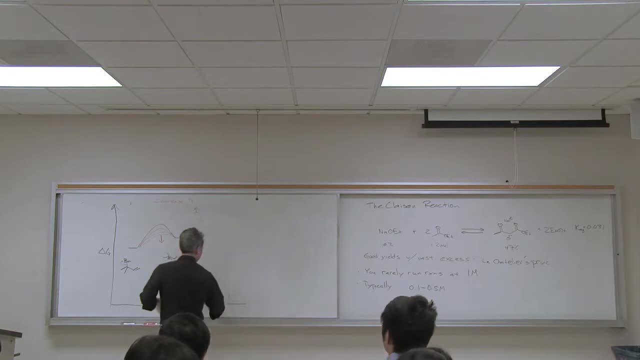 state Or more concentrated, if you could get it more concentrated, Okay. so if your reagents are cheap, add vast excesses. Wouldn't it be great if you could make all your reactions ten times faster and ten times higher yielding? That would be awesome. 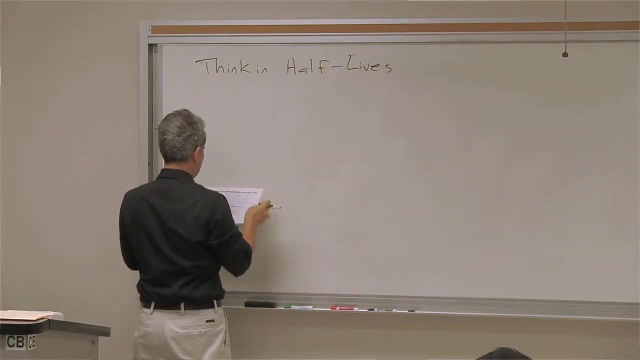 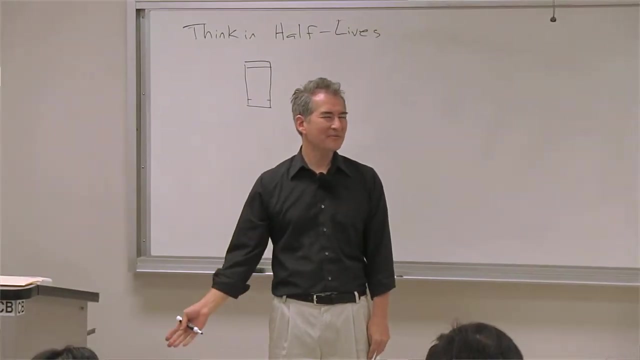 I'm going to draw out a TLC for reaction and the reaction is totally inconsequential. I just want to talk about All this. stuff is nice with free energy diagrams and entropies of activation and rate, But when you go into the lab that's not what you're thinking about. 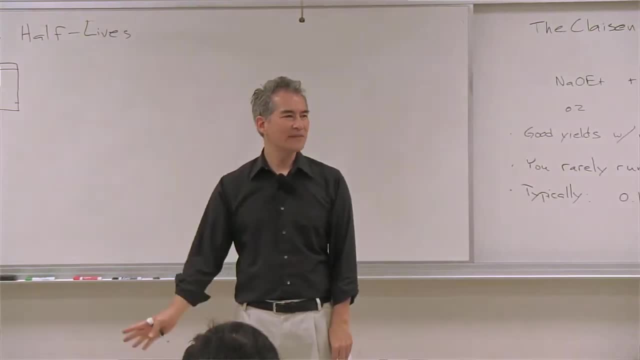 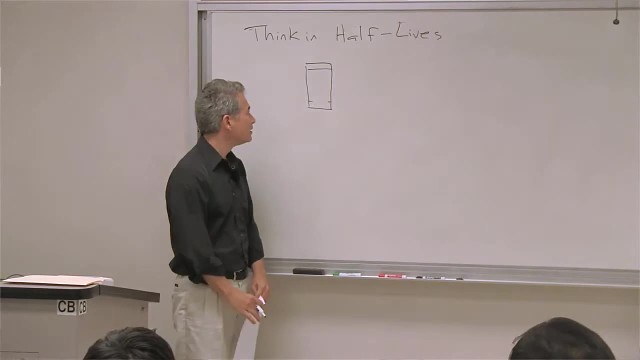 You're just collecting fractions and running some column or looking for the TLC plates, or who took my favorite flask? I thought I left that on the road. That's the kind of stuff that you're worried about. In the lab. you set up a reaction before you go to class and then you jump back to check. 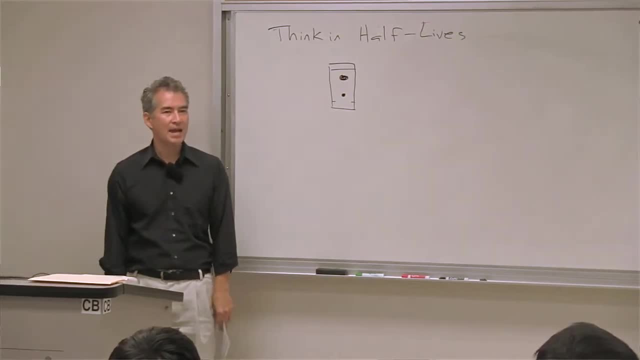 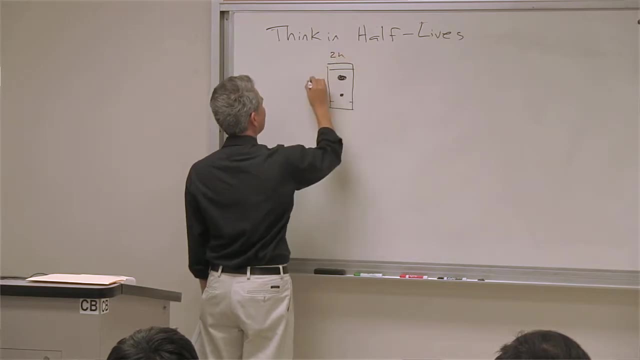 it and it looks like this, And there's no delta G or K or any of this stuff going on there. It's just a TLC plate, which is what you've got to work with. So let's suppose this is what it looks like after two hours. 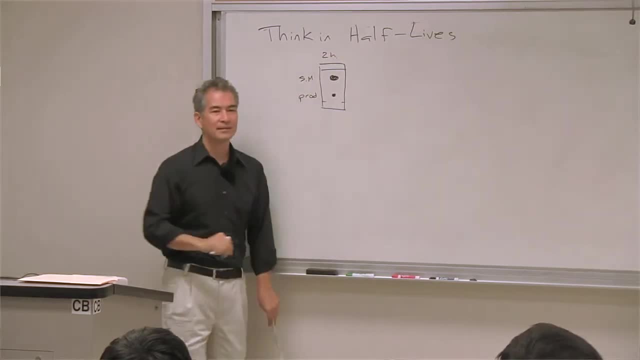 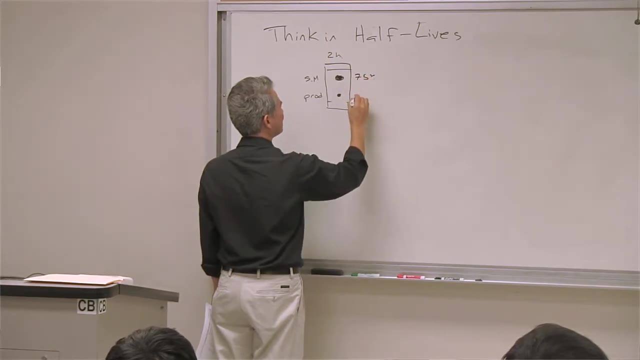 Here's your starting material, and that's great. You've got product appearing and it's growing. It's getting bigger. It looks like I mean you can be semi-quantitative, Nobody cares whether you're on, Spot on with your percentages. 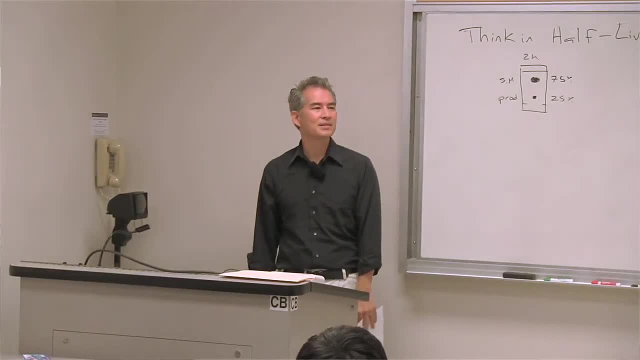 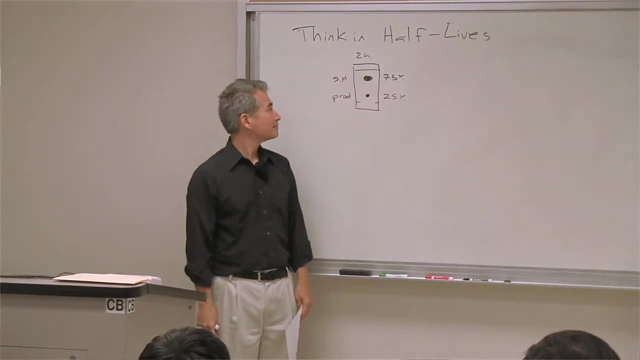 It looks like it's three to one so far, after two hours, and that's a very promising reaction, And so the question is: when is this reaction going to be done? We're two hours in, And why is this important to you? 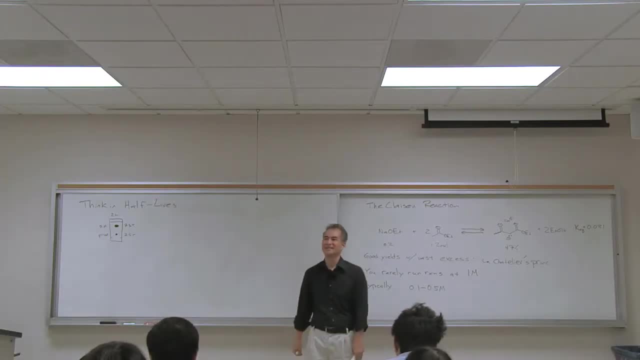 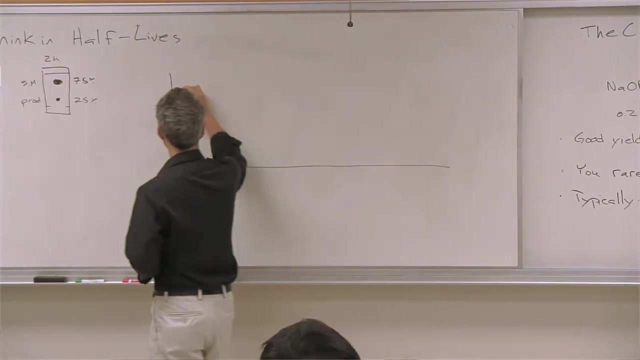 It's important because you have to decide how to use your time for the rest of the day. Let's talk about a reaction. Let's talk about a reaction progress curve. It'll help us understand how to think about this. This is not a reaction coordinate diagram. 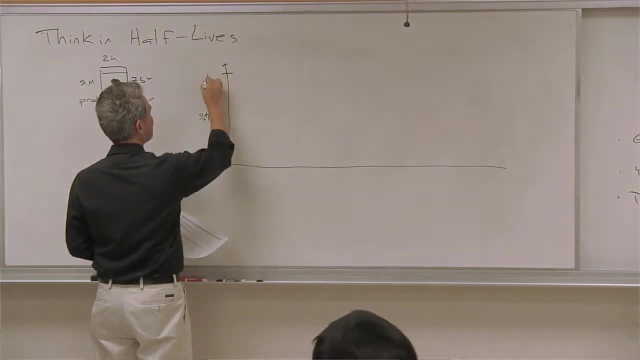 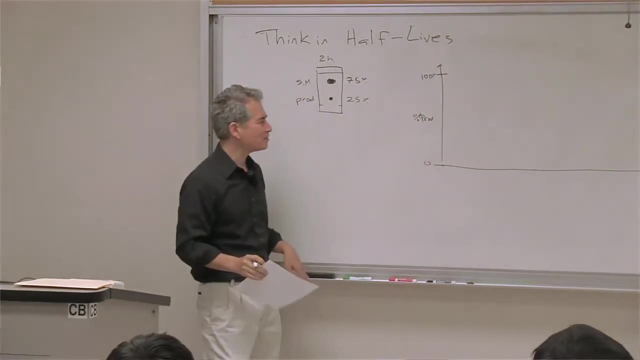 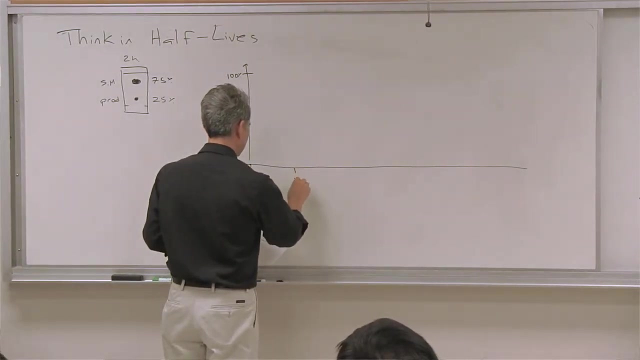 What I'm doing is I'm prodding percent product. The most product you can generate is 100% versus zero, versus time. What does the time course for this reaction look like as we watch product grow in? And so we'll start off over here at 8 am. 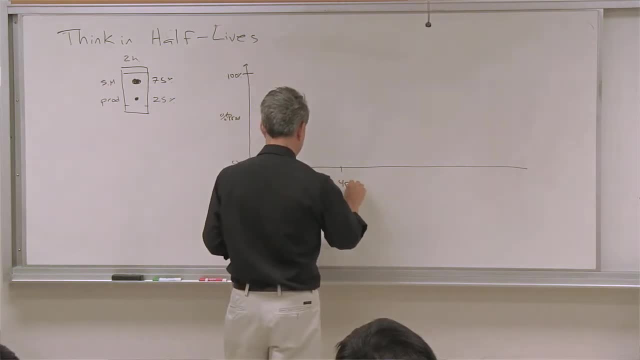 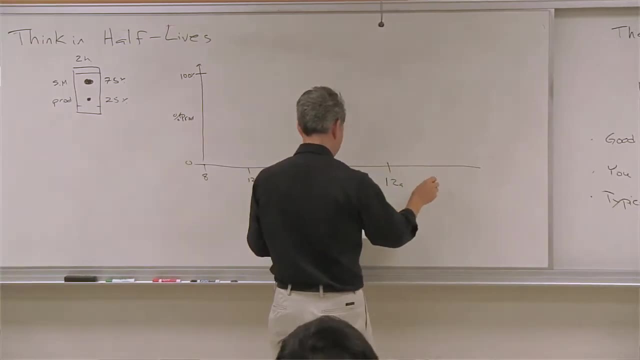 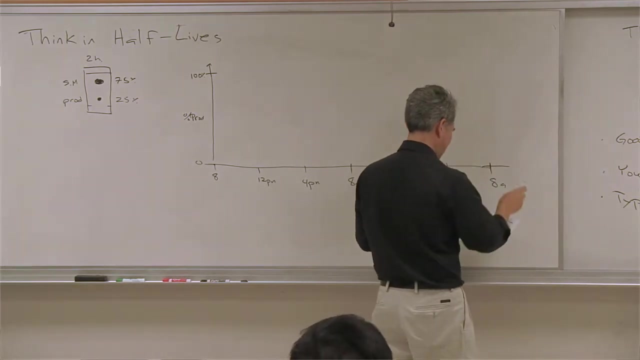 Here's noon today, Here's late afternoon, Here's beer time. Here's you go back to the lab and set up another reaction, You wake up at 4 am to start the new day, and so on and so forth. 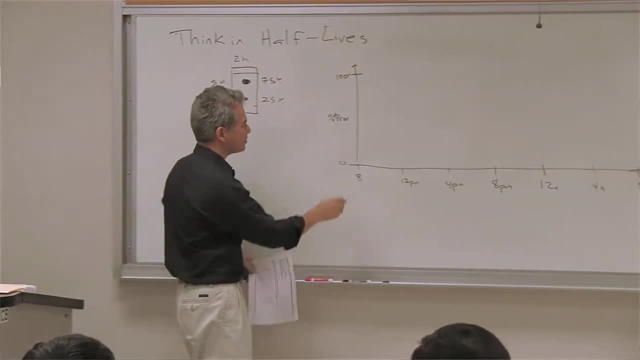 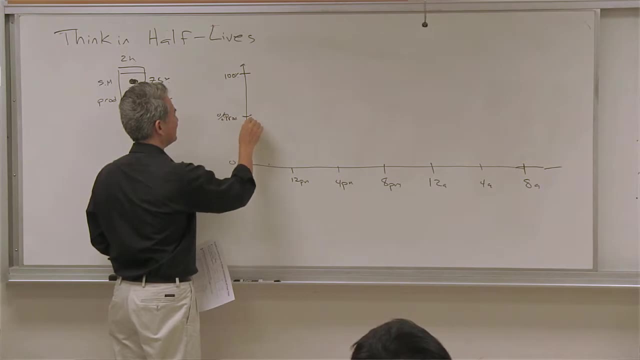 So what is this reaction telling you? So we're here at two hours in. We started it at 8 am this morning and we're two hours in. Let me try to draw up my Here's 50%. I'm not sure if I can fit this in. 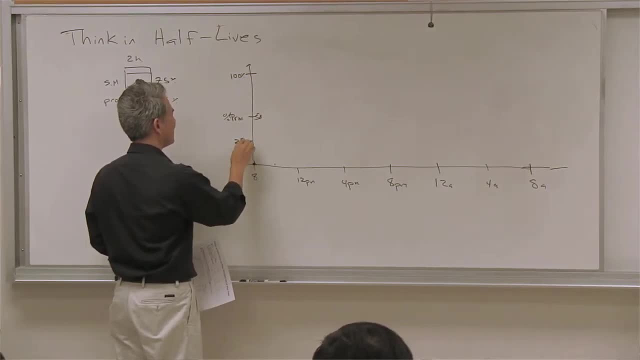 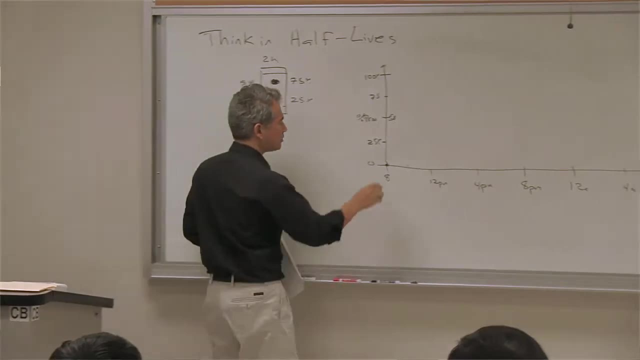 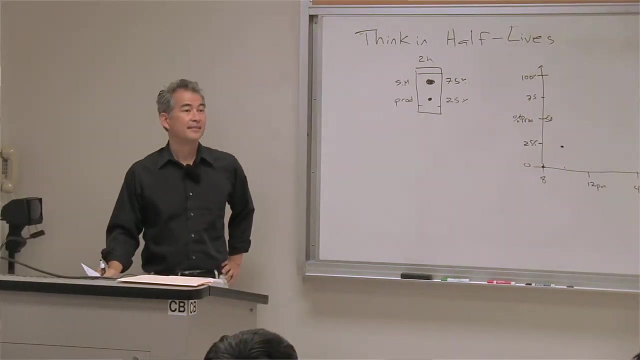 I'll write it right here: There's 50%, Here's 25%, Here's 75%. So we're at two hours in, We're at 25% yield, And the question is, where are you going to be at four hours? 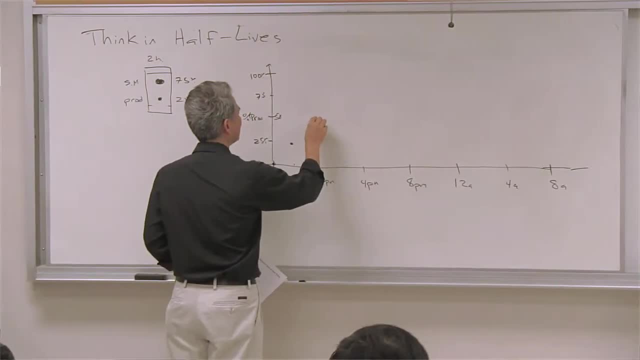 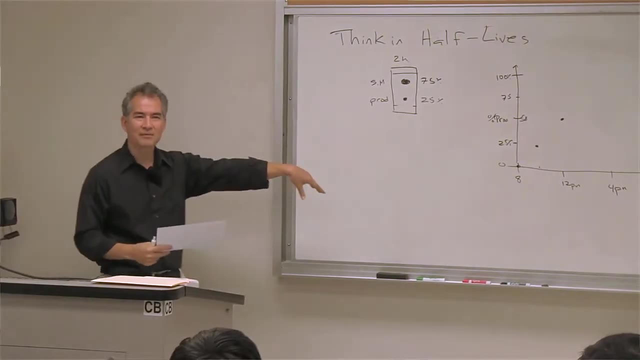 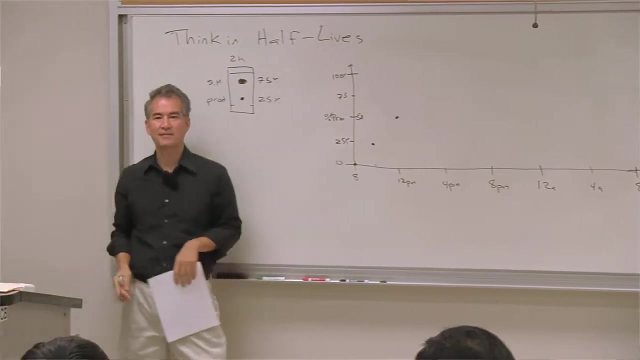 And I'll give you a hint. Typically most reactions are approximately linear for the first half-life- approximately Most reactions. I'm not talking about the other 3% of the reactions that don't follow this simple rule, But generally most reactions show an about-linear progress curve for the first half-life. 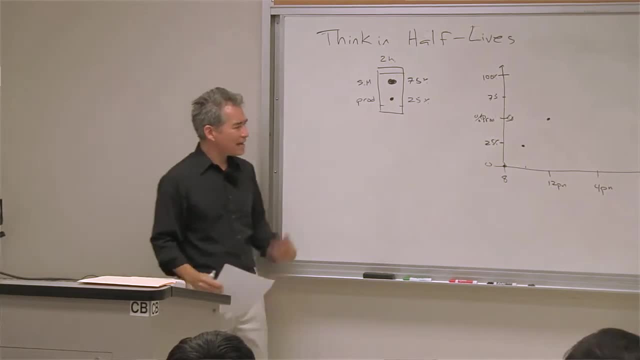 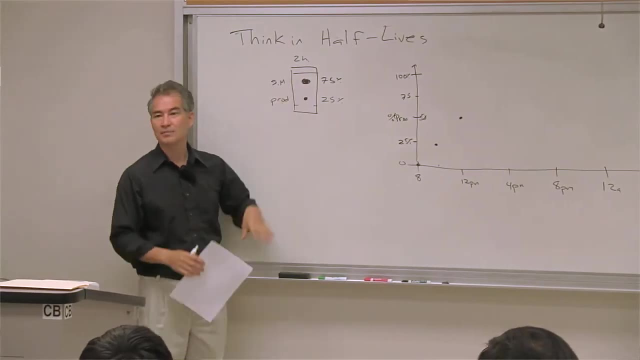 Half-life means half-done, So I could confidently predict that after four hours my reaction is going to be half-done, if this is indeed changing and growing bigger, and that's growing smaller. Just by looking at one TLC I can plan out what's going to happen. 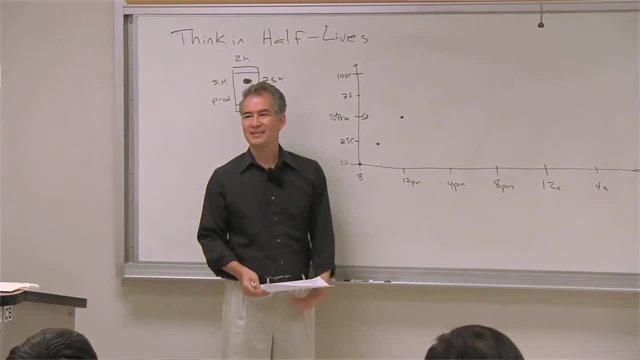 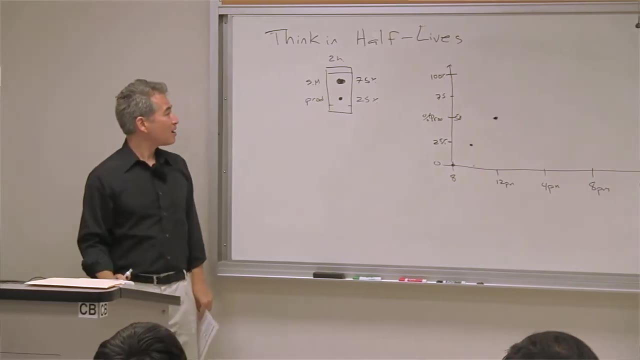 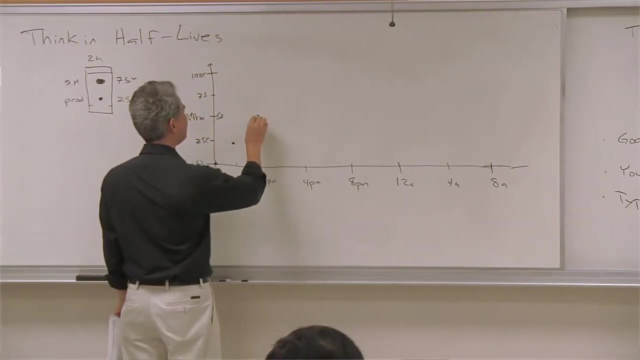 But the real question is: when is my reaction going to be complete? So if this is one half-life, if four hours is one half-life, how much product am I going to have after another four hours? So we've got 50% done after another four hours. 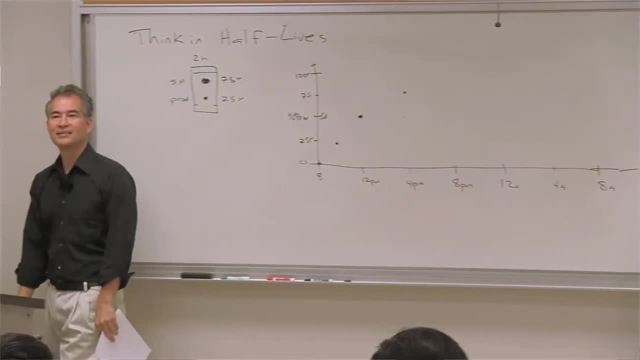 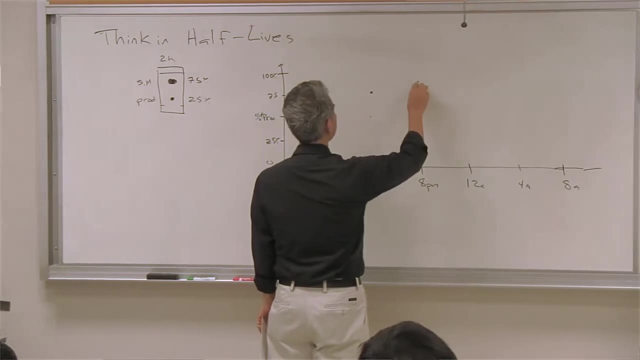 Another half will go. Now I'm at 75% yield. I've got 25% starting material left. Now half of that's going to react over the next four hours. So now we're at 87.5%. I don't know if I'm plotting this that correctly. All right- I don't know if I'm plotting this that correctly- I wait another four hours. Now we're at 92% or something like that, and so on and so forth. Generally, the rule here is that it takes about eight half-lives for you to reach completion. And so that number corresponds to greater than 99%, 99.9%, completion: Eight half-lives, Eight half-lives. In other words, if one half-life is four hours, we've got 32 hours to wait before this reaction. 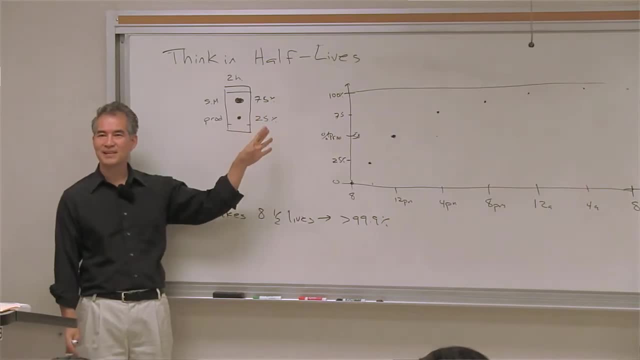 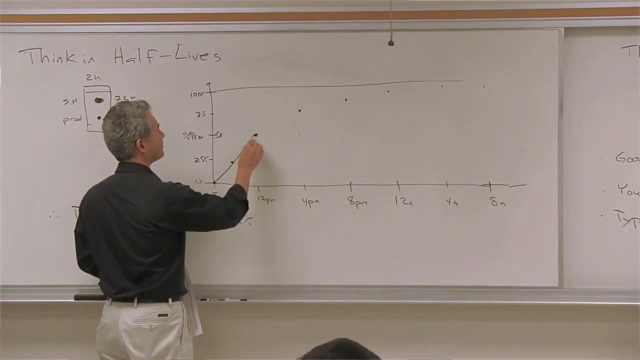 is complete right. Just by looking at our first TLC we could have guessed that. And the problem is that your tendency is to think linear, right. Your tendency is to extrapolate this linearity of the first half-life to think: oh, my reaction's. 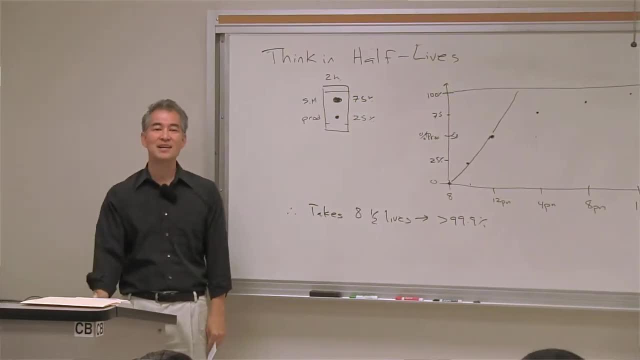 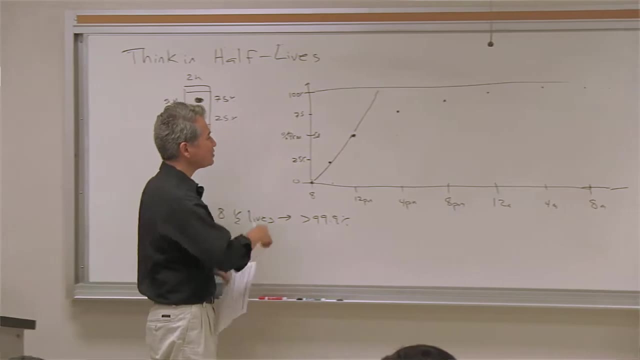 going to be done at four. Let me get everything ready to work on my. You're wasting your time. You're misbudgeting your time in the lab. if you're thinking linearly, Very few reactions. And why is it true that reactions typically follow this kind of time progression curve? 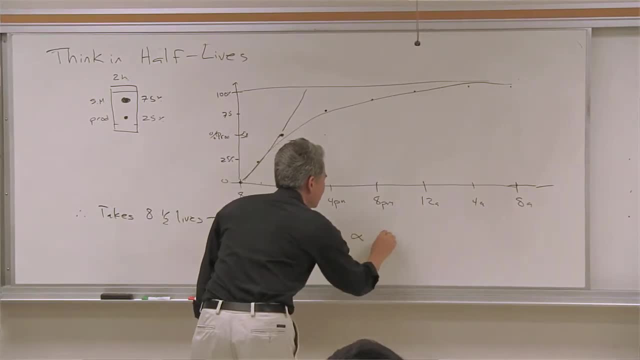 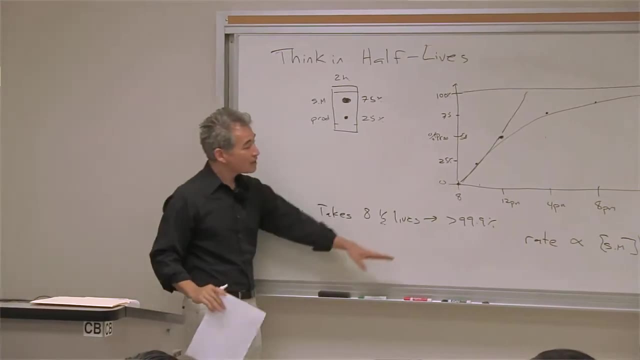 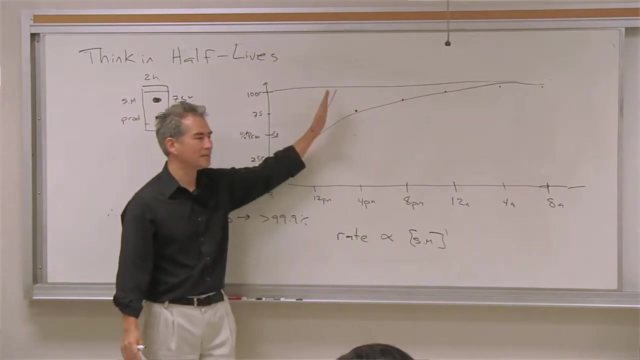 And the reason is that most reactions- not all- are first-order. in starting material. There's a first-order concentration dependence And as the amount of starting material decreases, the rate of your reaction will decrease. There are some reactions that have a zeroth-order dependence and are totally 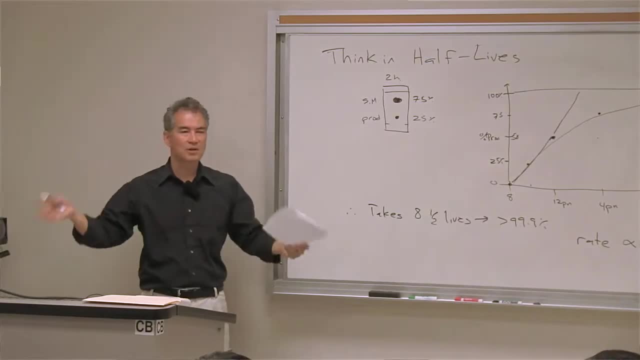 That's not common. There's some catalytic reactions where you're waiting for the ligand to fall off. There's some catalytic reactions where you're waiting for the ligand to fall off. There's some catalytic reactions where you're waiting for the ligand to fall off the metal. 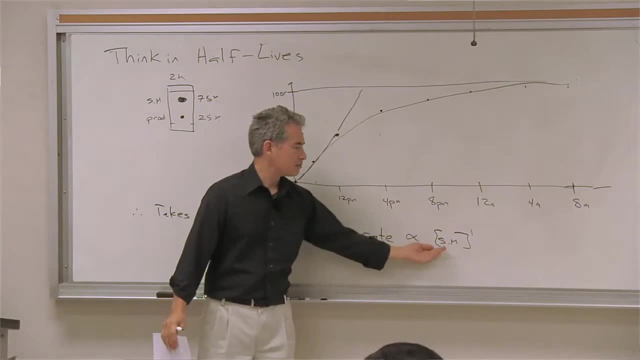 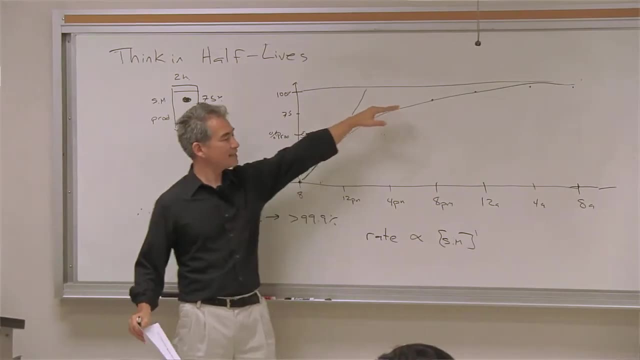 or something like that. Most reactions follow this type of a rate dependence on starting material concentration, So you'll have a tendency to think like this. But as soon as you start thinking like this, you can make use of your time. You got another 32 hours for your reaction to be done. 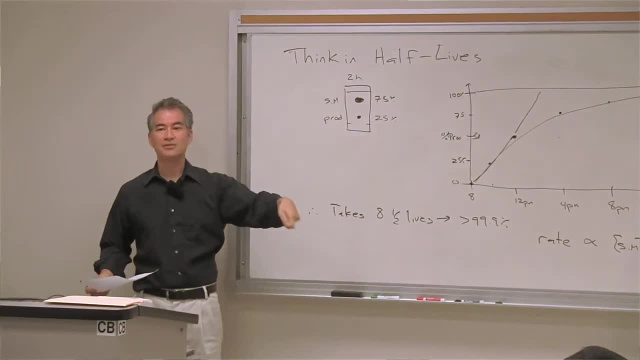 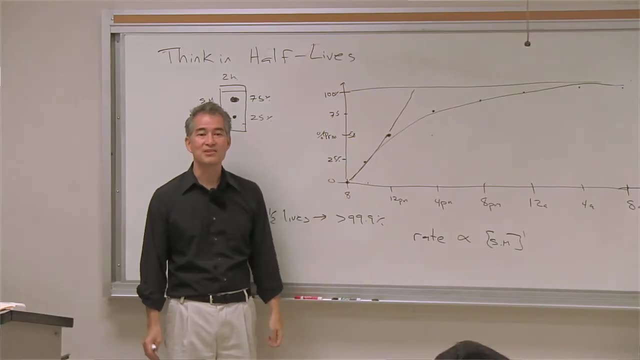 Set up another reaction. Or if you're not happy with that heat it, Do something. Add more reagent, Make it 10 times faster. It's not like just because it was written in some procedure. you have to follow the procedure. 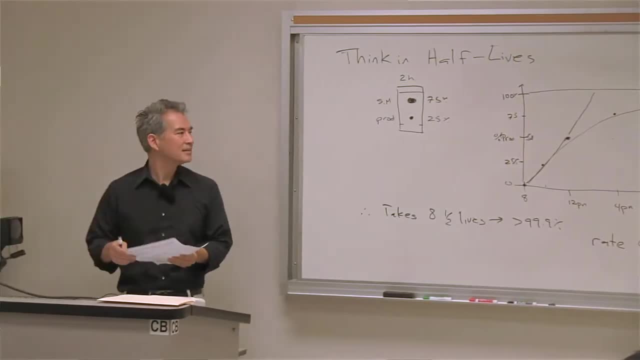 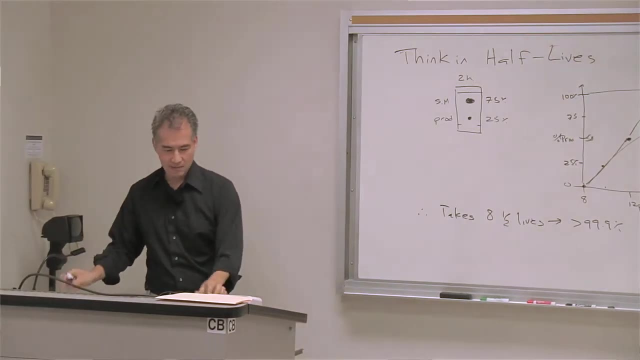 You can use a. You can use a basic understanding of concentration and temperature and time to make your reactions do whatever you want, And so we encourage you to do that here at UCI and everywhere else. Okay, So let's take a look at. 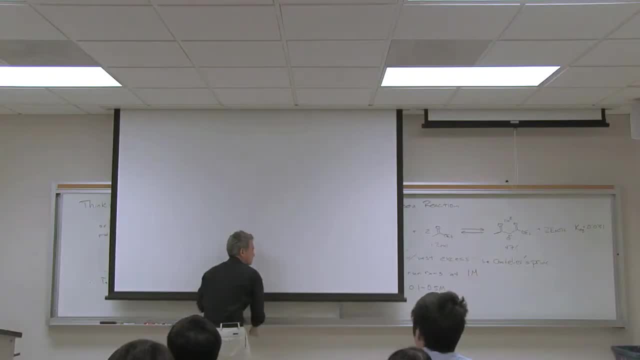 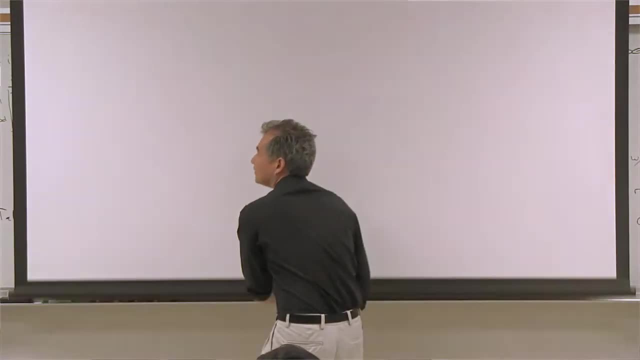 We've talked a lot about rate constants in this class And I want to put some numbers on those rate constants and get you to stop thinking about rate constants Because, like I said, you don't When you're in the lab, you're not thinking about rate constants. 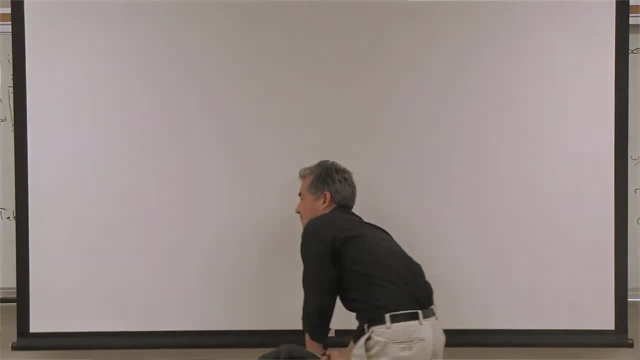 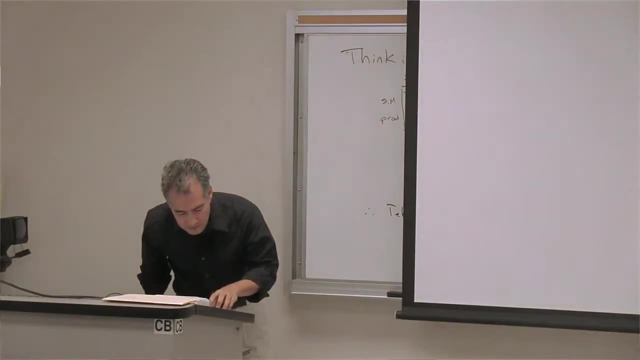 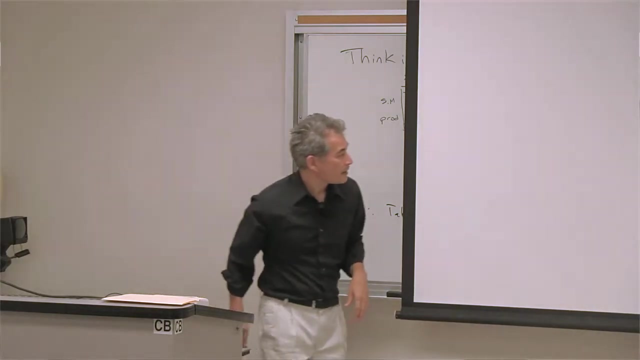 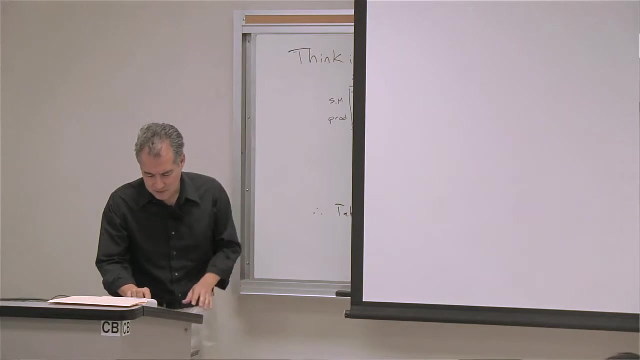 You're thinking about screens that don't go down. Okay, Let me. I hope this thing is going to turn on in a moment here. I'm just going to bring up a slide from the notes that I posted online, because I can't reproduce this chart here. 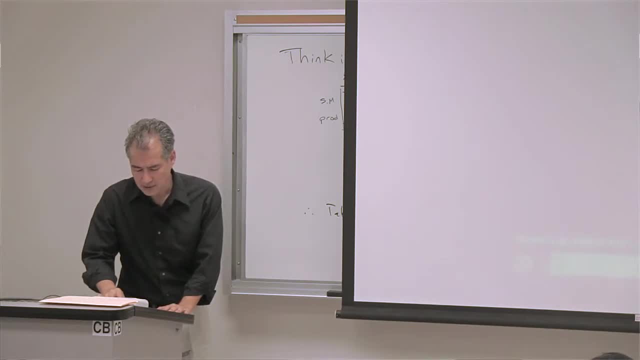 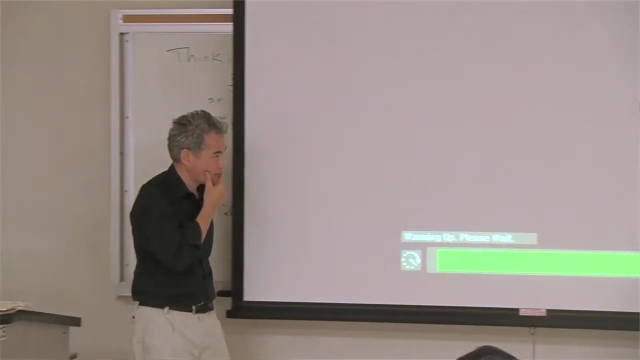 And the projector's warming up. for a second, I just want to look at a A table that relates- That relates rate constants- to half-lives. That's promising. There we go. So when you think about reactions that you run in the laboratory- and specifically I'm 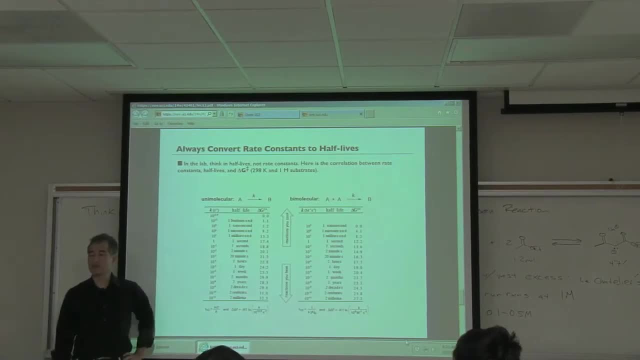 giving you examples of elementary reactions. let's suppose you know something about the rate constant for a reaction. There's a simple equation. I'm sorry I wrote it so small here If you can't see this. If you're thinking about a unimolecular process, your rate determining step is some unimolecular. 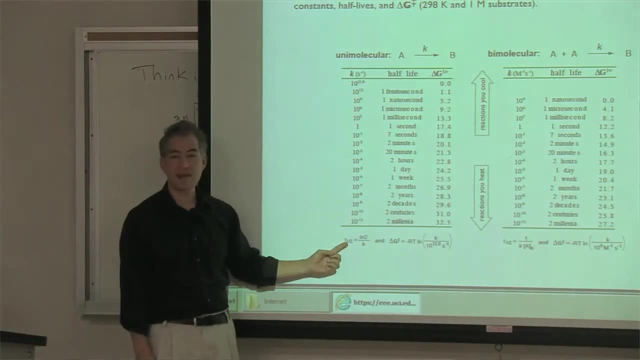 process. for example, there's a simple relationship between half-life and rate constant, And that is that the half-life is equal to natural log of two divided by the rate constant. So bigger rate constant means shorter half-life. Now I'm too stupid to know what natural log of two is, so I always use one. 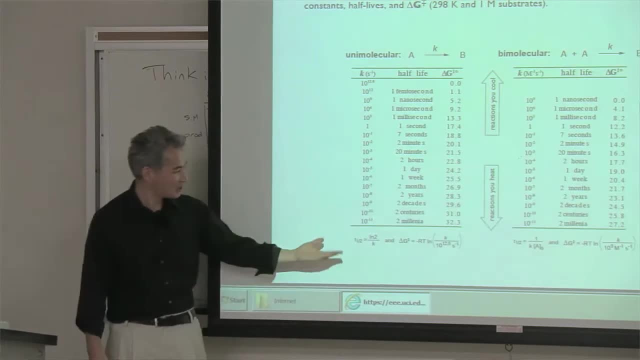 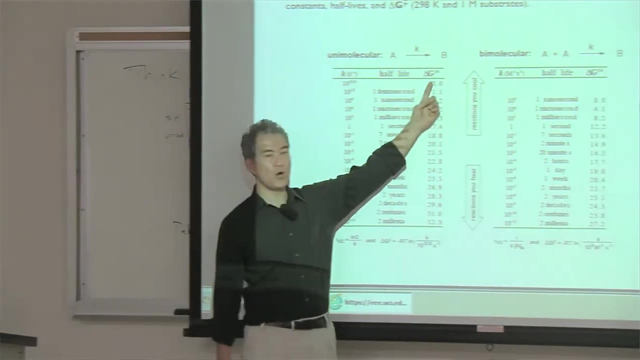 And it's never failed me right. Natural log of two is close enough to one where half-life is approximately the inverse of the rate constant. So if you take, for example, a reaction that has no barrier, that's the fastest possible reaction for a unimolecular reaction, a no-barrier reaction. 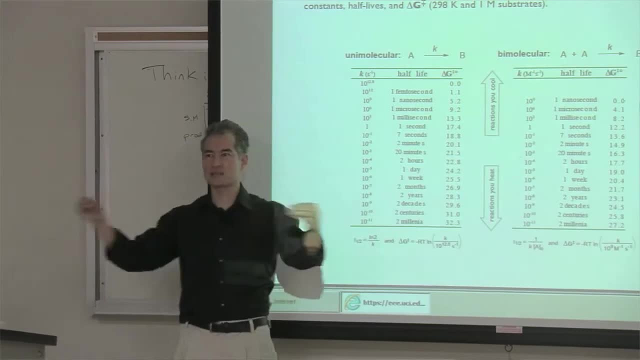 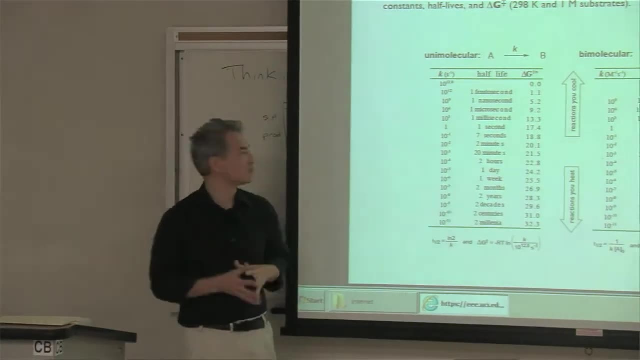 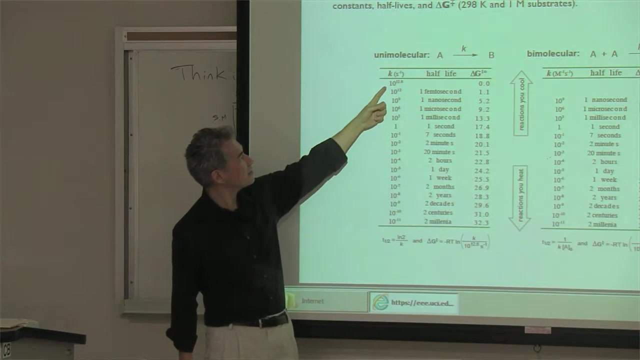 And we said that what determines the maximum rate is the rate of vibration. That's about 12.8, 10 to the 12.8 times a second. your reaction's creating product. This is the typical range of rate constants. It's for unimolecular processes that we talked about. 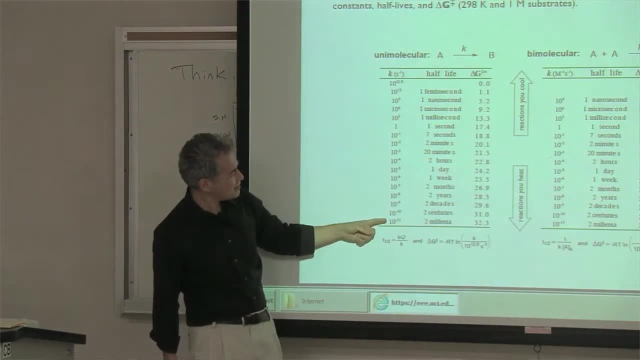 At the upper end is a bond vibration And at the lower end is kind of random. here It's just determined by how long you're willing to wait, right, You're not willing to wait that long, So these reactions are totally meaningless to you at room temperature. 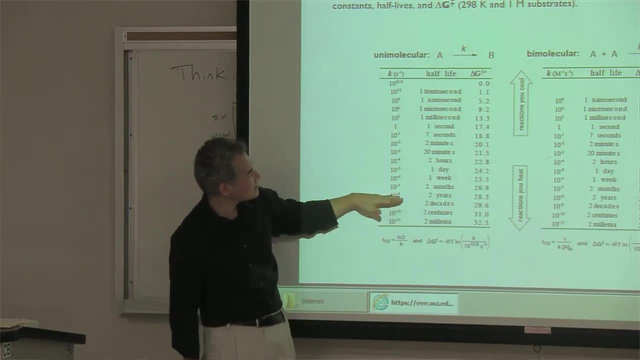 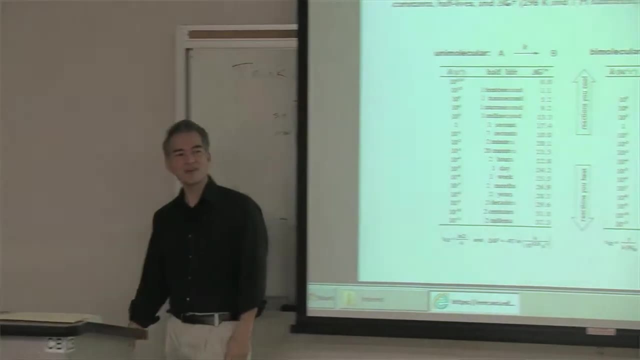 So if you're not happy with reactions that are going to take two months or two years or two decades, heat those reactions. You can heat them. That's how you get over this K. All of these K values And half-lives here are for room temperature. 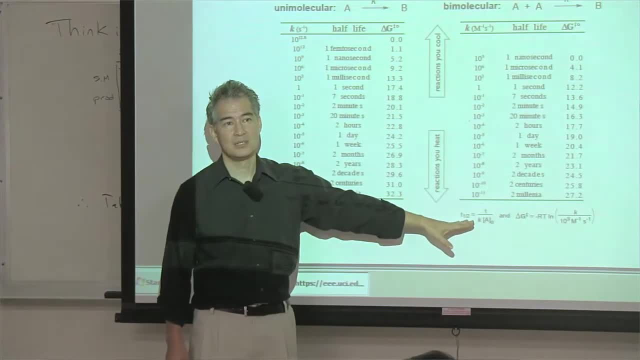 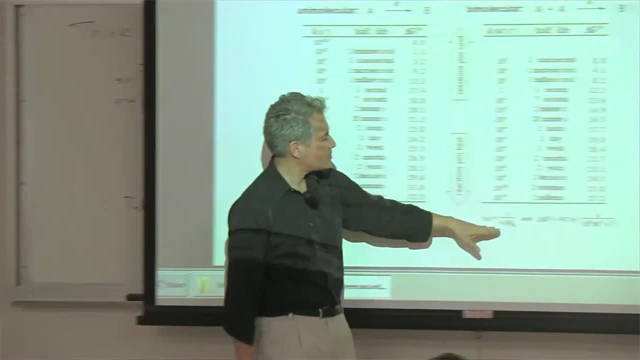 So if you look at bimolecular reactions, the equation is not as simple. Bimolecular reactions: there's a concentration dependence because things have to collide with each other, And so you use something called the integrated rate equation. I usually just extrapolate back to one molar. 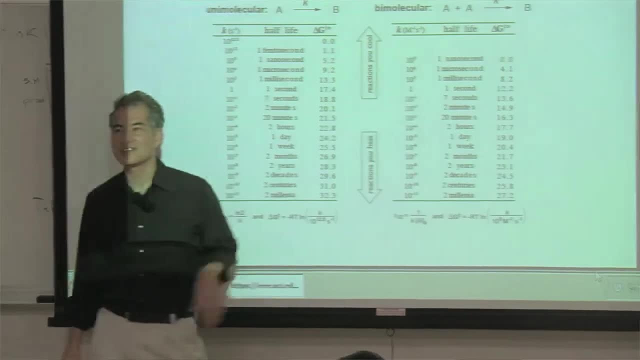 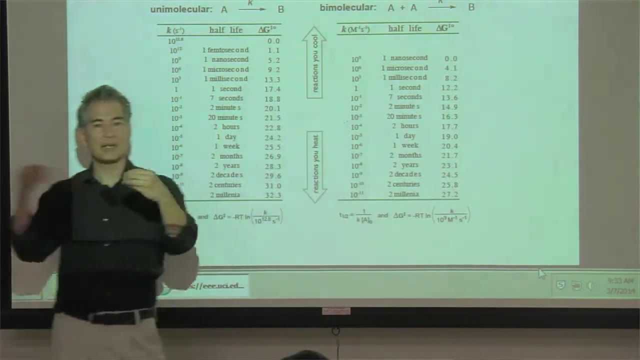 If it is one molar, this becomes one, and it's the same equation that I just gave you before And you can see again. there's this. so what's the maximum rate constant you can have for a bimolecular process? 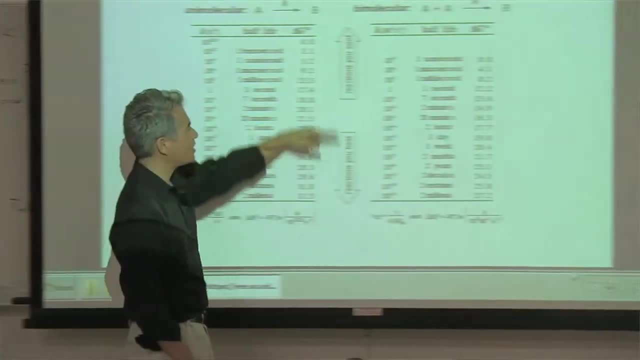 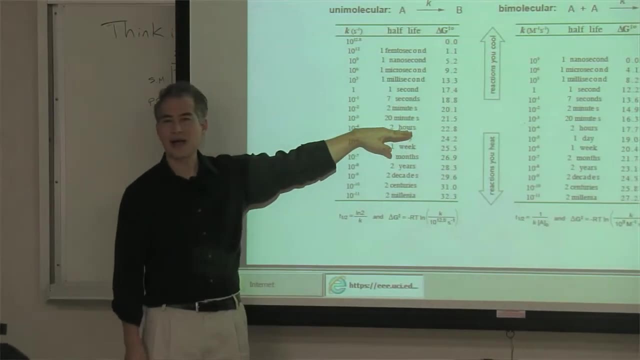 It's limited by diffusion, not by a bond vibration. So you're starting up over here. So let me invite you to just think about one type of number for both of these processes, And that's a two-hour half-life reaction. That's the kinds of reactions you're going to run in the lab. Things that take about two hours. You can have some reactions that you cool. All of these reactions that are faster are so exothermic. you're typically cooling those down, trying to get better selectivity. Any reaction you've ever run that has free energies. 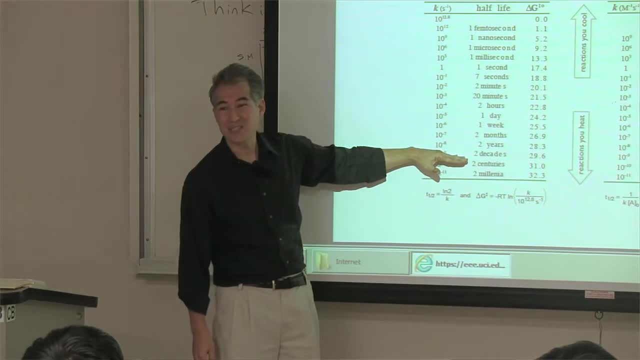 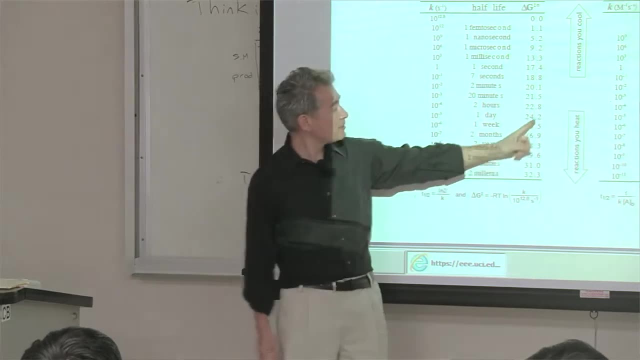 Of activation that are higher than this. You're probably heating those to get them to go faster, because you're not happy waiting two decades for your reactions to complete. Those are reactions you're really heating hot. So all these reactions down here are reactions you heat. 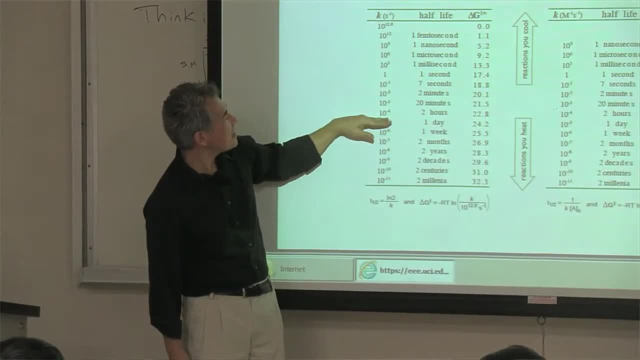 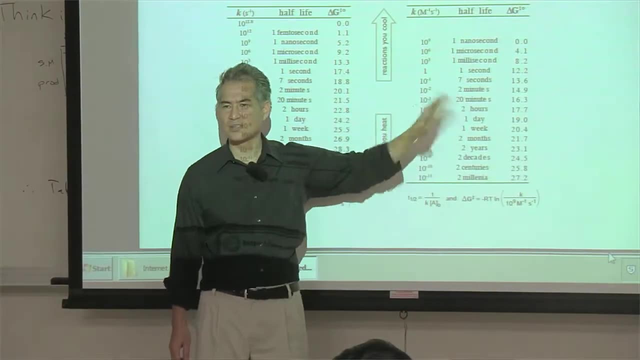 All these reactions up here are reactions you cool, And so try to keep this in mind. Rate constants about 10 to the minus fourth per second or per molar per second: Those are reactions that are that you're running at room temperature in the lab. 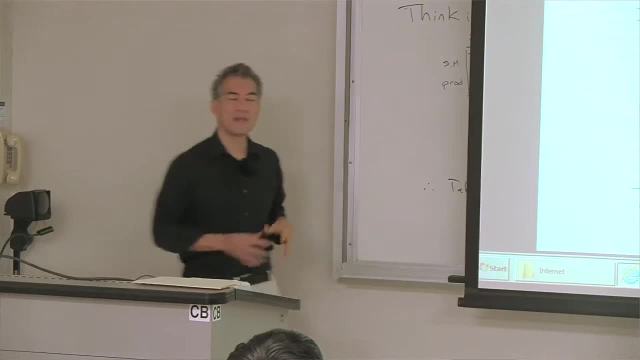 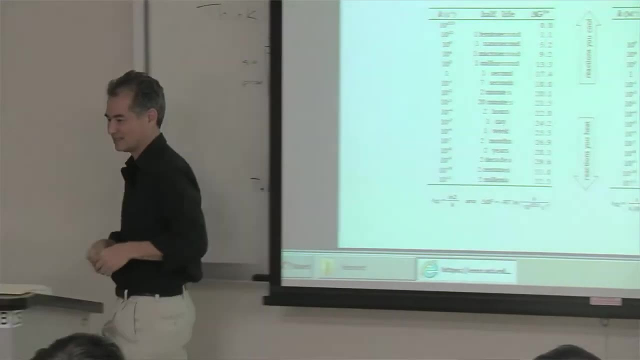 10 to the minus four. Just keep that in mind. Okay, If somebody tells you about their fancy reaction- that is a rate constant of 10 to the minus eight- you're just like: no, That's no good, That's a crummy reaction. 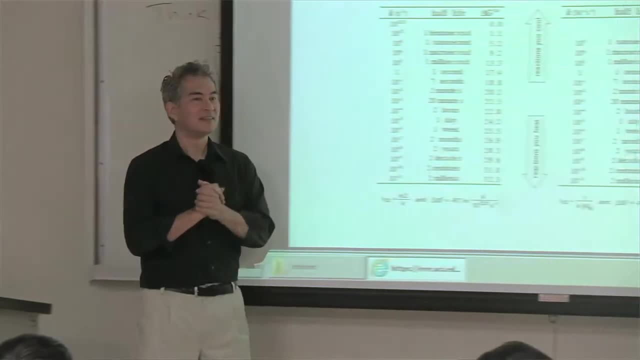 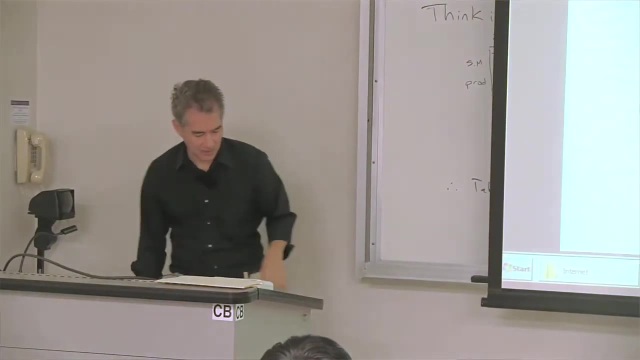 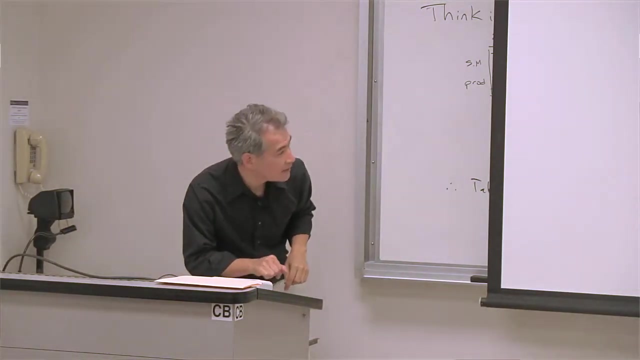 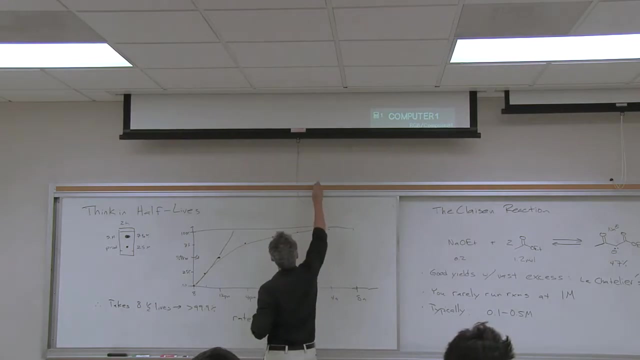 Or if somebody tells you about their rate constant, that's 10 to the plus fifth. that's a fast reaction, That's an impressive reaction. Okay, 10 to the minus four, Good number to keep in mind. Okay, Think in half lives in the lab. 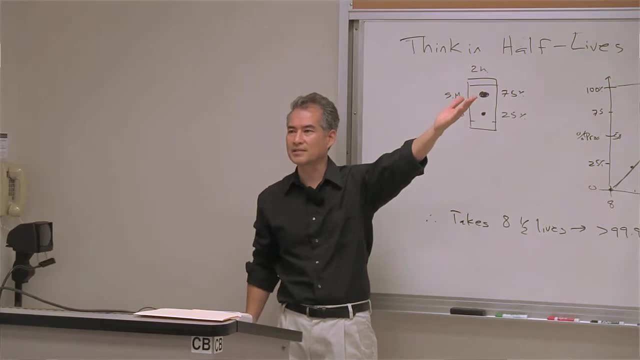 Right, Our clocks. I don't know if we have a clock in here. There's a clock over on the wall on the side here. It's not in per second, It's in minutes, hours, So think in half lives, Just like a clock does. 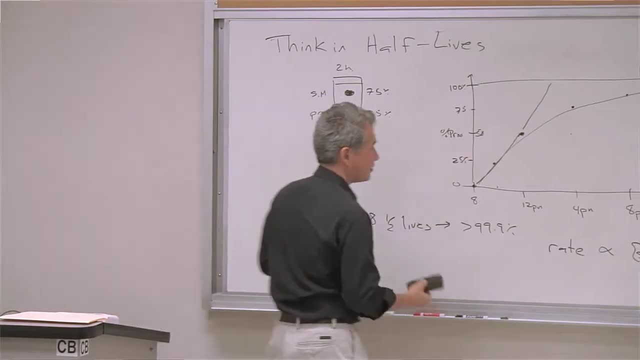 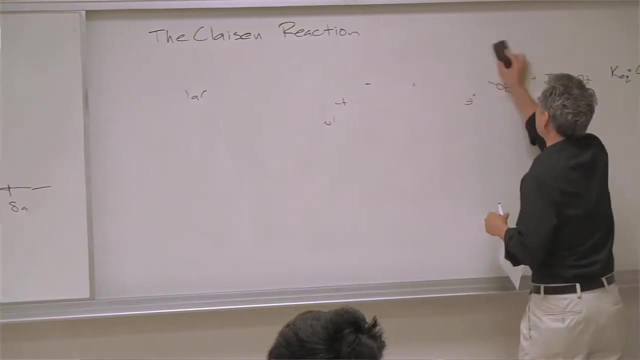 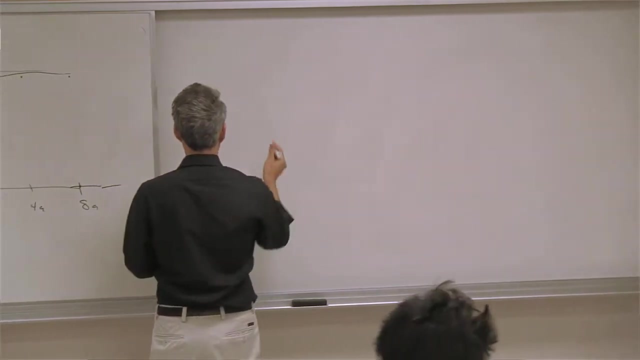 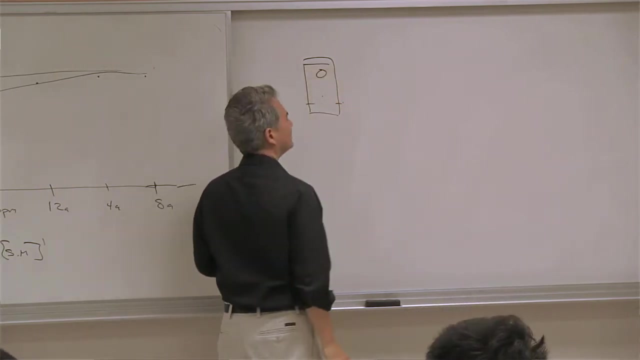 Okay, Let's come back to this other tool that you have to make your reactions work better. Okay, I gave you this very optimistic scenario where after two hours, you had 25% product, but more typically it looks like this: Starting materials on top, and you're like now, what do I do? 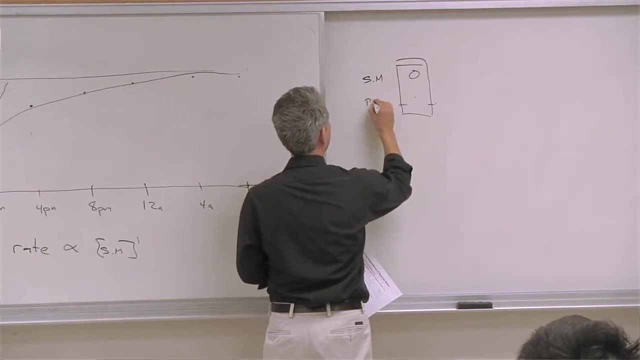 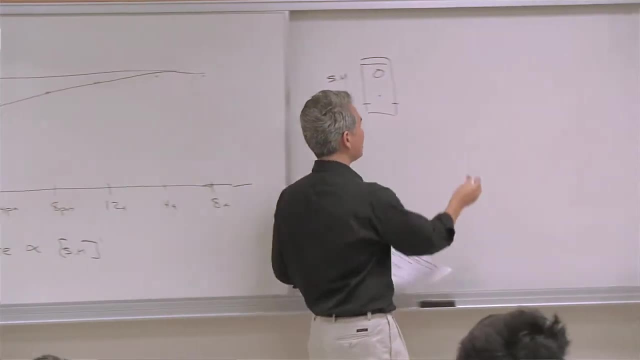 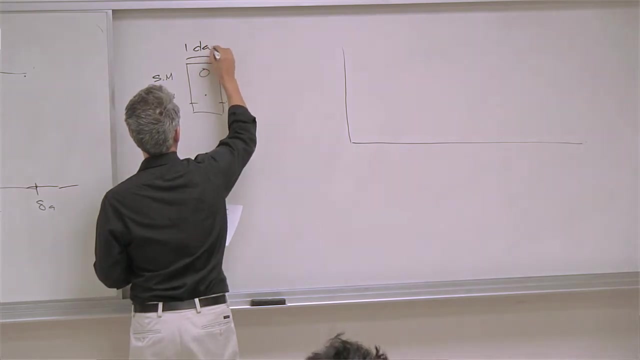 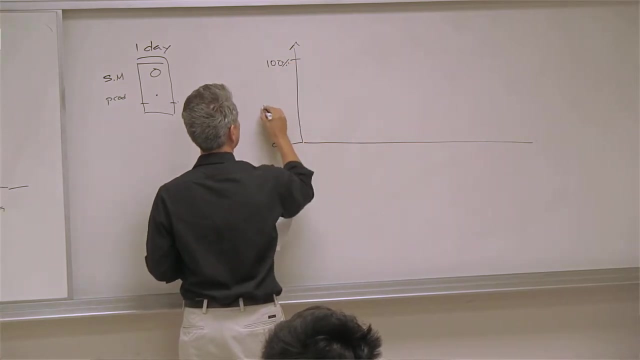 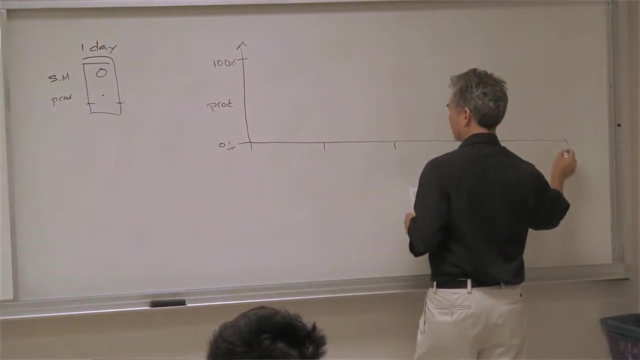 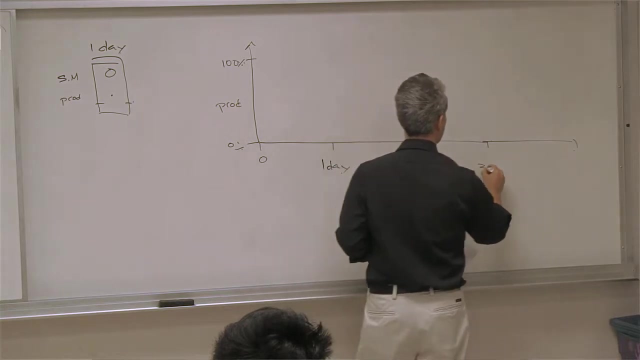 What does that mean when your starting material looks like this and your product is down here, some teeny- and I'm this is optimistic, because usually there's side products that are coming in faster. And let me trace out this reaction: progress curve For a reaction that looks like this. let's suppose this is one day, and so you can. 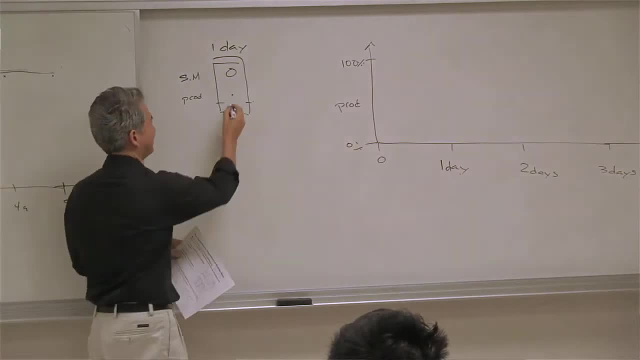 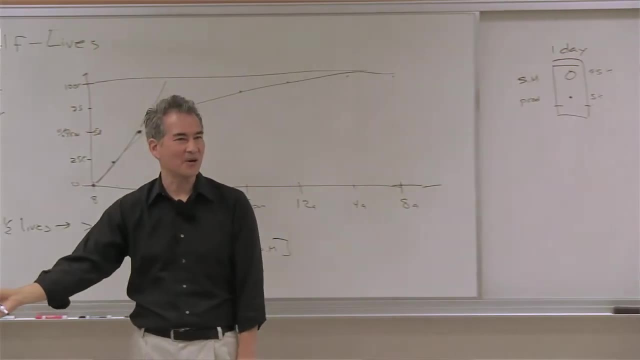 see what's happening here. I I don't know what kind of number I'm. let's suppose this is 5% versus 95.. Does it really matter whether it's 10 to 90 or 95,, 90,, no? 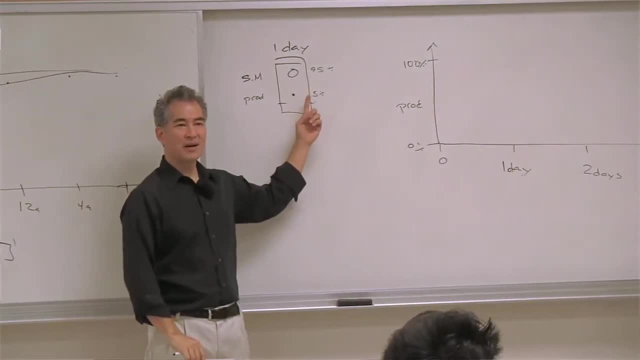 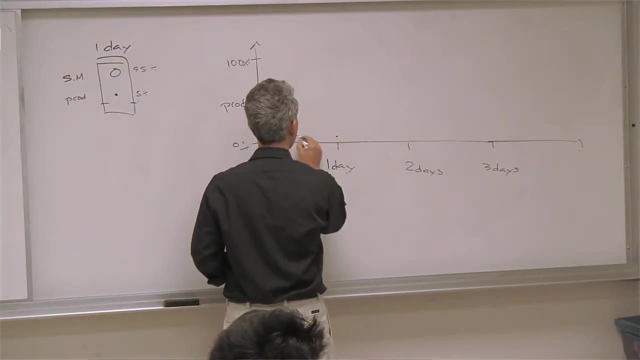 You can tell what's going to happen If you've been waiting a day to get to here. where are you on this progress curve? Remember, the progress curves get slower and slower and slower. If you're at 10% after one day, look how long it's going to take you to get to one half. 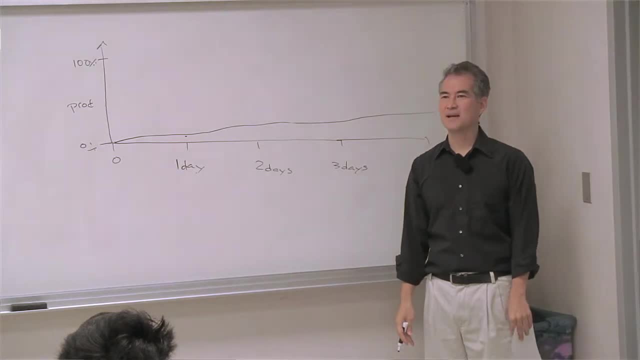 life, Days and days, and days and days, to get to one half life. And so what are you going to do? What are you going to do in the lab? Right, You're. it's not going to do you any good to keep TLCing this reaction. 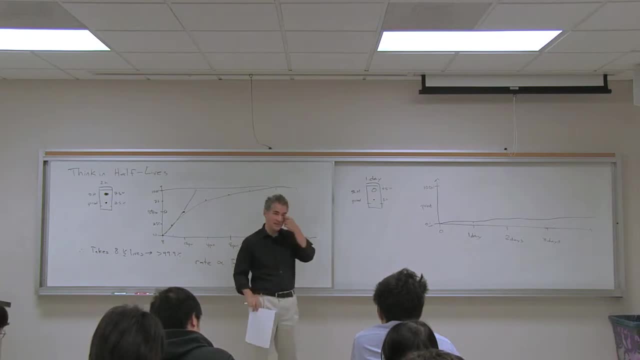 I mean as long as you can see that it's growing in and the reaction hasn't stopped. I didn't mean to have this curvy line that was supposed to be a kind of nice even curve there, Right, TLCing. it isn't going to help you. 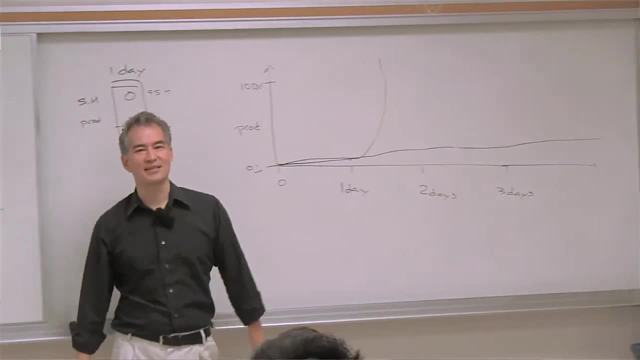 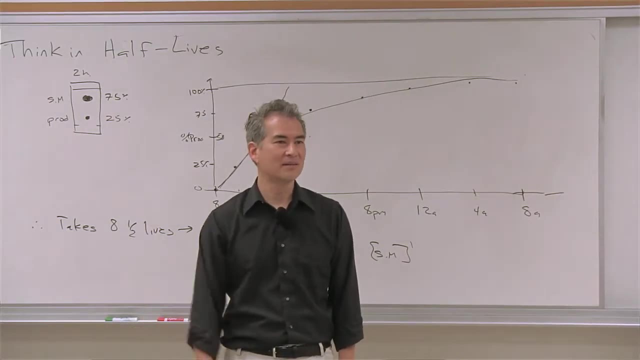 I promise you your reaction is not going to do this right. No reaction does that- Soluble reactions. don't just suddenly decide that they're going to amp up and give you 100%. Your wishful thinking will not help you. It's not going to help you. 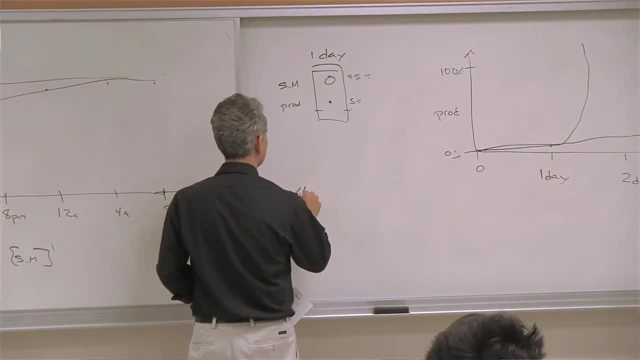 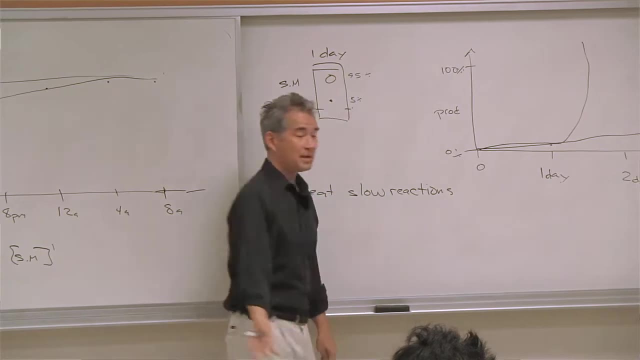 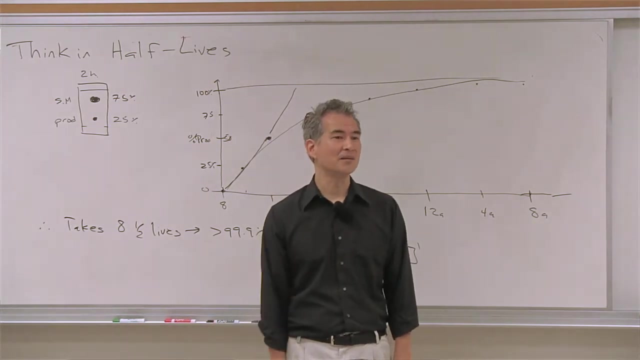 So you need to take control, And let me just suggest one thing: You may choose to just throw it away. It's not going anywhere Too slow. Before you throw it away, heat it up. It could all decompose to junk, but you were just going to throw it away anyways. 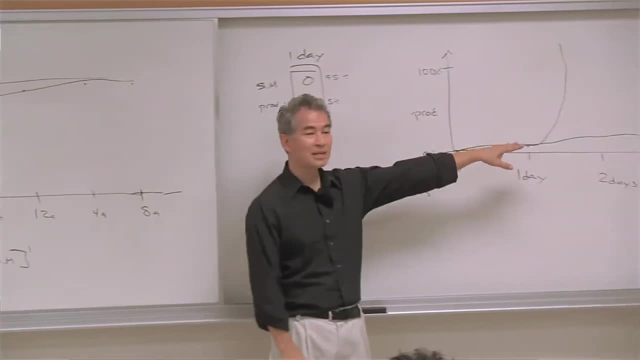 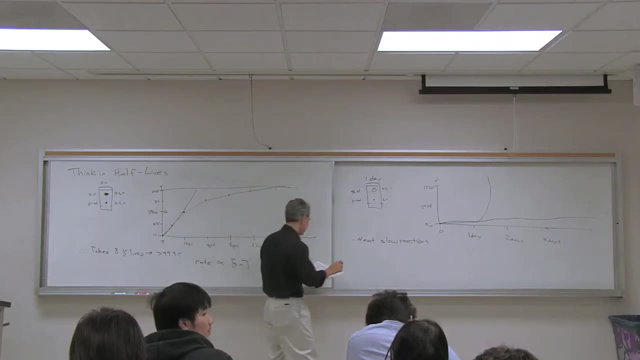 So why don't you heat it up before you throw it away? You might actually be able to push it to completion faster. You change the rate constant when you heat things. That's the effect of temperature, Because it makes reactions go faster, And I'll give you a simple rule of thumb that actually works pretty well. 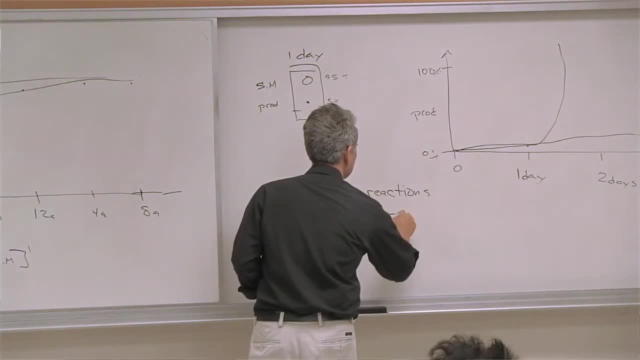 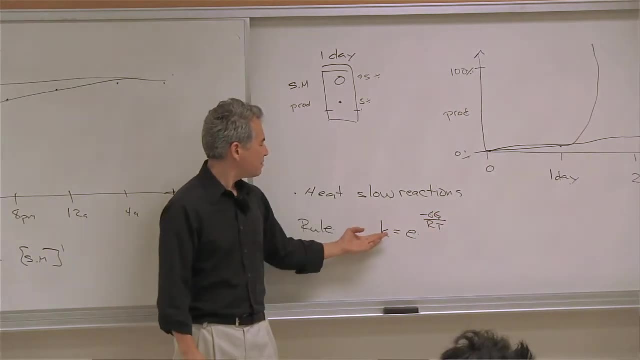 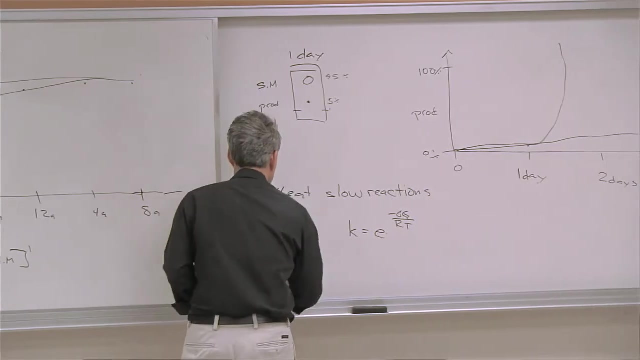 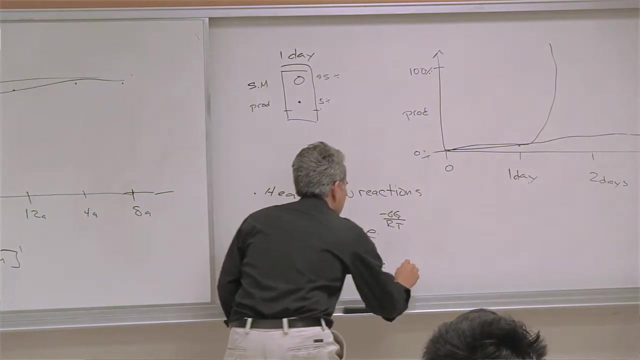 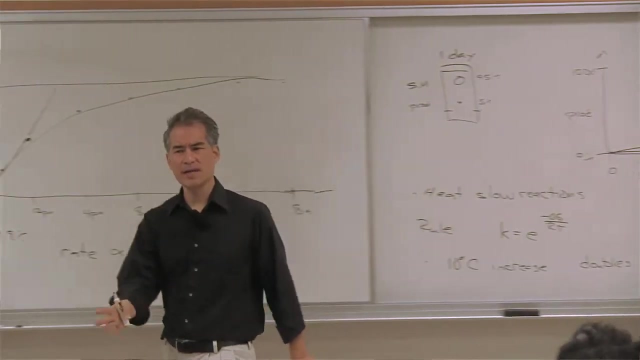 And let me just remind you why it works well. Right, Reactions obey this simple dependence of rate constant on temperature. And so if you heat reactions because of this equation, Amp about every 10 degree increase and you can plug the numbers in yourself to see what happens. 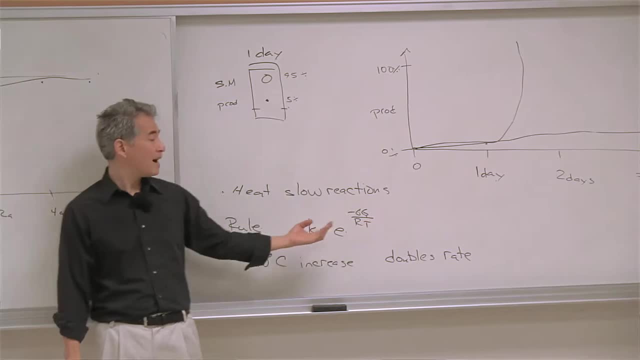 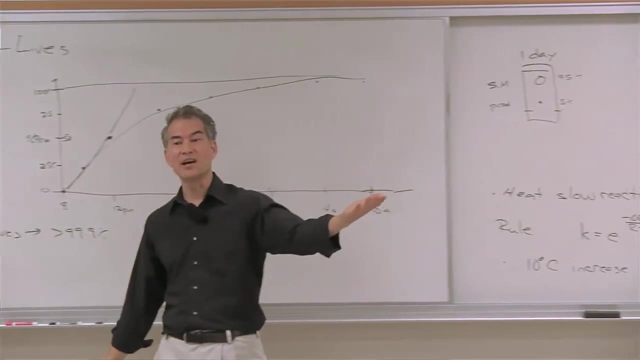 if you compare 300 Kelvin with 310 Kelvin, What you'll find is that each 10 degree increase- you know I'm talking about around room temperature not going from 700 Kelvin to 710.. In the typical temperature ranges you're interested in- a 10 degree increase in temperature will. approximately double the rate of your reaction, and so you can use that. So if you change the temperature from 20 degrees to 60 degrees, that's 2 to the 4th right, That 40 degree increase. So each 10 degree change in reaction temperature will approximately double the rate of your. 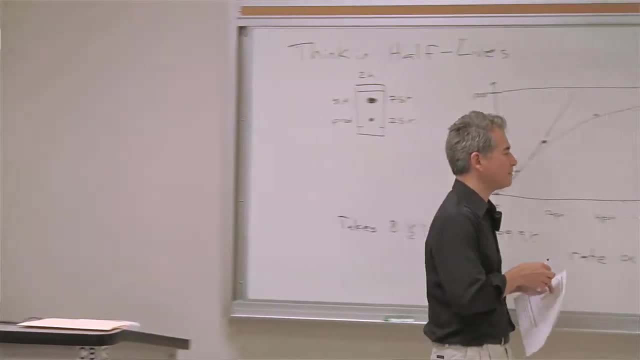 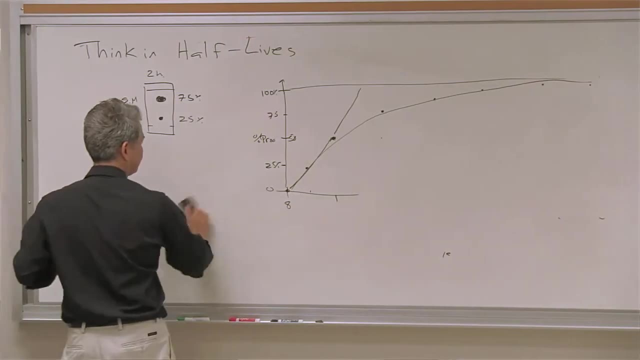 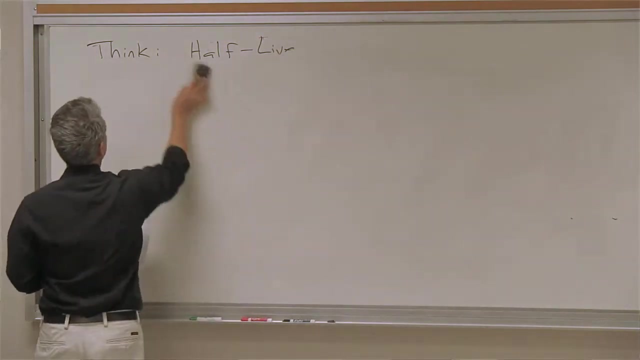 reactions, And so you can use that to force your reactions to finish faster or to estimate what's going to happen when you cool things down. That's a very good estimate for most of the reactions that you run in the lab. OK, I've got one last thing to talk about. that's very practical. 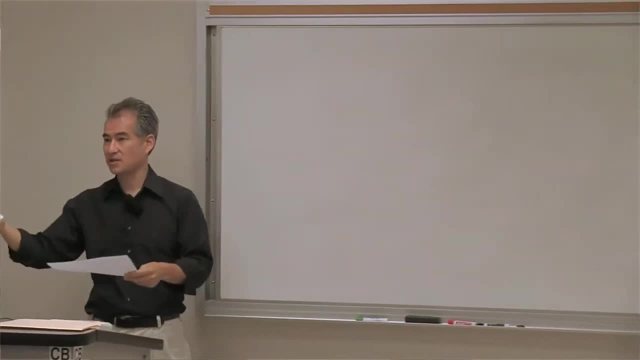 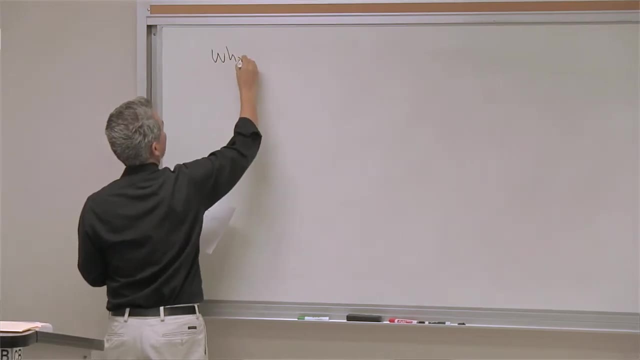 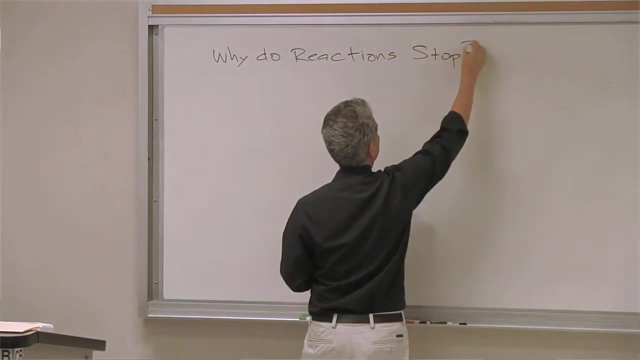 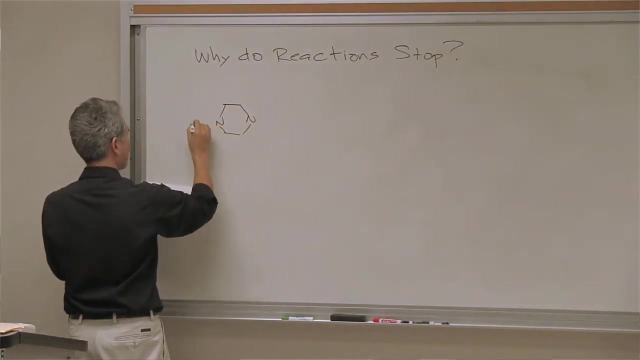 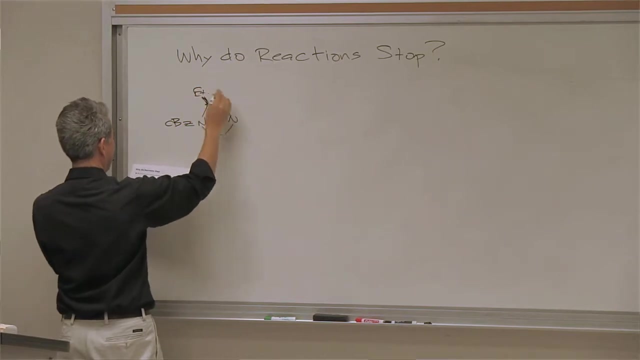 I'm now really trying to tell you about stuff that's practical for how to make yourself more productive in the laboratory. OK, OK, OK, Great, Great. this issue of why reactions stop- The structure of this is totally inconsequential. I'm just 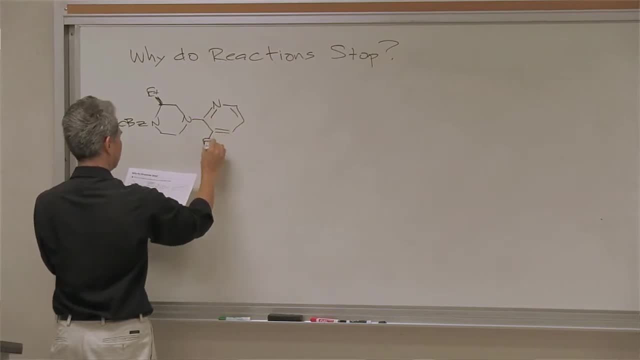 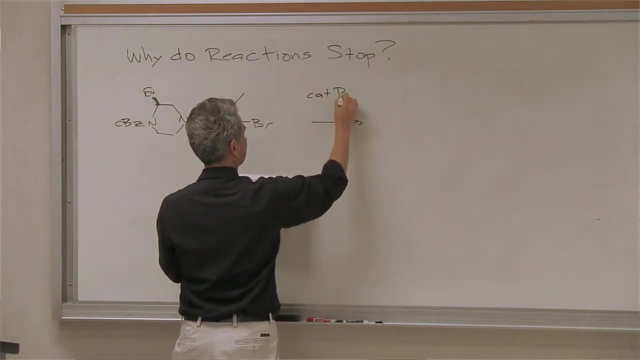 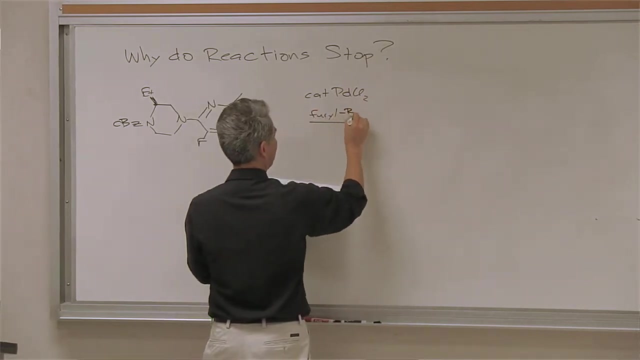 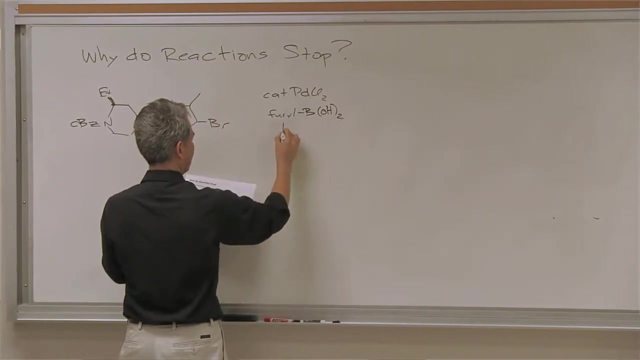 kind of picking out one example. So this is a Suzuki coupling reaction where they're coupling some fural boronic acid. I don't have room here above the arrow, let me make a little space. And you always have some nucleophile in the. 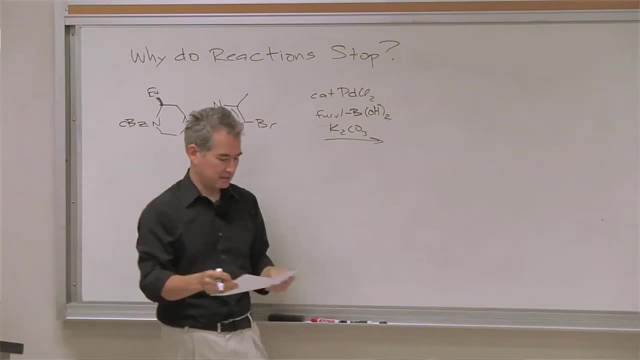 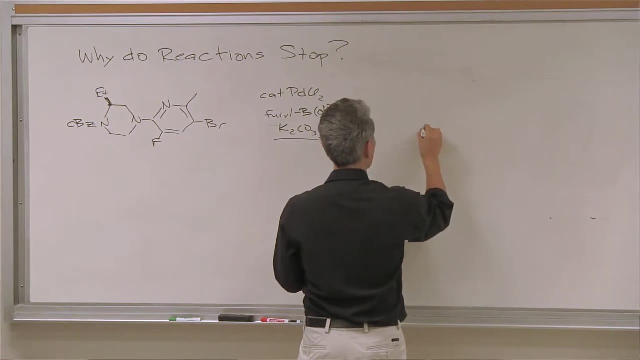 in Suzuki couplings that can attack the boron to make a boronate. So the idea here is that you want to do a cross coupling with the boronic acid. I'm not going to draw the whole structure of the product, I'll just draw this new arrow system that you generate to make a new carbon-carbon. 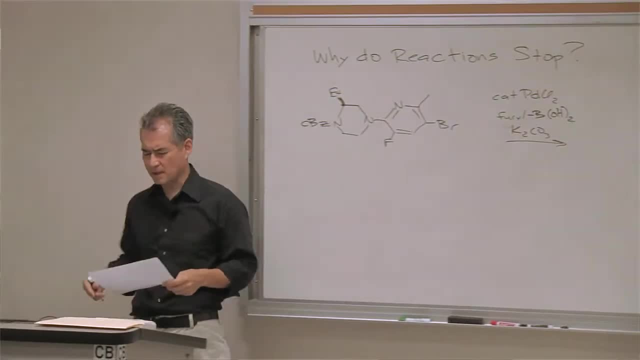 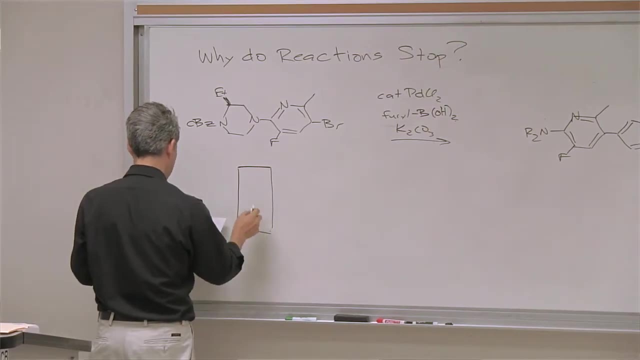 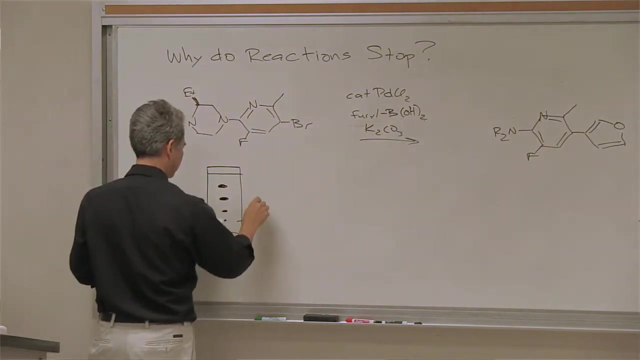 bond. So that's a Suzuki coupling. you make a carbon-carbon bond. Let's suppose you run the reaction and here's what it looks like after two hours. Let me just write boronic acid here, or aryl boronic acid. Here's what it looks like after. 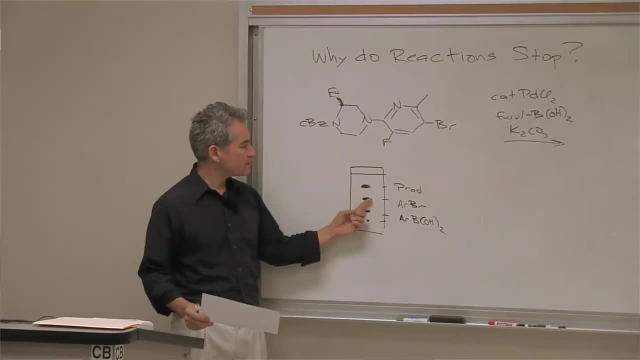 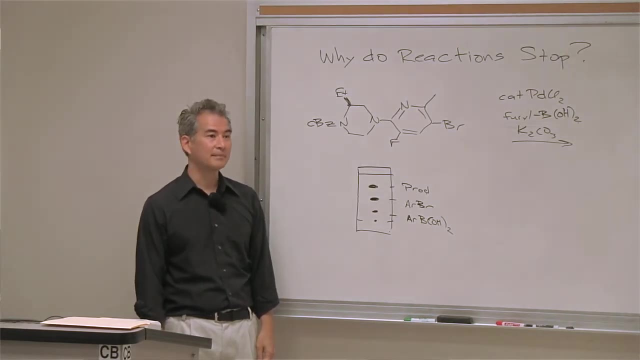 two hours, which is promising, right, There's the product forming, there's my starting material. That's two hours. But then let's suppose you come back after another two hours and it looks the same. And then you come back after another two hours and it's still the same. 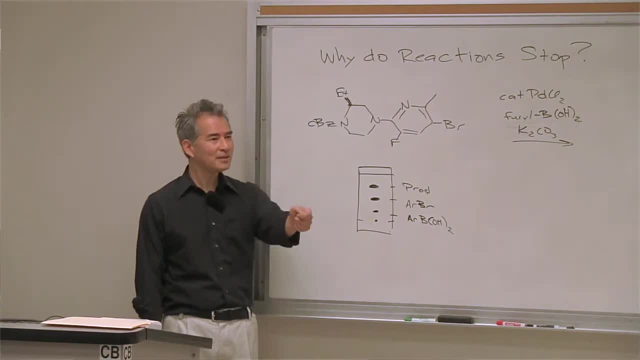 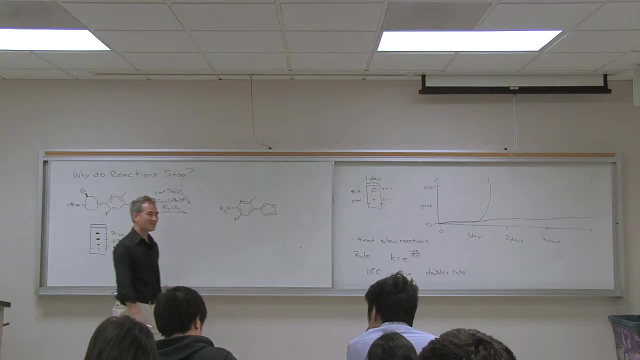 Okay, Okay, It still looks the same. What do you think it's going to look like if you wait another two hours? It's going to look the same. Of course it's going to look the same, Right? And so the question is: why did it stop, Right? If you're, you could work it up and take a. 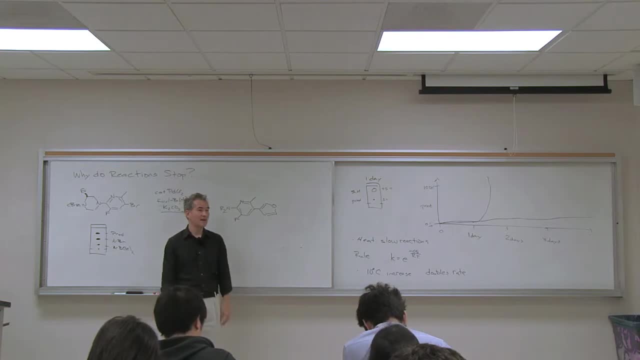 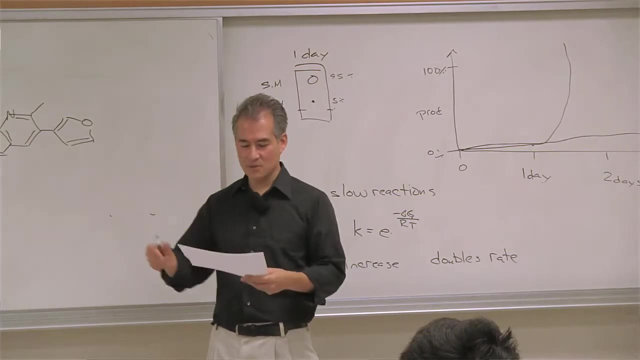 50% yield on this reaction. right, You've already got 50% product. Or you could try to ask yourself: why did my reaction stop? Before I work this reaction up, what can I do to increase the yield? So let's talk about why reactions stop. 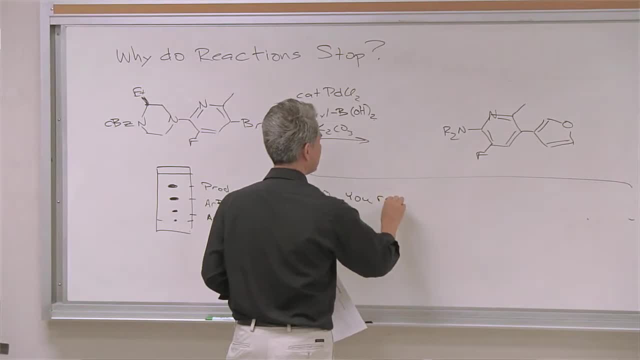 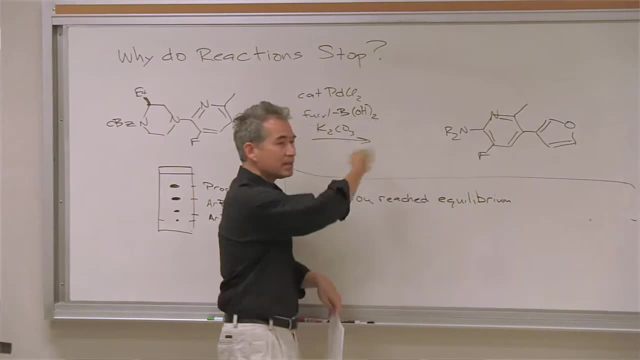 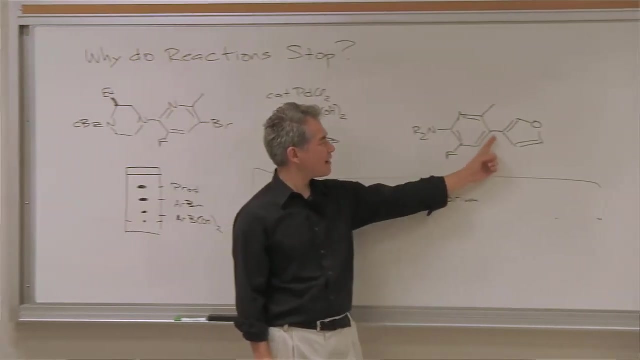 Okay, One possibility is: you reached equilibrium, Right? Maybe this is an equilibrium reaction and the equilibrium constant is one to one. Is that realistic? Is it realistic that bromide came back in and cleaved this off to regenerate? No, that's not realistic, Right? This is a 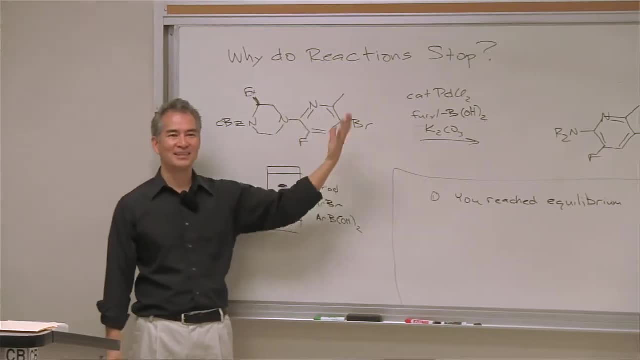 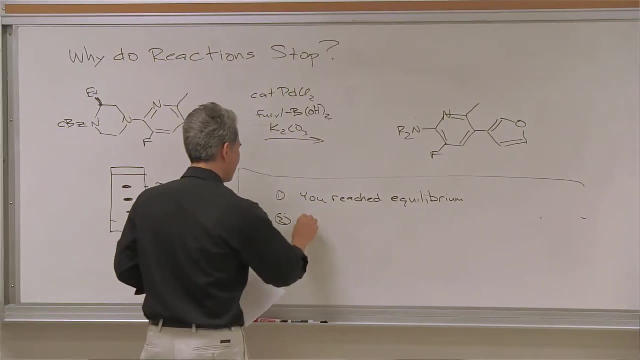 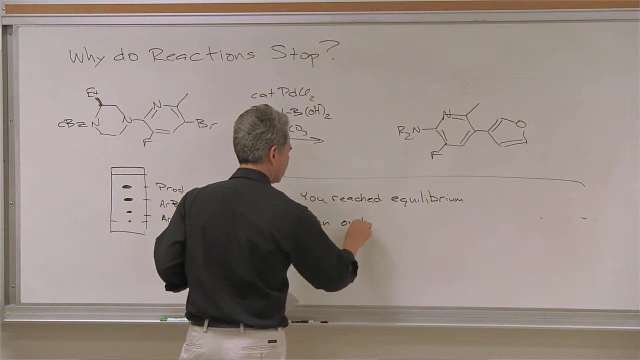 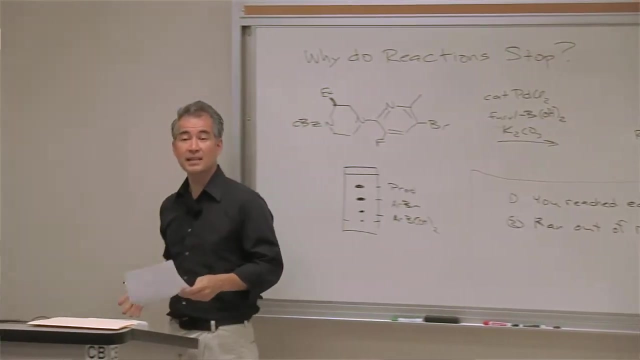 thermodynamically favorable reaction. It's not reversible. It's not like we reach it, That's very rarely. what's controlling your reactions or limiting your yields? Here's another possibility, and this is far more likely. The far more likely possibility is you ran out of reagents Right. Once you run out of reagents, it's over. You're not. 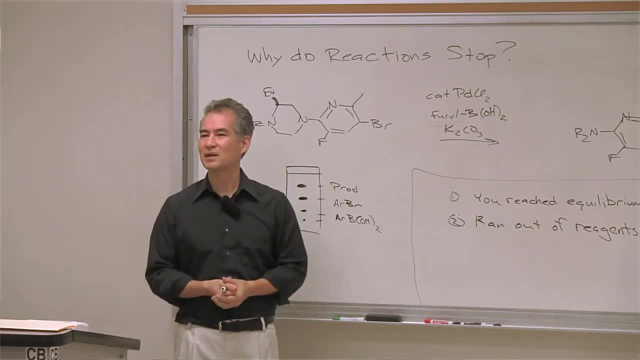 going to form any more product. It's so obvious, Of course, there's no way to form more product. And so what are the reagents in this reaction? Well, you're going to have a reaction that's not going to form any more product. You're going to have a reaction that's not going. 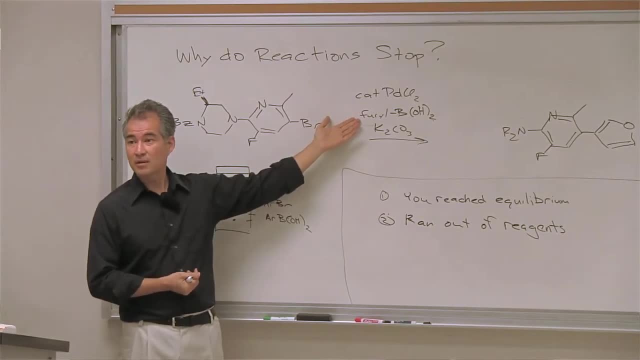 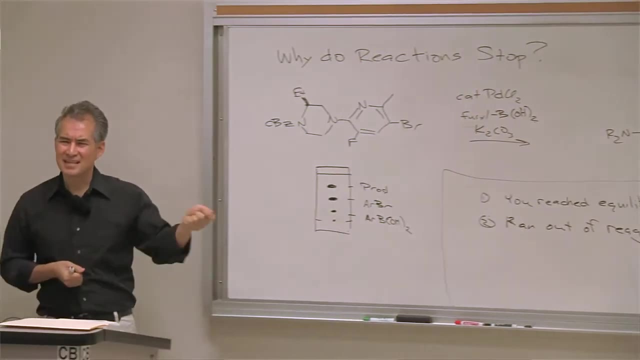 to form any more product. Well, there's two of them: The furoboronic acid, the boronic acid starting material, and the potassium carbonate. There's usually an excess of this. It's not easy to TLC that, so we can't tell- but usually there's enough of an excess that. 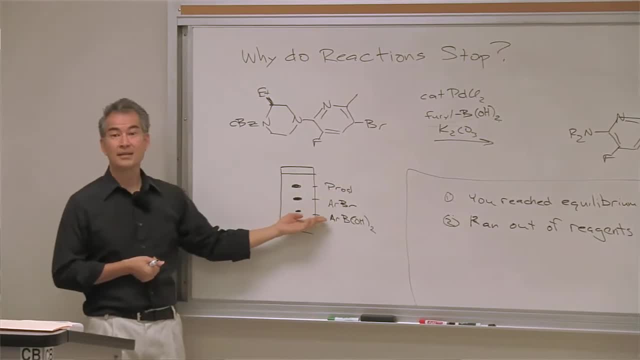 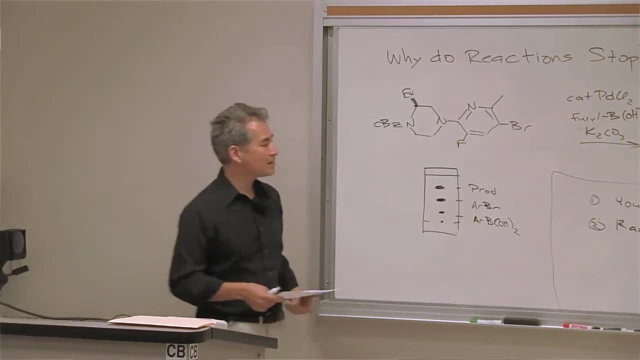 you don't run out of that component. But here I look at my TLC plate: It's still there. In this particular case, I know I didn't run out of my reagent because I can see that it's still there. And so now we're down to the last possibility for why your reaction stopped. 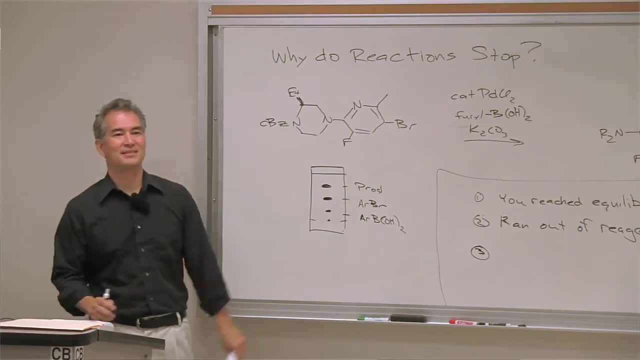 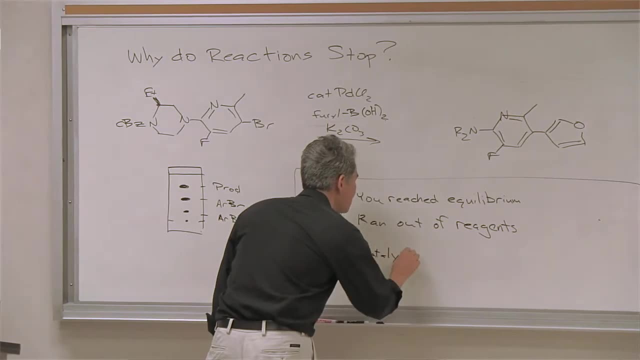 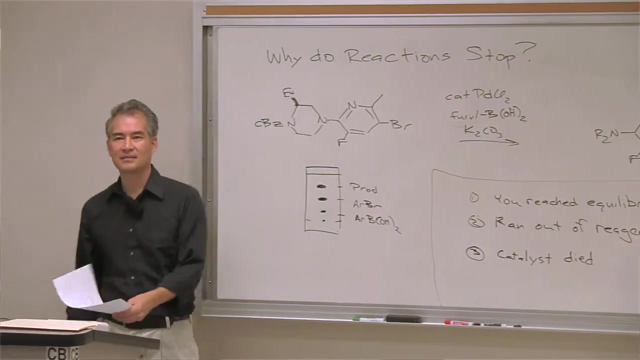 And there's not other secret possibilities here. Right, These are the possibilities. The last possibility is that the catalyst died, Right? So let's just suppose you had run out of the boronic acid reagent. What could you do to fix that situation? You dump. 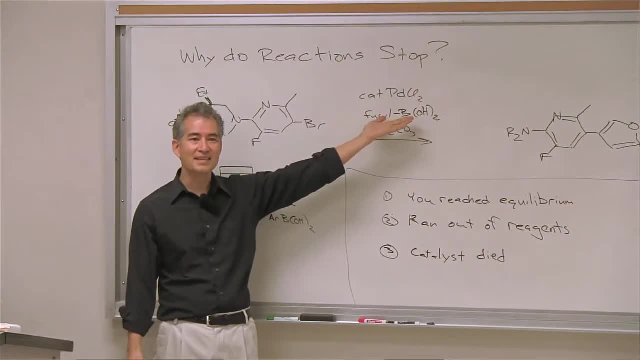 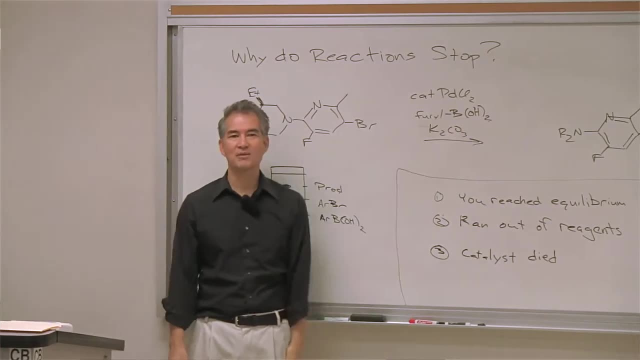 in more of the furoboronic acid That's commercially available. In this case, it took you 10 steps to make this. You don't want to dump in an excess of this. It's easy to dump in an excess of the reagent you ran out of. Just scoop in some more, Right. 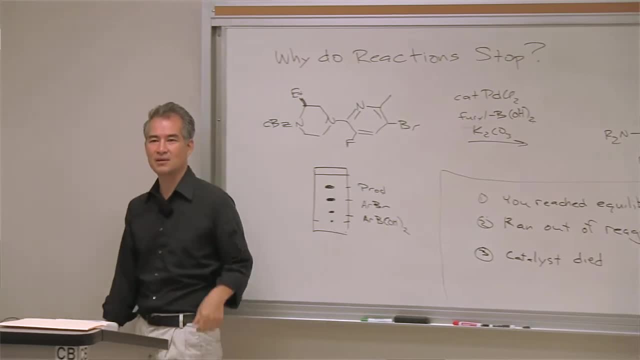 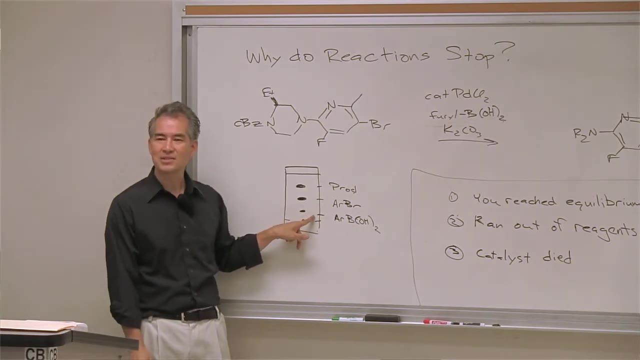 Rather than work your reaction up and take a 50% yield, just scoop in more of the reagent you ran out of And you can push your reaction to completion. But let's suppose there's still boronic acid there. We know that's not the problem, based on my TLC plate, If you see. 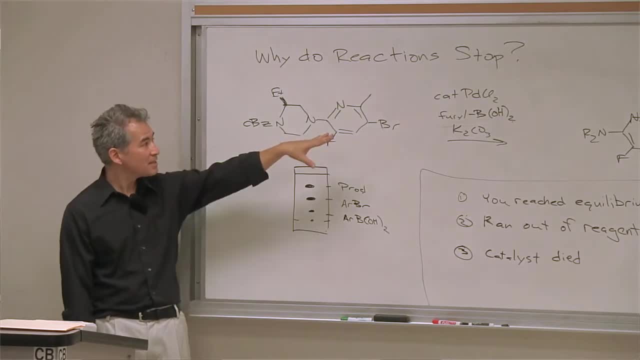 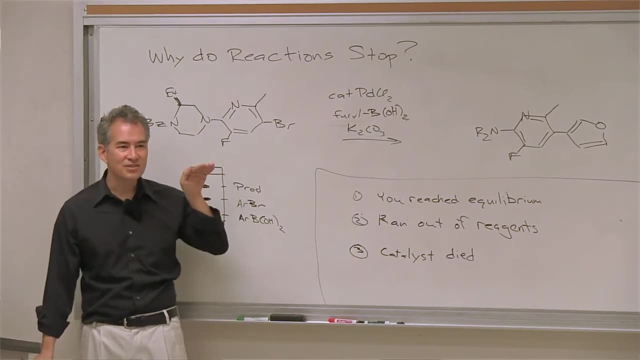 all of your starting materials on the TLC plate. in this particular case, that's because your catalyst died. It's not because the reaction just decided to stop. Reactions keep going until they reach equilibrium, And the equilibrium concept of this is going to lie way over on. 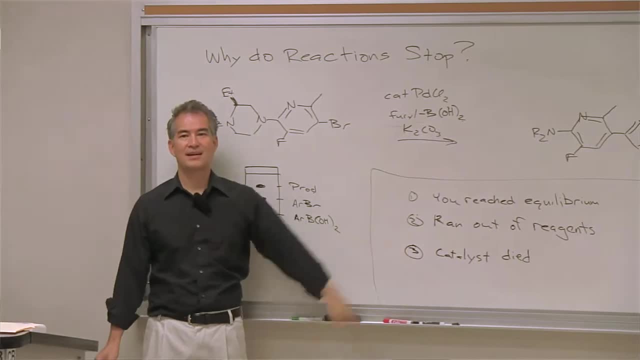 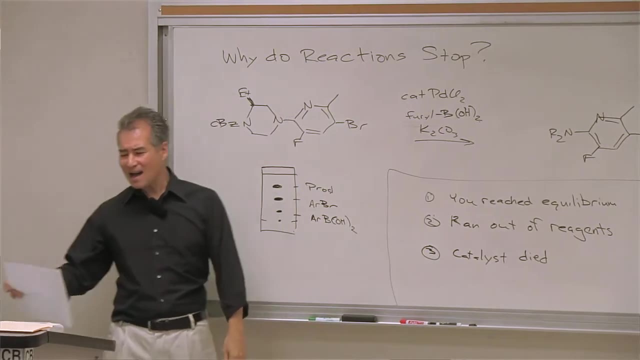 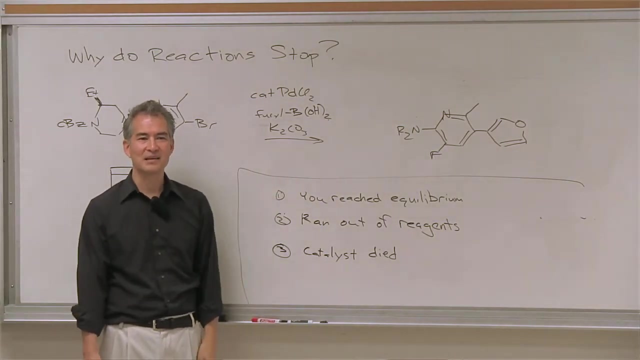 that side. So how do you fix the problem of the catalyst dying? Add more catalyst. It's possible your catalyst could be so expensive that you couldn't possibly afford to put in another equivalent or 5 mole percent of your catalyst. But generally who cares what the procedure said in the literature?